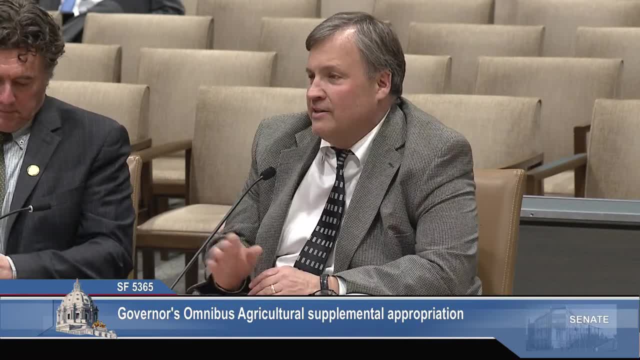 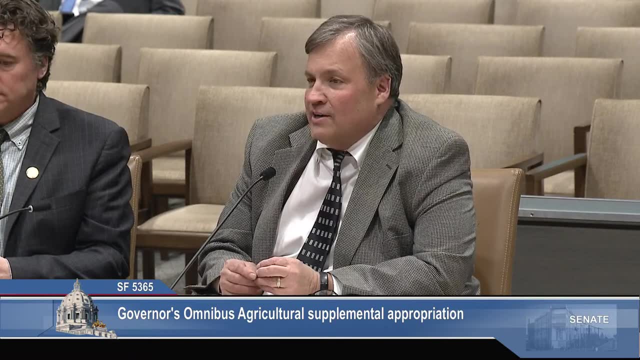 But all good stuff that will relate to the amendment and the DE you'll see later in working with the Senate and appreciate that. So with that I'll have. Ms Medina is going to walk through. You can just go to the next slide. She's going to walk through the slides. 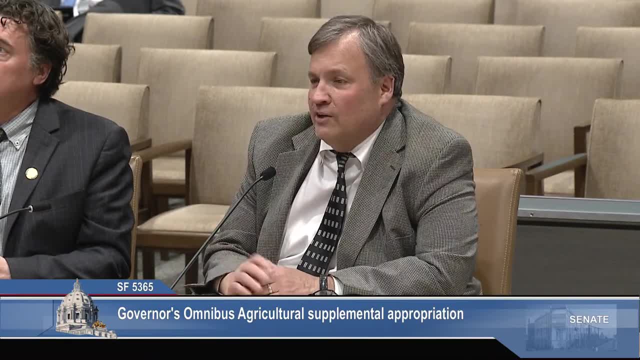 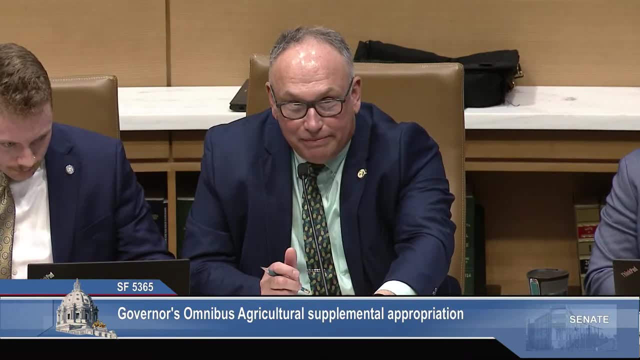 It's our mission. You can keep going And we'll just go right through it. I'll just turn it over to her and she can walk through the slides And we're glad to take any questions. Great, And you can just state your name and you know what to do. 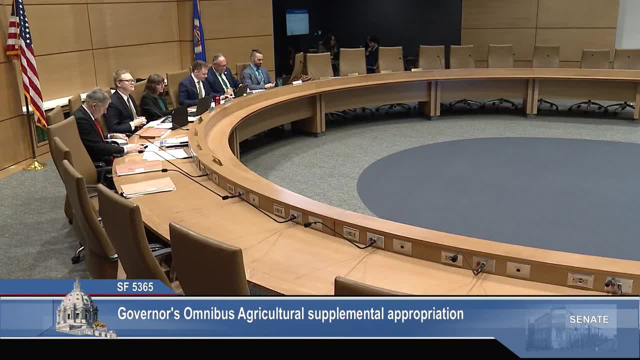 Perfect. Thank you, Mr Chair. For the record, my name is Michelle Medina and I serve as the governor. I'm the director of government relations for the Minnesota Department of Agriculture And I'll walk through the different budget appropriations. So the first one we have is: 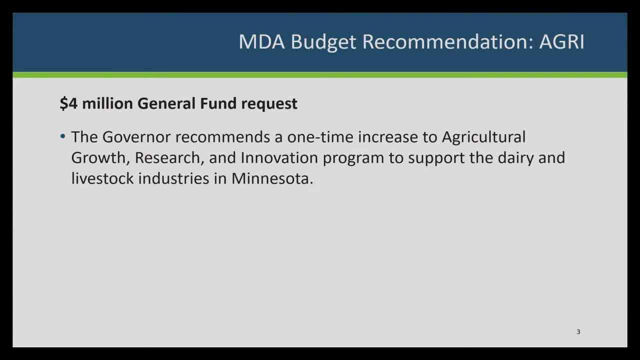 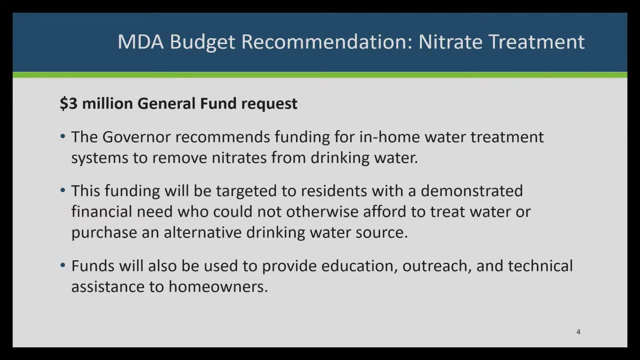 $4 million general fund request for agri. So this helps support the dairy and lassock industries in the state of Minnesota. This is in fiscal year 2025.. Also $3 million from general fund for nitrate treatment. So the governor recommends funding some in-home water. 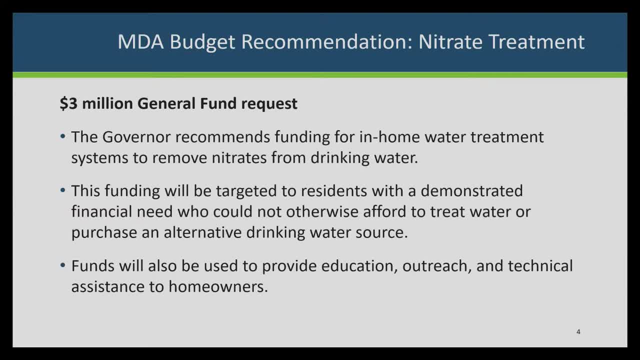 treatment systems to remove nitrates from drinking water. This will be targeted towards those homes that have the most need, So the, and also the residents that are in-home water treatment systems to remove nitrates from drinking water. So this will reduce the risk of overstating написhing during that period. The other one that we 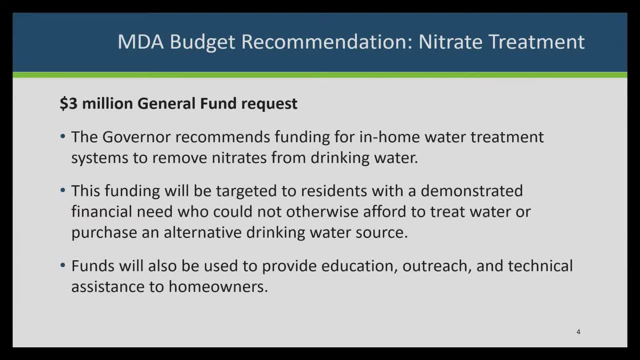 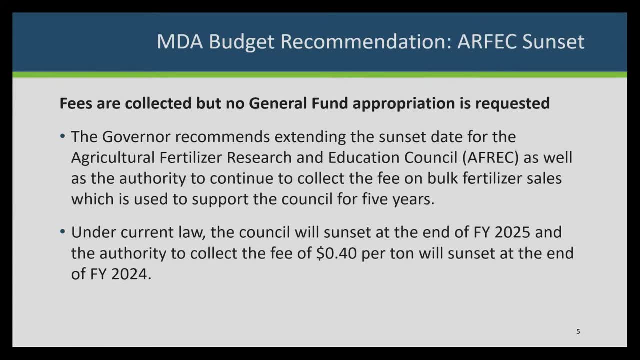 will be focusing on subscribers and healthily mothers at most risk-so pregnant people and children. So we'll focus on those areas And then we can also do use the funds for education, outreach and technical assistance, And this is just one time in 2025.. 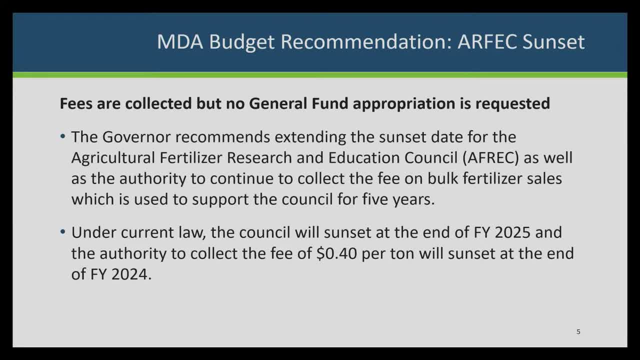 And then we have an Afrec sunset. So fees are collected for this, but there is no general funding wheels that are teacher's board, ak Можно Building For and consequent hydraulic educationpews and cater이다. So this extends the Afrec, the agricultural. 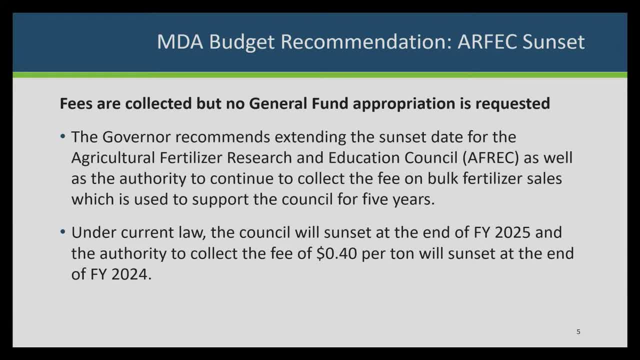 fertilizer research and education council For five more years. So it gives us an authority to collect the fees for on bulk favorites and thank you for giving us permission to provide the very dropouts for all of ourども cambium plans for on bulk for larger sales for five years and then also use those fees for 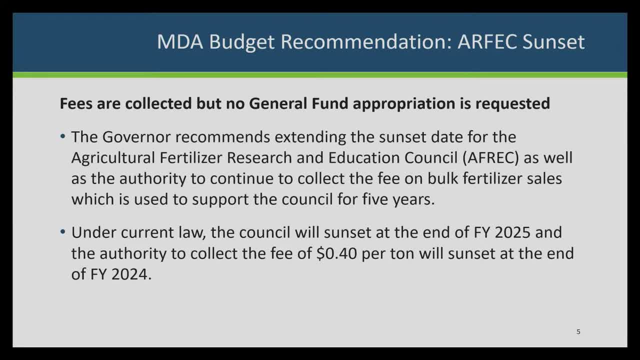 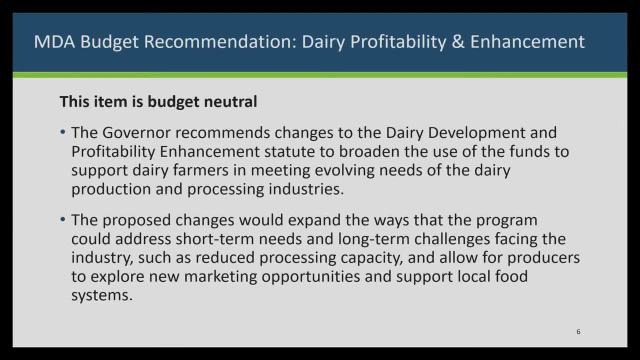 five years as well. so as a reminder, this fee collects 40 cents per ton and would sense that at the end of fiscal year 2024. another budget-neutral item is the dairy profit enhancement. so this one is changes to the dairy development and profitability enhancement statute to broaden the use of the funds to support. 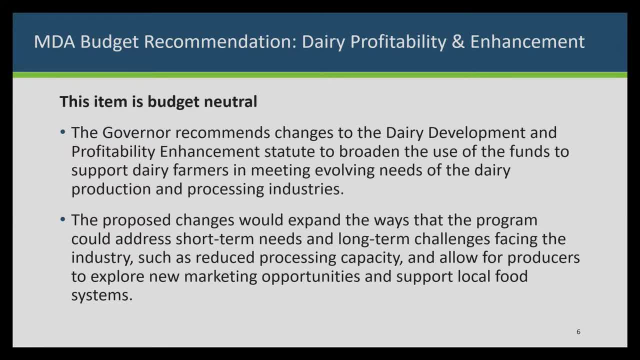 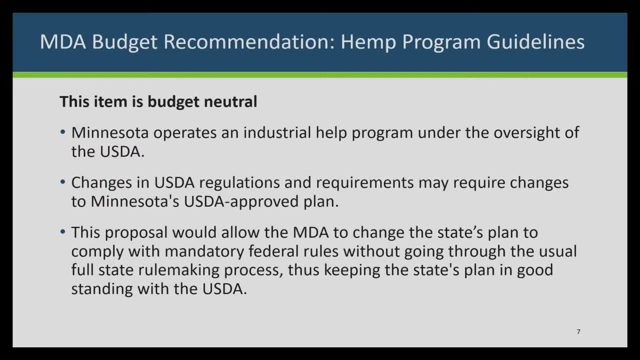 dairy farmers to kind of keep up with the evolving needs of the dairy industry. so this would just expand how we can use the funds. but again budget-neutral: the hemp program guidelines. another budget-neutral proposal. so we have a Minnesota hemp program is through the USDA and we need to keep up with their. 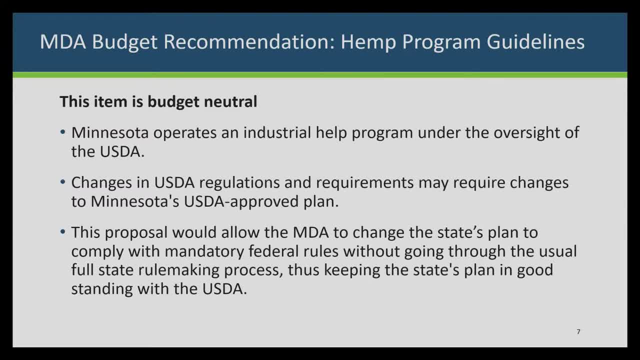 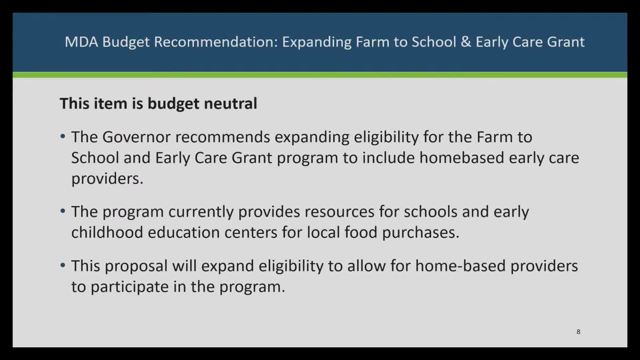 different requirements and changes to the program. so every time they make a change we have to update our state plan. this allows us to do that more seamlessly by not having to do rulemaking every time, but to update it through statute. then we had the expanding farm to school and early care. 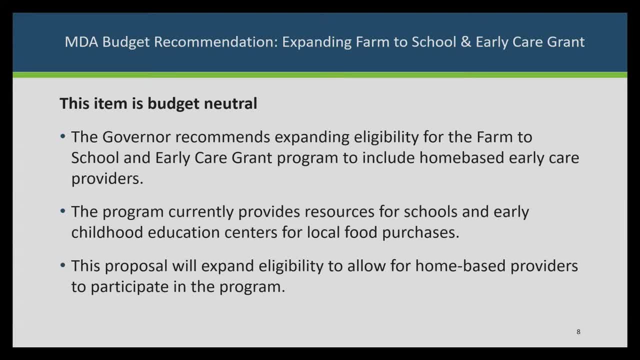 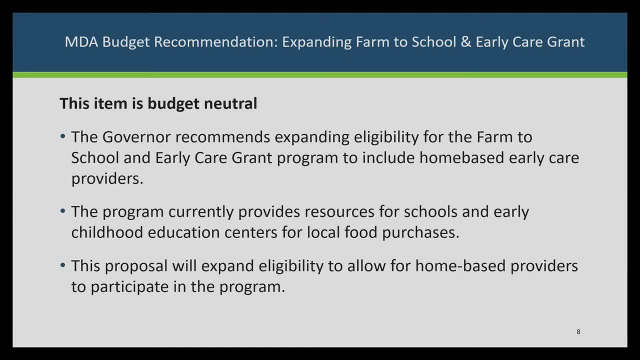 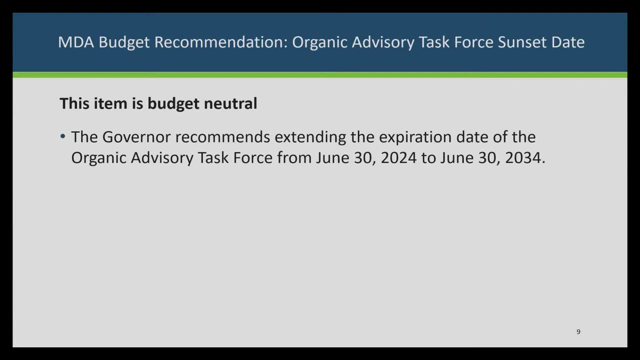 So this would allow them to apply for these grant programs as well. It's currently only provides resources for schools and education centers for local food purchases And then again just expands it to home-based providers. The organic advisory task force- sunset date. this would extend the advisory task force for another 10 years. 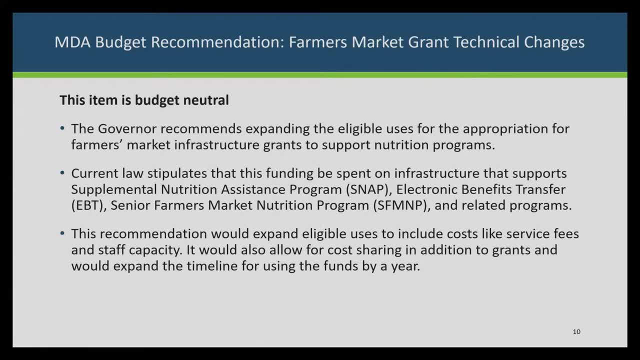 So it extended out to 2034 For the farmers market grant technical changes. This is would expand the eligibility uses for the appropriation that was from last year's session For the farmers markets infrastructure grants to support nutrition programs. So this would let them to expand those uses to cover costs like service fees and staff capacity. 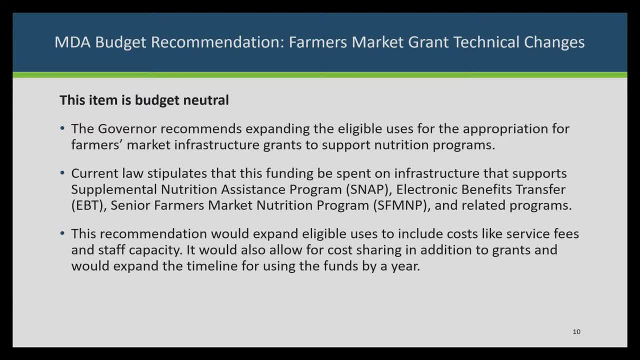 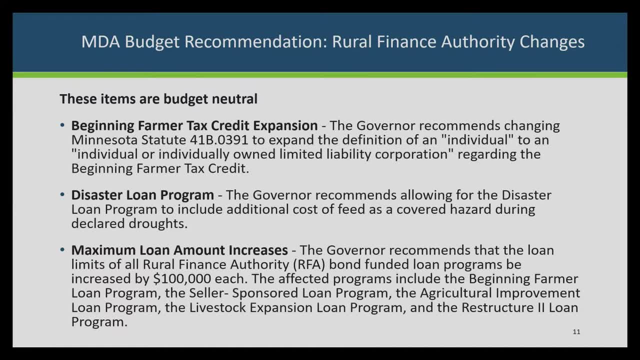 And we were quite a bit with the farmers market Association and these were all changes that they were very supportive of. Then we have some real finance authority changes. These are all budget neutral. So the first one is, for the beginning, farmer tax credit expansion. So this would expand the definition of an individual to an individually individual or individually owned limited liability corporation. 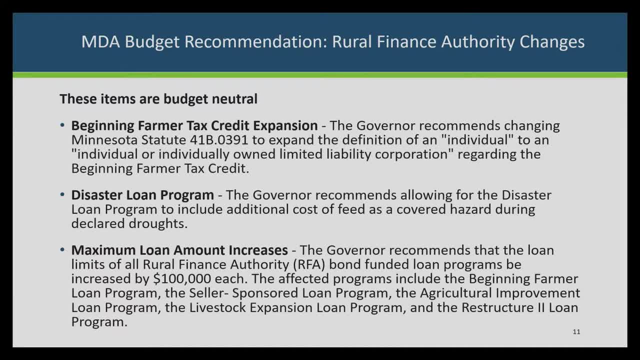 We know that a lot of beginning farmers create LLC's and they apply for this program with an LLC Which currently is not eligible for this program. It has to be an individual applying. so this would allow those LLC's owned by an individual to apply and Receive that tax credit for the disaster loan program. 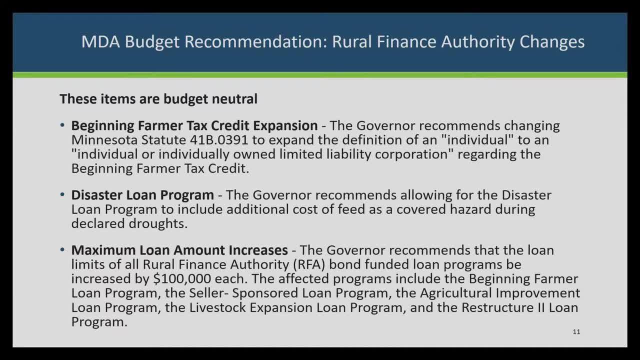 This would allow the additional cost of feed to be covered as a hazard during declared droughts and Then for the maximum loan amount increases. so the governor recommends that we increase All of RFAs bond funded loan programs by $100,000 each. So this would include the beginning farmer loan program, the seller sponsored loan program. 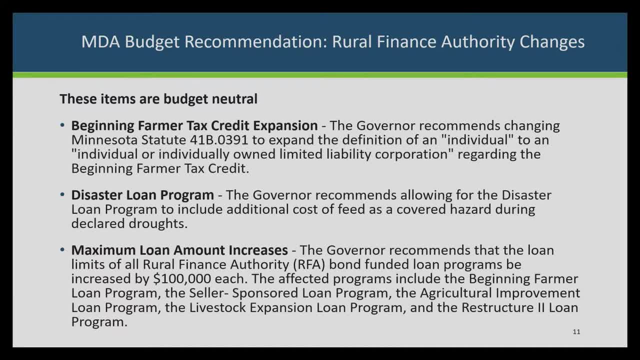 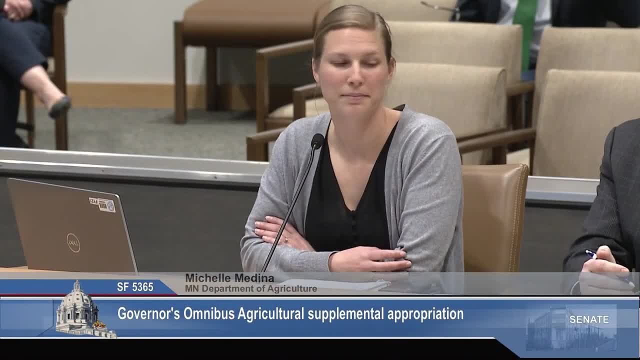 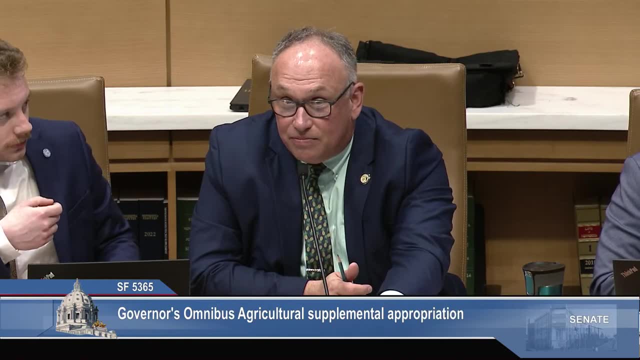 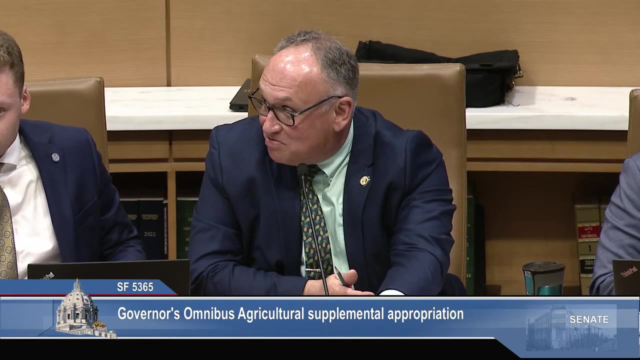 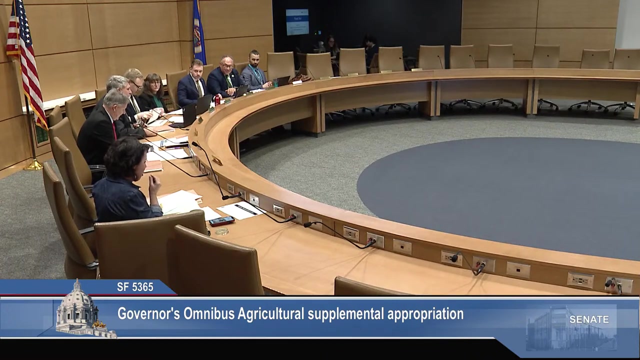 That your cultural improvement loan program, the last log expansion loan program and the restructure to loan program, and That is all the changes. Okay, thank you. anything else? Questions for the commissioner. presentation senator Dornan. Thank you, mr Chair, And I just had a question on the three million general fund request. if there's a little more details to that. 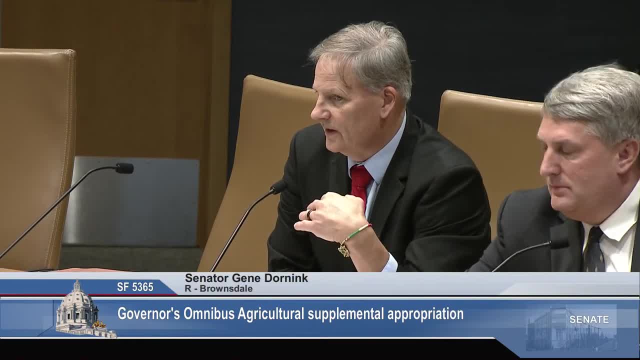 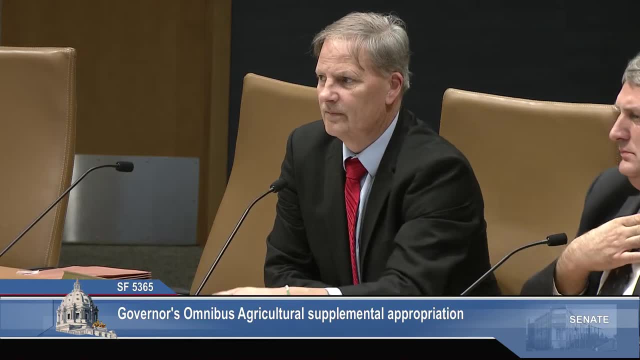 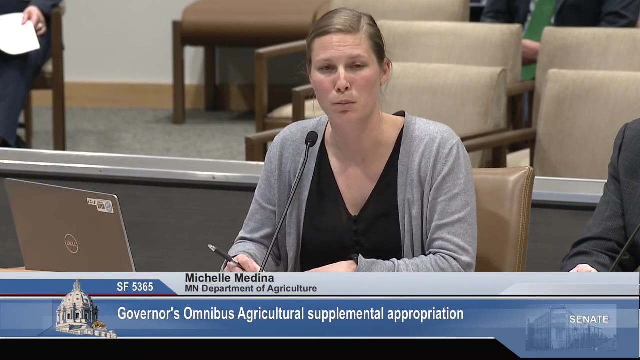 as far as how they're gonna administer that with the Costs for per residents. So they have a any of those details worked out or not, yet, Spadina or commissioner, don't take it. Yeah, mr Chair, senator. So we're expecting them to cost about two thousand six hundred dollars per RO system per household. 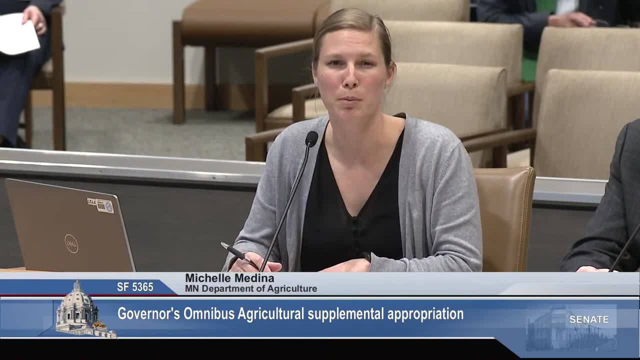 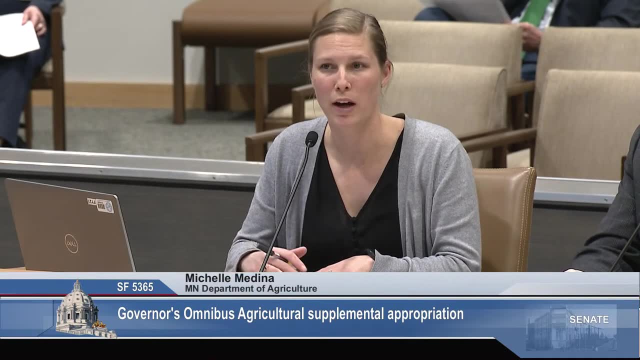 So with that three million dollars to be available for over three years, We assume about 1 million per year. at that rate We figure that we could do about 150 of wells at 100 percent cost year. So we'd pay all the 2600, we could do 350 wells and a 50 percent cost share. 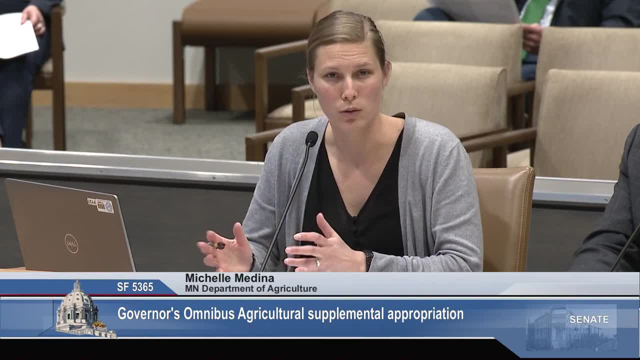 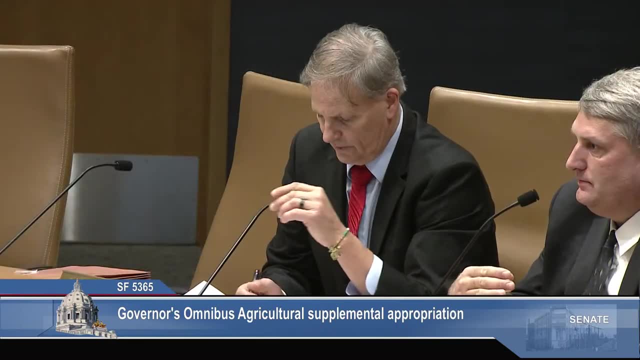 So a total then of 500 wells we could do per year with that funding if we had three, if we had 1 million per year. Senator, I think we're sure the follow-up just talks about demonstrate financial need. Do you have a cutoff on where we're gonna? 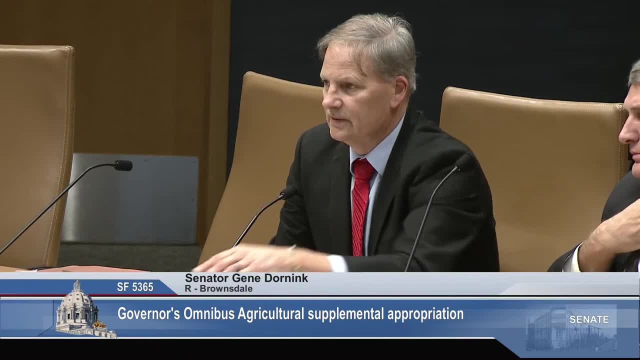 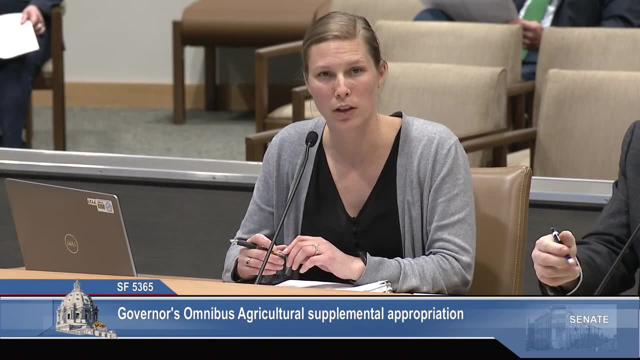 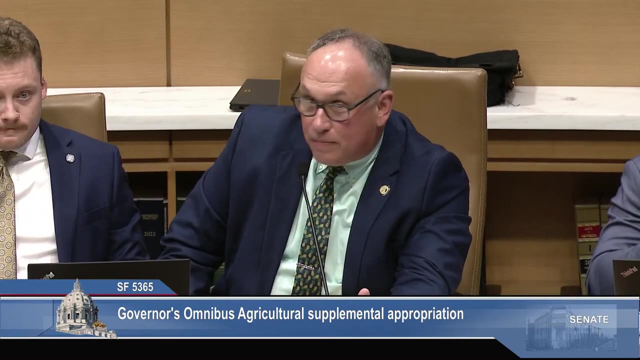 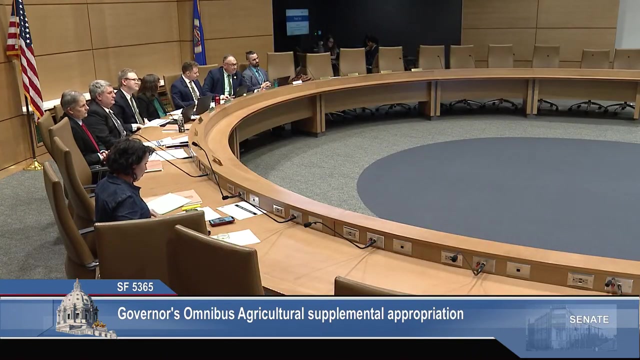 Yeah, what's the threshold there? Dean, mr Chair and senator. so we're looking at Minnesotans that are at or below 200 percent of poverty. Any other questions? Okay, seeing no more senator putt, Thank you. Thank you, mr Chair. 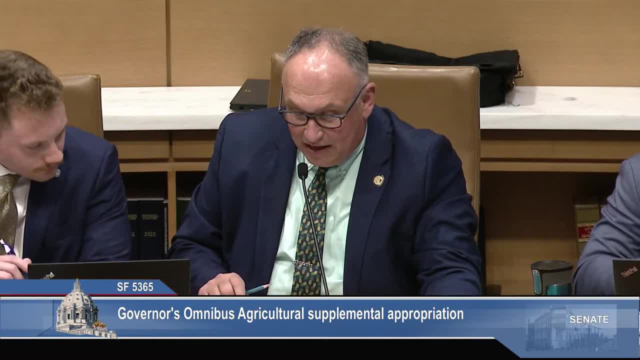 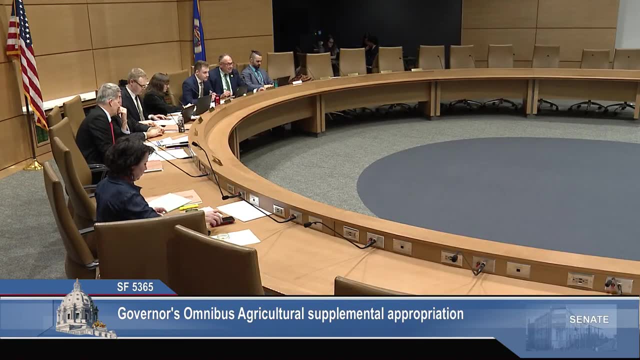 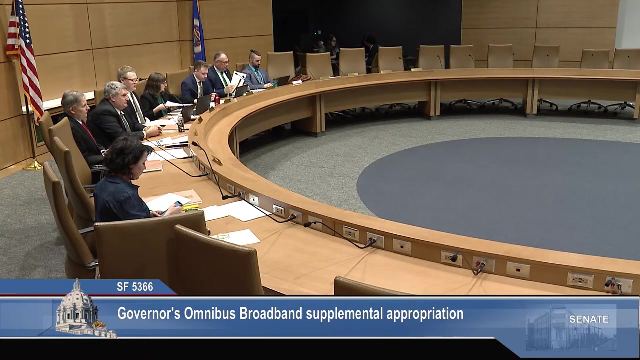 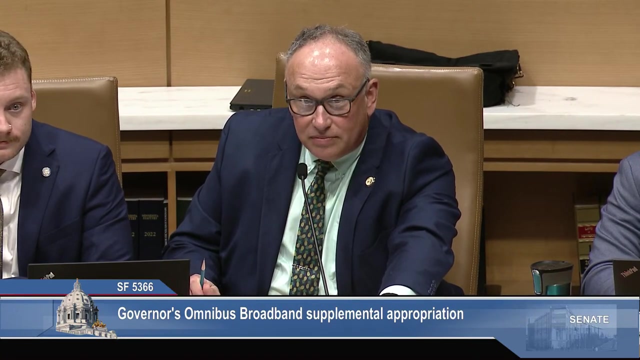 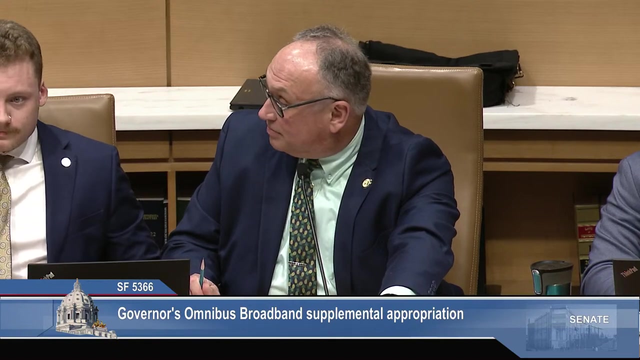 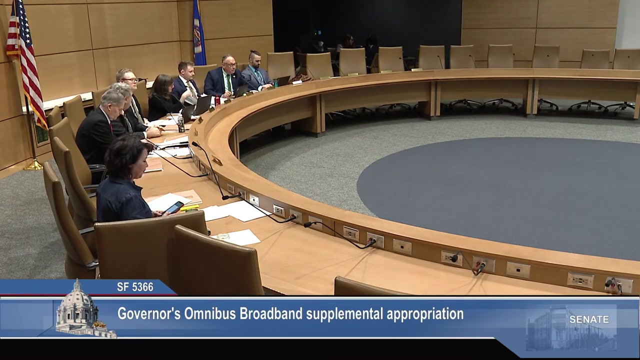 Okay, Thank you. with that, We will be laying Senate file 53 65 over, And now we are on to Senate file 53 66. Mr Townsend, Please, Thank you. While they are getting set up, Senator Putnam, do you have any opening comments? 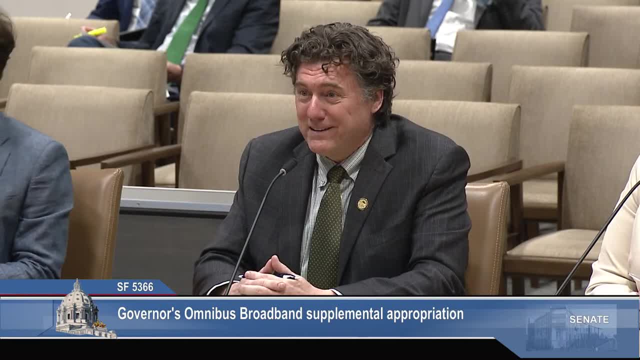 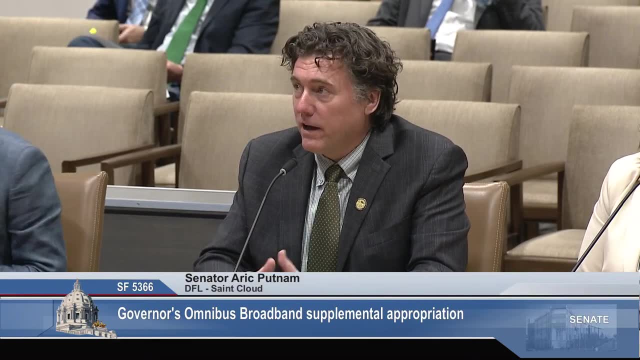 MR. Thank you, Mr Chair, Excellent timing. Yes, what we're about to hear is the governor's supplemental broadband budget proposal, and I'm grateful to have our friends from the Office of Broadband here to tell us all about it. 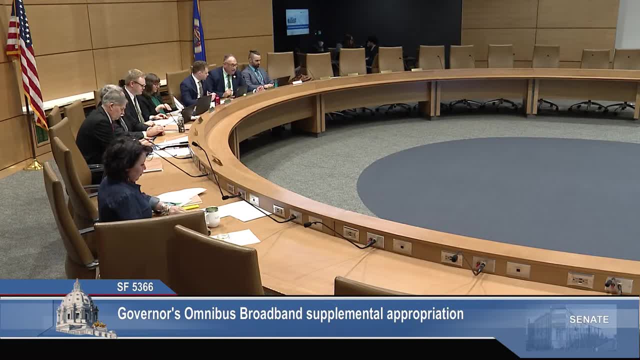 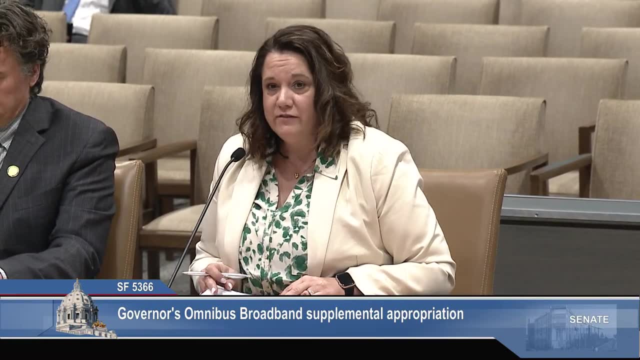 MR. Okay, You may state your name and begin your testimony, MS. Well, good afternoon Senators, and thank you, Chair. My name is Bree Mackey, for the record, and I'm the Executive Director of the Office of 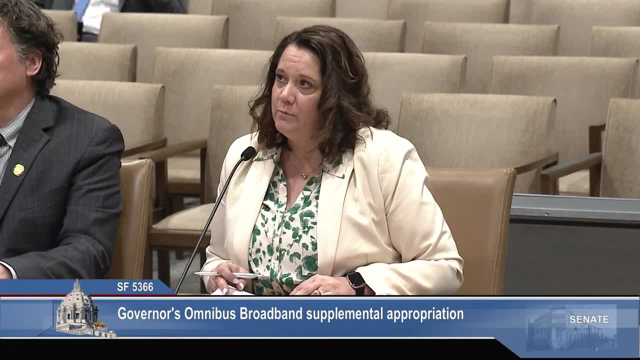 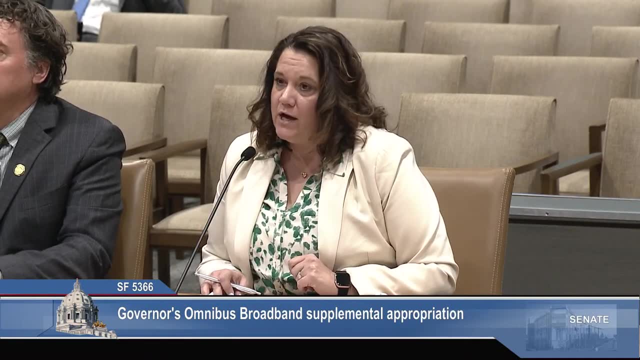 Broadband Development, And today we are going to present the 2024 Broadband Supplemental Budget Proposals. So there are two items we'd like to discuss with you today, and one is the transfer authority and the other is authorization to utilize the budget. 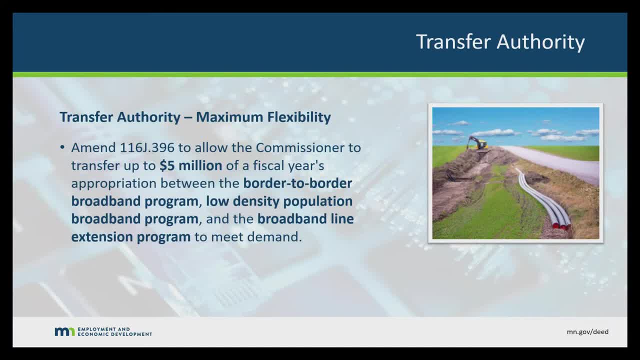 The first item is the federal digital equity funding. Both of these are budget neutral, so I just want to point those out to you. So the transfer authority really is asking and allowing the commissioner to transfer up to $5 million of the fiscal year's appropriations between the border-to-border grant program. 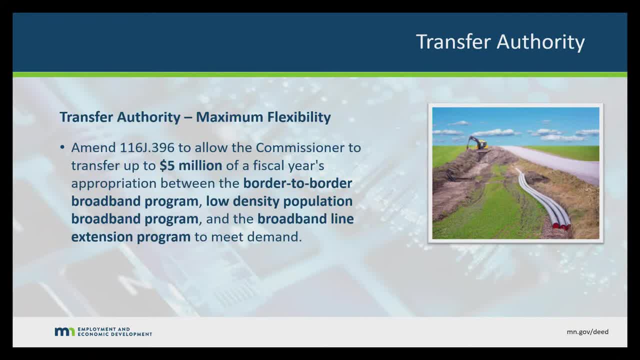 the low-population density broadband program and the line extension program to meet the demands, And I'll share a little bit more about each of those in a little bit MS, Thank you. The next slide, just as a reminder, and I know you have seen this earlier in this session. 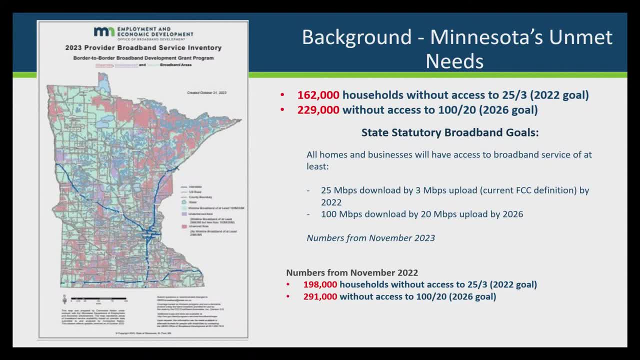 but what is the need? that is still out there, And so, based on our maps from last fall, we are still showing that 162 homes are without the access of 25-3, and 229,000 homes do not have the speed goals of 2026 at 100 by 20.. 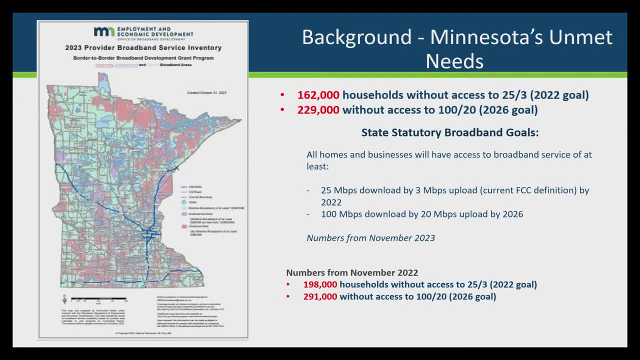 I do like to point out on this slide. if you look back a year ago- November of 2022, you'd see that the programs that you all authorize are making a difference, but the need continues to be there. I also can we go back one second? sorry, just two things also to point out, and again: 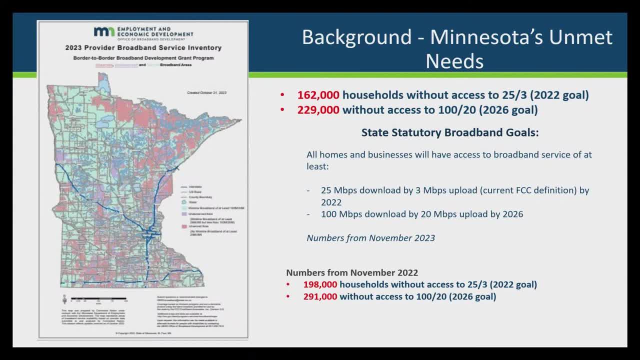 as the Committee of Jurisdiction, you are very well aware that these locations are the most expensive and the hardest to serve, And so flexibility to move where the need is and the best grant applications that come in to meet those needs with match fund is what we're looking for in those transfer authorities. 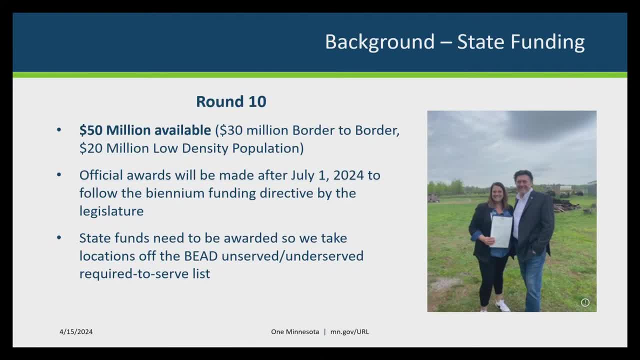 MS. Thank you. Just again, as a reminder, we are in grant round 10 of the biennium appropriation that you all made available last year, with 50 million available in our border-to-border grant program and 20 in the low population density program. 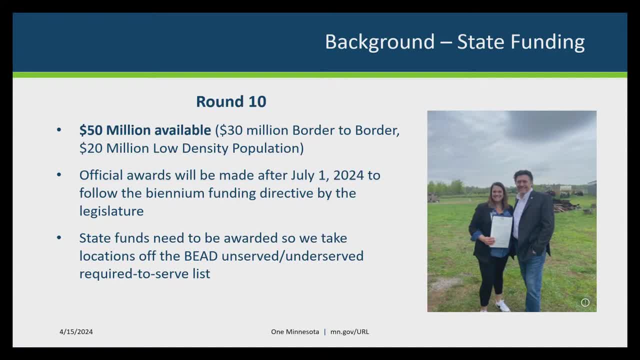 Official awards are hopefully to be made July 1 to line up with the next biennium and state funds need to be awarded so that we can take locations off our BEAD. final map of unserved and underserved locations As a reminder. just for historical information: grant round 9 last year when we made our 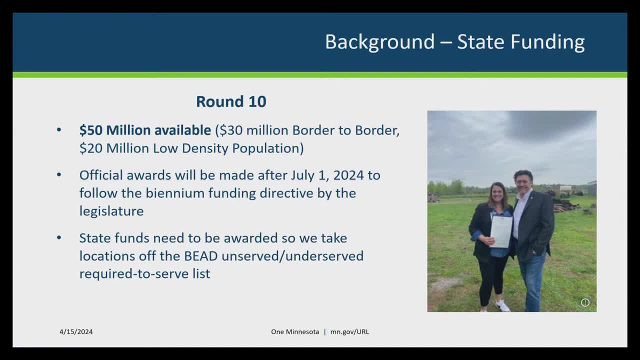 award, or actually a few. about a month ago, I guess, we had over 69 applications In the border-to-border. we had 38 applications for over $65.5 million in requests and 31 applications in the low population for 85.8 in requests. 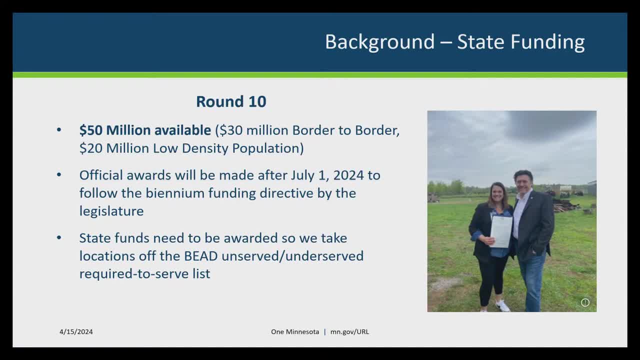 MS. That includes land use and that's a $65.5 million pool. We know that the need and the requests are still out there. I also just want to point out that with those awards came 49 percent match, so 51 million. 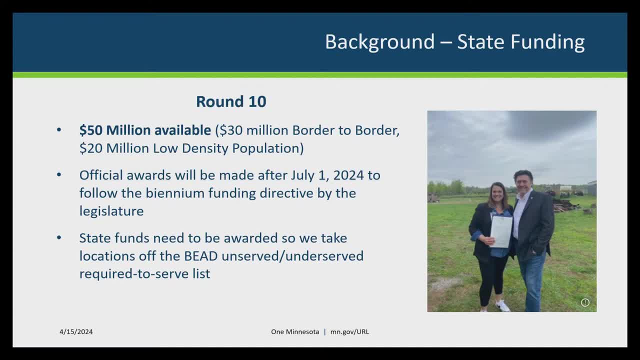 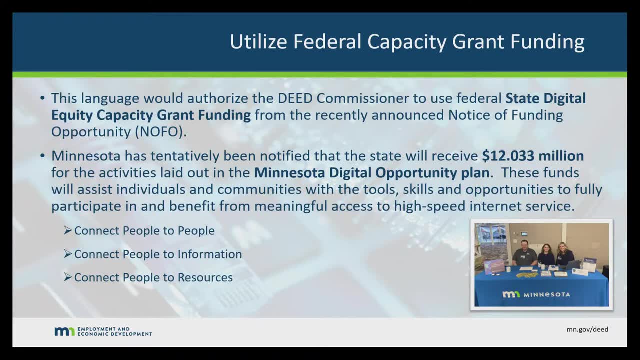 in local match was also leveraged by awarding these grants. All right, so utilizing the federal capacity grant dollars. so, as you recall, the language would or we're in the middle. We just got approval of our digital opportunity plan by NTIA on March 23,. in order to help, 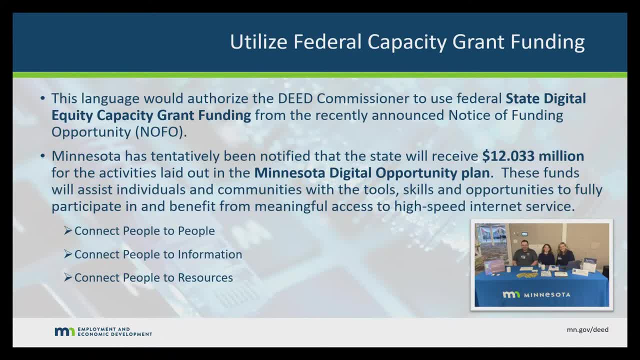 the state of Minnesota, and the state of Minnesota will be able to receive funding by the end of March 26.. What we' re asking here is for the dean commissioner to use the federal state digital capacity grant funding from the recent announcement of notice of funding opportunity from ntia. 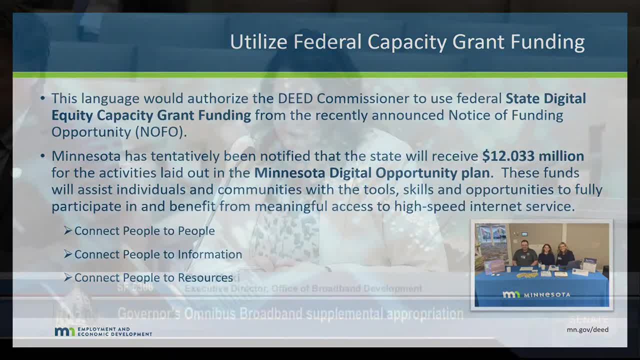 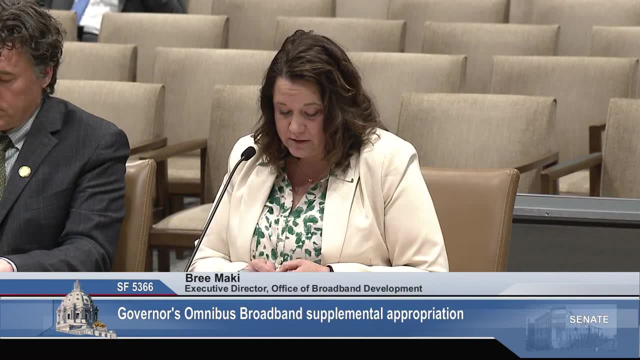 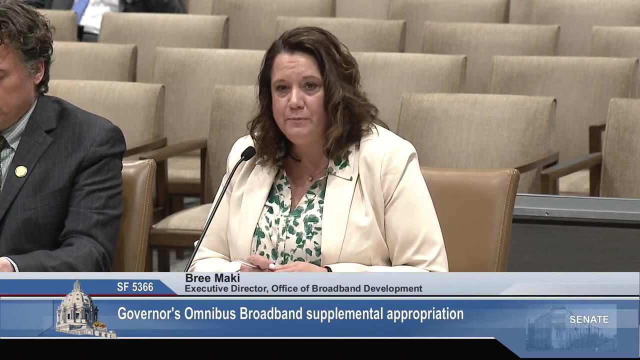 Minnesota has been notified that will tentatively receive $12 million for activities laid out in our digital opportunity plan. these funds will assist people with high speed internet. we learned in our digital opportunity plan that what matters most to Minnesota is connecting people to people, people to information and 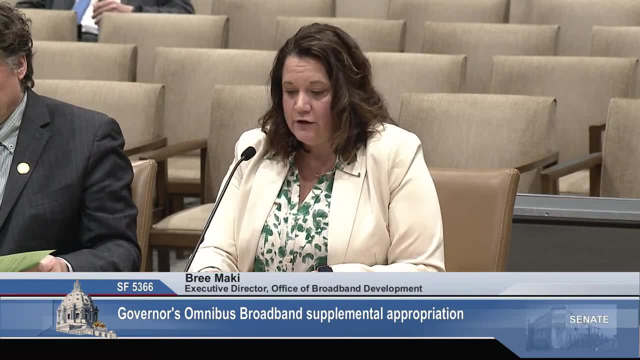 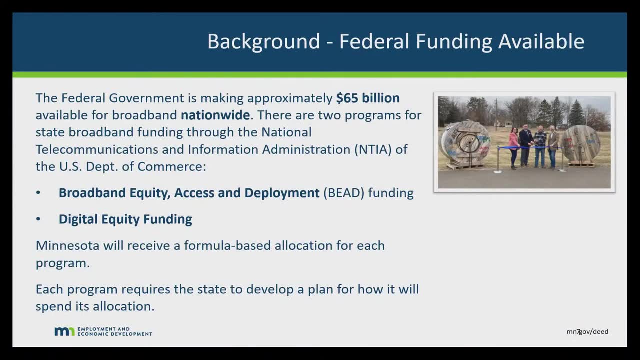 people to resources. As a reminder, the federal funding made available is through the ntia, so the national telecommunications information administration. through the infrastructure investment and jobs act. We talk a lot about a bead and again bead is the program that will be involved in the development of. 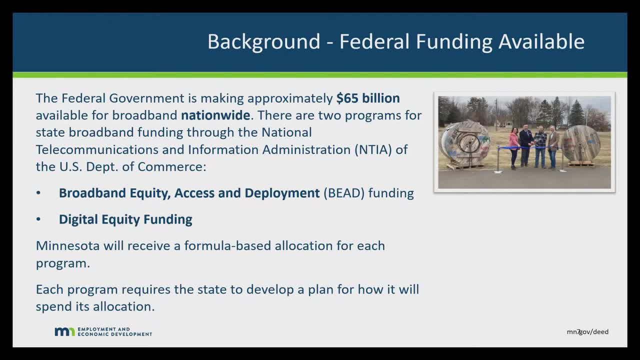 broadband across the state. The digital equity funding is what is in our digital opportunity plan and really again, those skills and needs of the folks to be able to participate in the high speed, affordable internet world. Each program required the state to develop plans, So with the 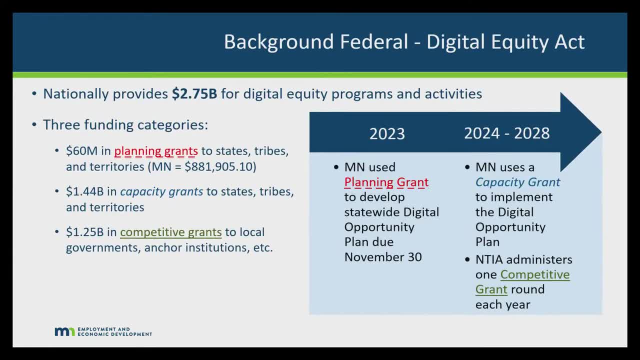 digital equity plan. thank you as a reminder- and I know you' ve seen this all before- but we did receive planning dollars to develop that plan And now we' re moving into the notice of funding to be able to apply for the capacity grants to be able to do some. 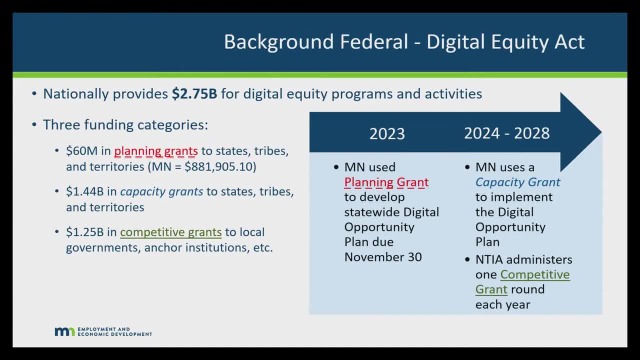 of those initiatives that we identified in the plan, And so that' s just a little timeline and the different areas. We can also look at applying for competitive grants when the notice of funding comes out for that as well. For Minnesota, when we went forward to create a digital 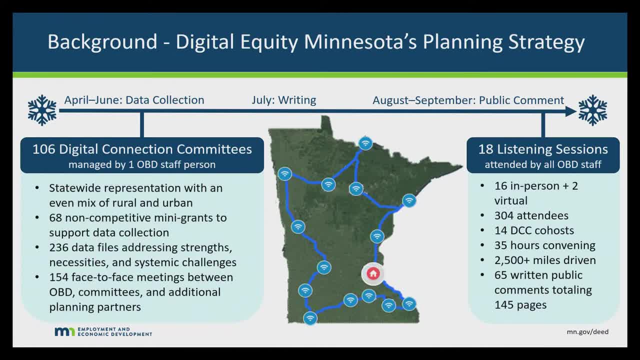 opportunity plan. we went across the state and had digital connection committees that were self directed and self acknowledged, and we had over 106 digital connection committees across the state. We took information from all of them based on what they have identified as needs, barriers, information. 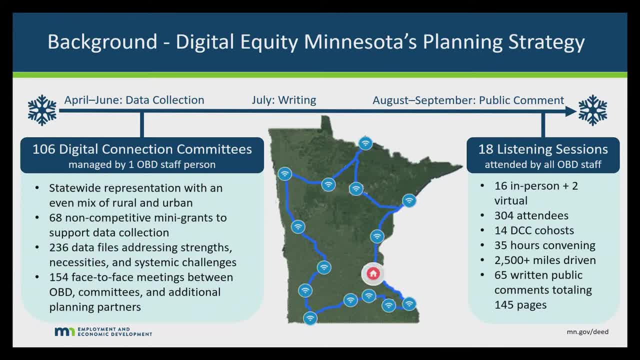 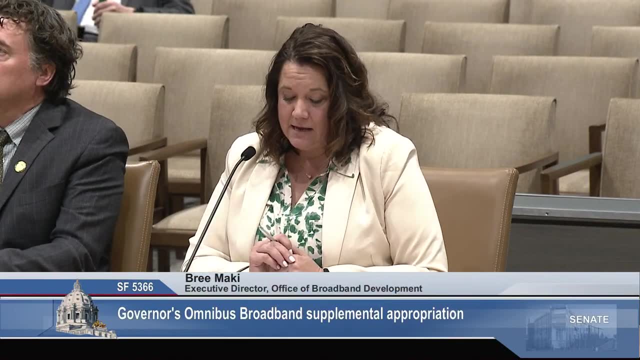 resources and then developed a plan. that was not something that was formed before we went on into communities, but was really formed after gathering all of that information. We also did listening sessions across the state to develop that plan, And here' s just a list of some of the 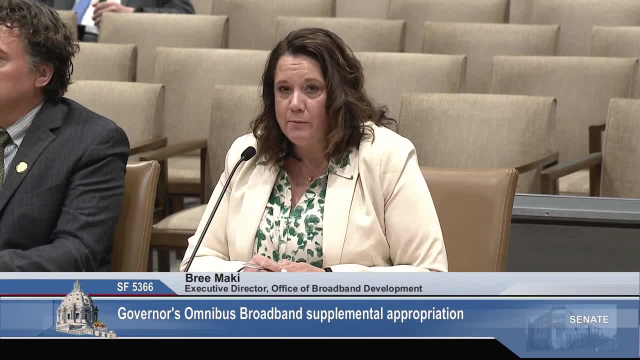 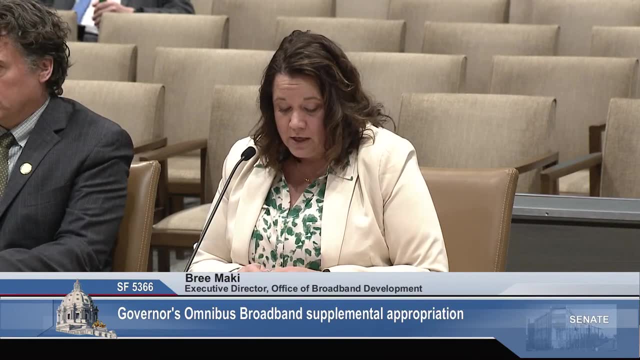 example, activities that came out of our plan. I do want to state that the approved digital opportunity plan is available on our website as well, as we do have paper copies for those that would like those as well. But some of the things we did identify is: 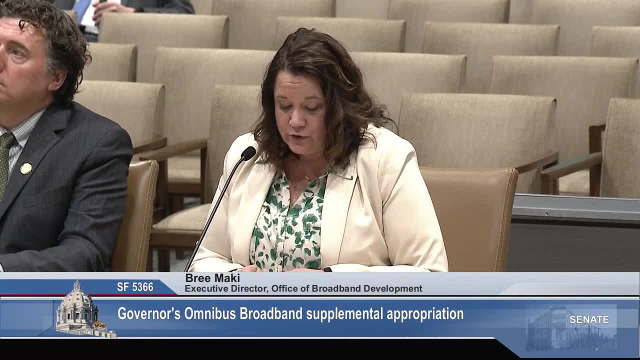 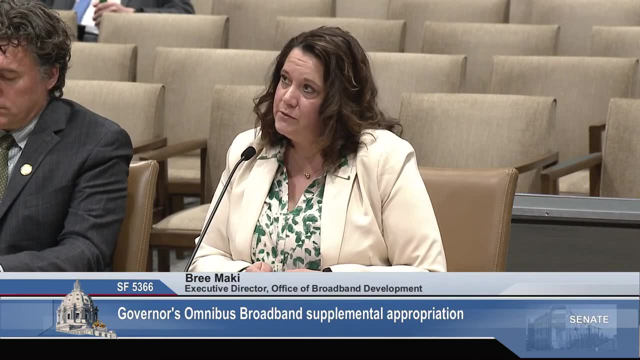 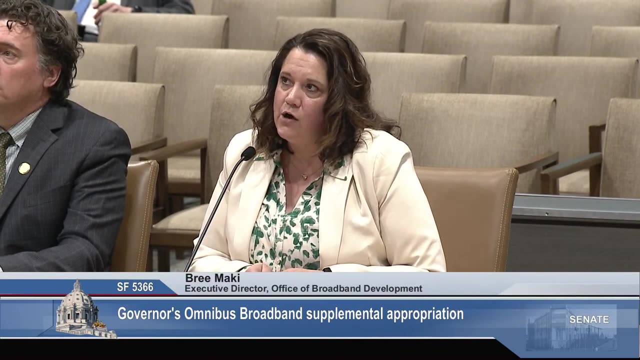 to develop curriculum and administer grants to high schools and two year colleges to support the training and hiring of students in paid technician internships or technical support, As well as creating programs possibly for our townships, cities, counties, in a formula base, So not to create an 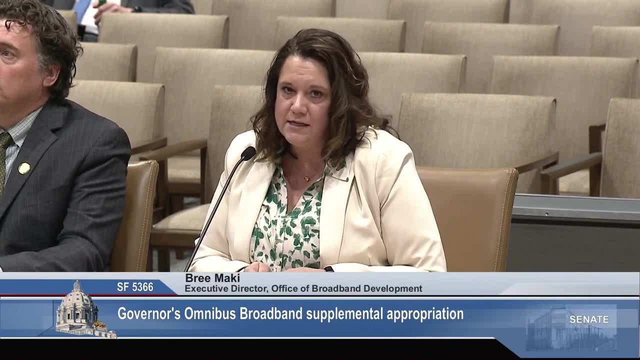 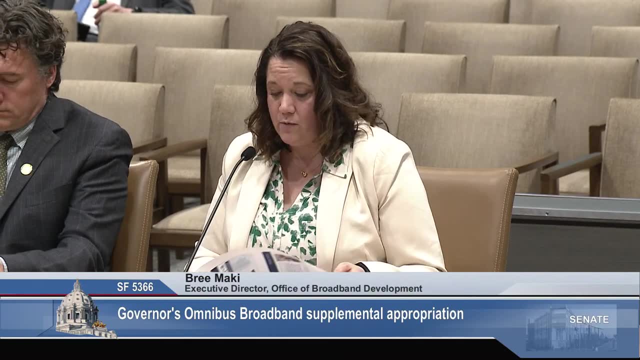 equity issue for counties and local governments that have the resource to apply for those grants, but really providing digital opportunity across the state in many ways. And finally, where are we now? So again, as I stated, our approved plan is available on our website. It was accepted by. 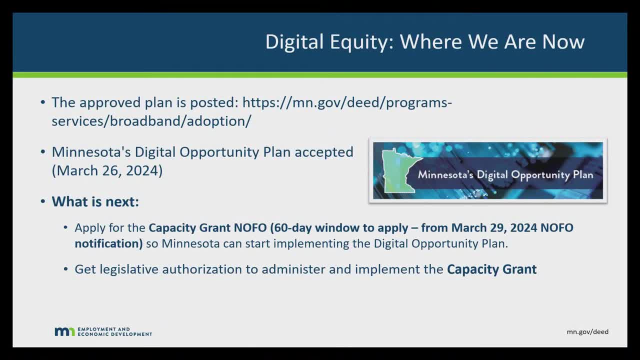 NTIA on March 26.. And next step is we have 60 days for the approval of the program And then we have the approval of the program from March 29 to put in our application for our capacity grant request of $12 million. 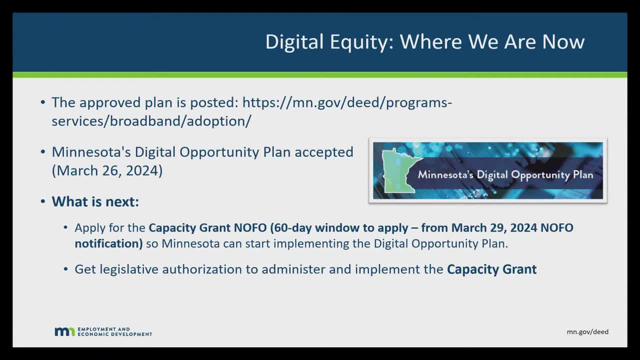 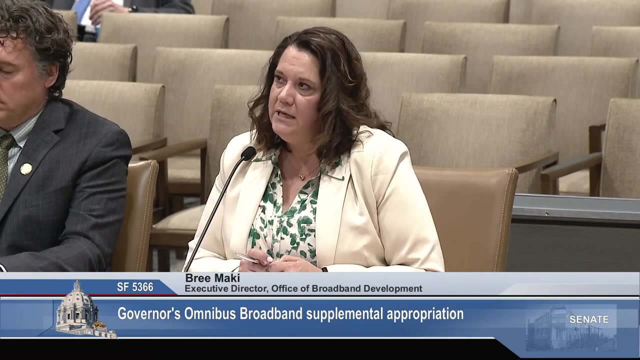 So we do have an opportunity when we submit our capacity grants to do a little bit of update, if we wish to. in our digital opportunity plan We know that we would like to add some language around careers and broadband infrastructure to help meet some of the needs we are seeing and 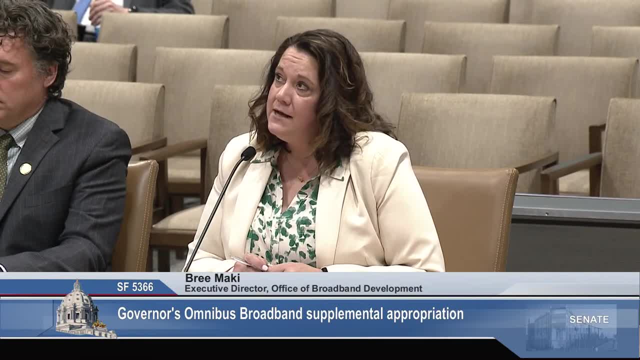 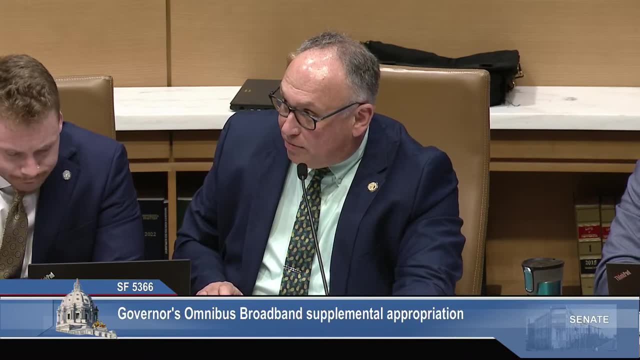 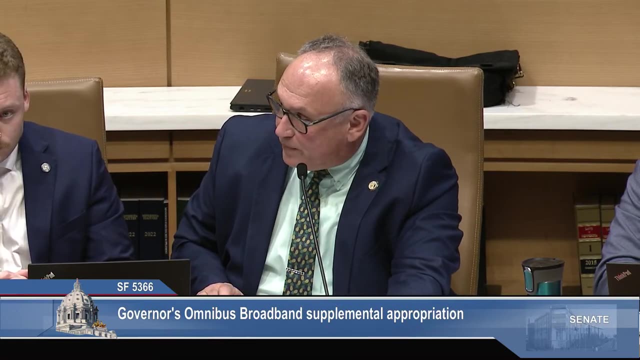 conversations we're having across the state. So with that, that is the presentation and happy to stand for questions. Thank you, Ms Mackey. Questions from members. Senator Westrom. Ms Mackey, how much money are you looking to transfer to the? 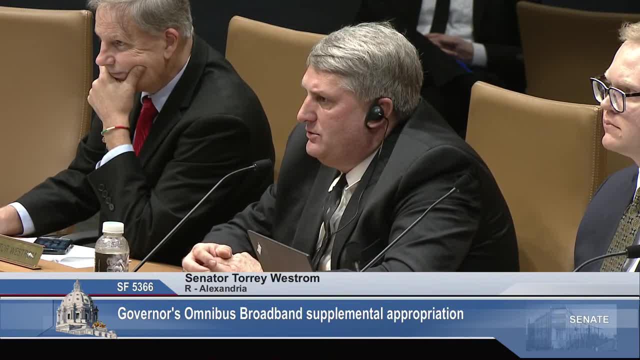 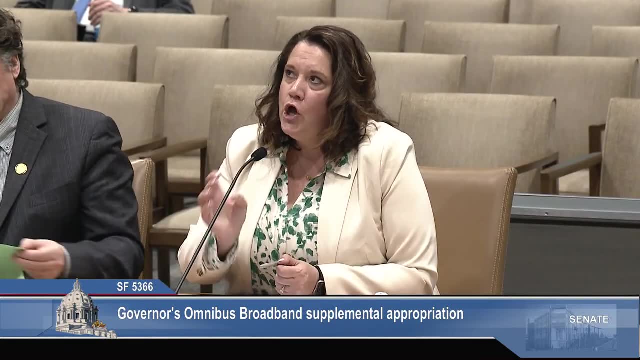 low density program or from that. can you revisit that a little more, Ms Mackey? Yes, thank you, Chair, and thank you, Senator, for the question. So, really, what that would allow us to do is up to $5 million in transfer, based on the applications. 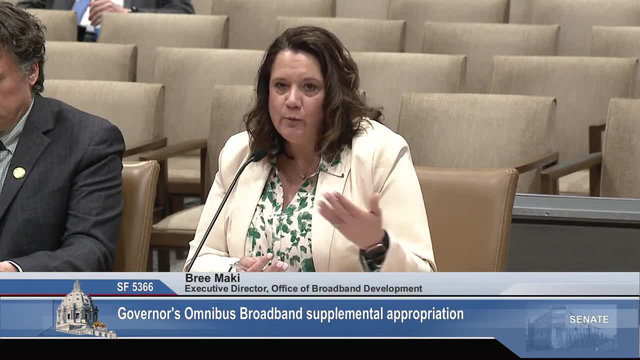 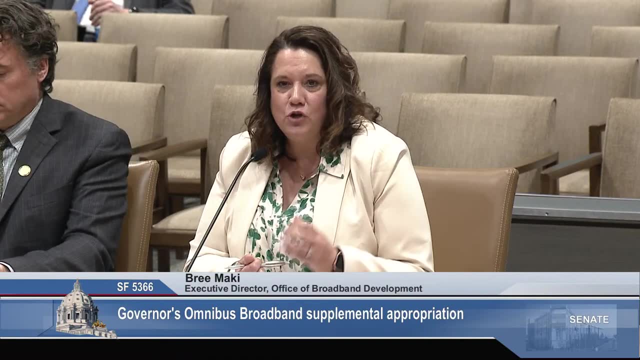 we would receive during this application time. So we know right now we only have that additional $50 million. we'll be making awards. What we saw last time is that we had some good applications because of the threshold of only $20 million. in the low population we were. 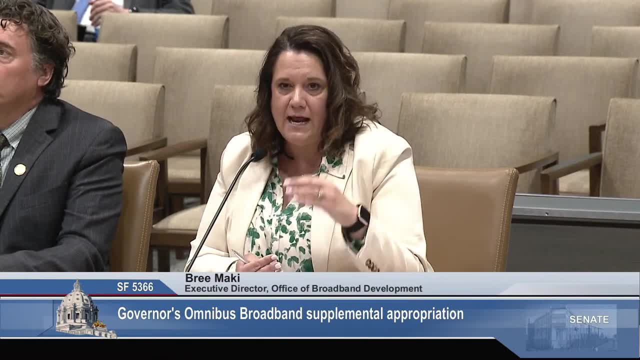 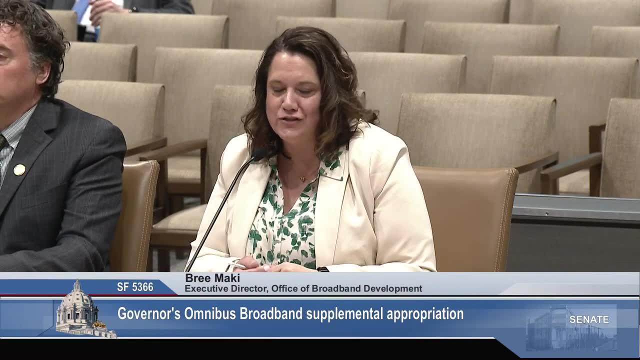 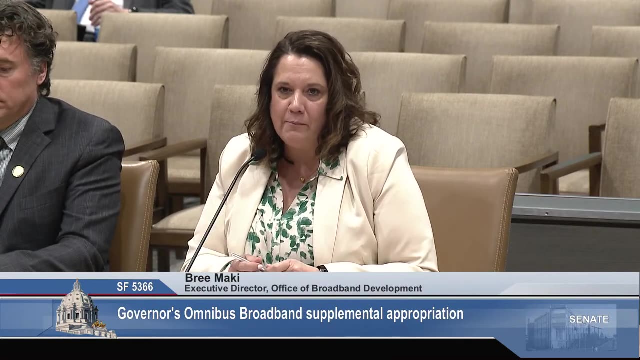 either unable to fund the next one and have to fund a little less because we couldn't go over the $20 million and we had some applications that were very close and an extra, say $300,000 or $1 million maybe would have been something that would have made for a good application. 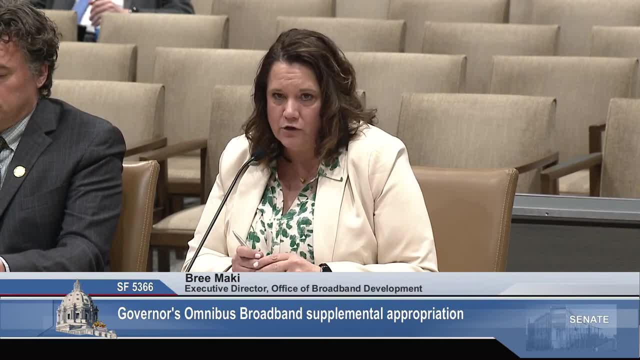 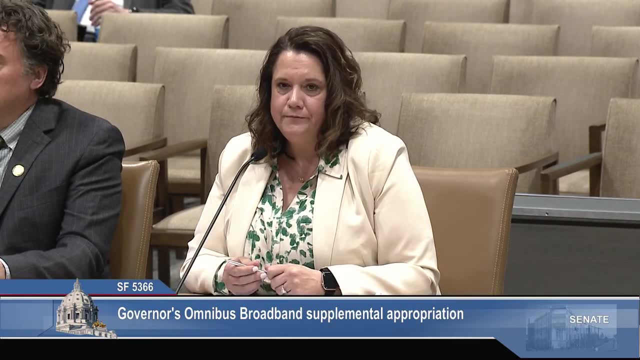 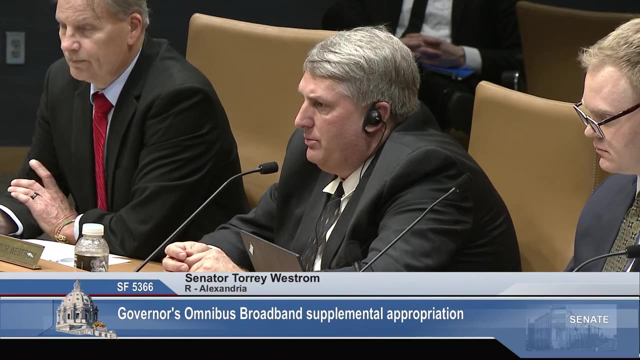 So just looking to transfer up to $5 million within that funding cycle. but it varies a little bit on the applications we receive: Senator Westrom, Mr Chair, so Ms Mackey. so it's just flexibility of up to $5 million out of the regular rural. 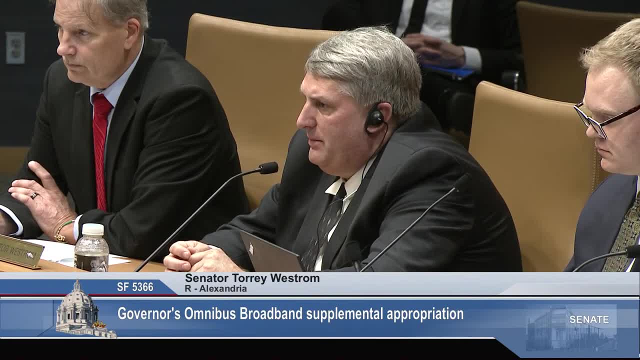 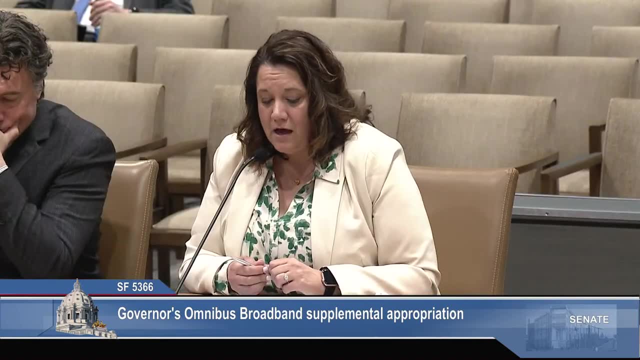 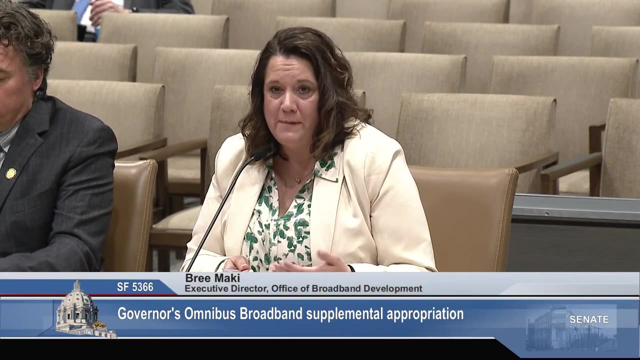 broadband dollars to the low density program. is that correct, Ms Mackey? Yes again, thank you, Chair and Senator Westrom. So yes, essentially. however, it could also look where maybe we have a really excellent application in traditional border to border, but just not enough. 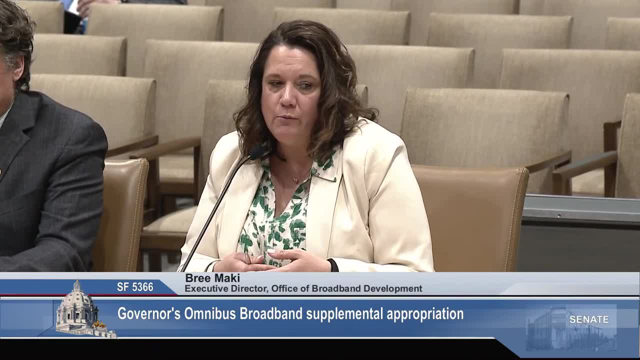 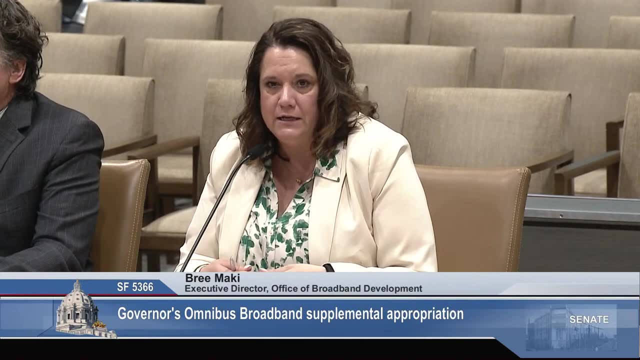 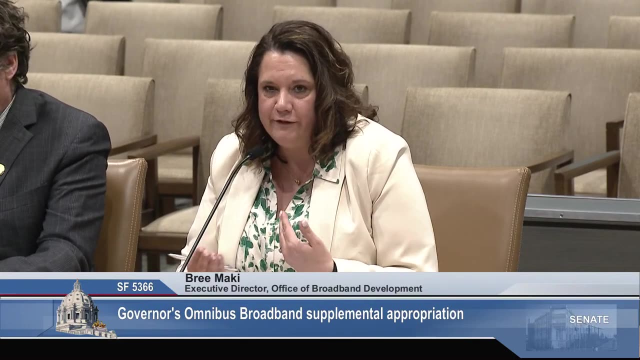 dollars and maybe less applications for the low population. We also look at local match and we have some pretty incredible counties stepping up with their ARPA funding and some additional resources and we want to make sure we're leveraging as much local match as well. so it really would allow. 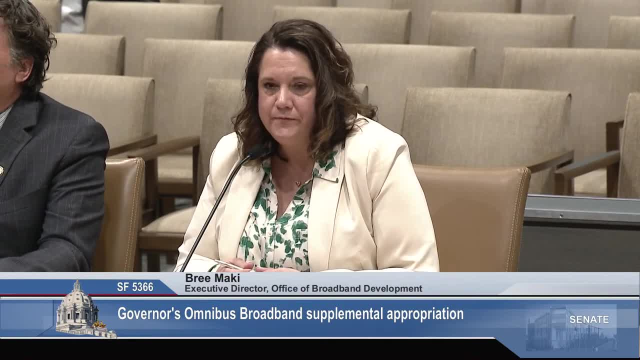 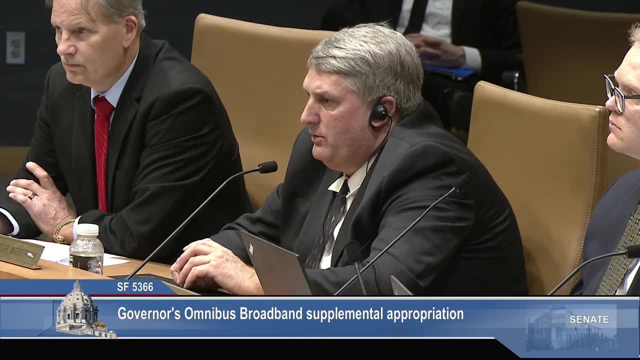 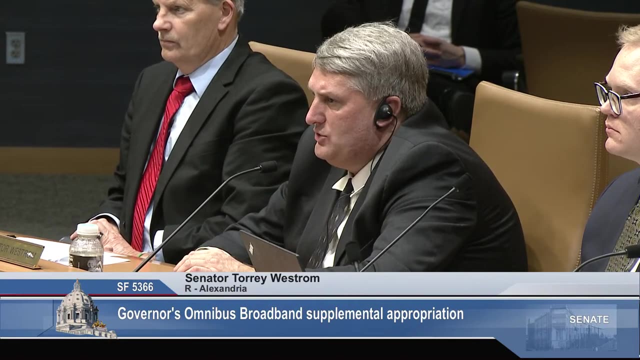 flexibility between those programs based on the applications. Senator Westrom, Mr Chair, thank you, Ms Mackey. so it could go either way. you could potentially take some out of the low density dollars and put them into the regular rural broadband if you had strong. 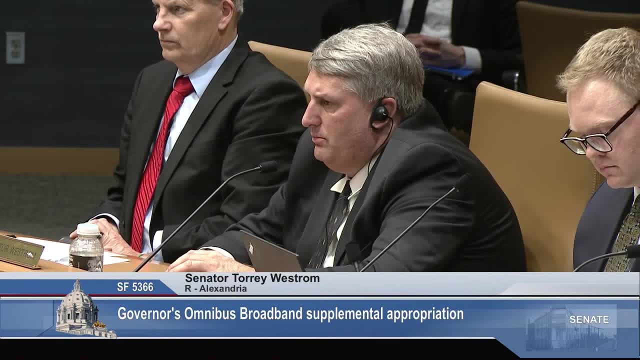 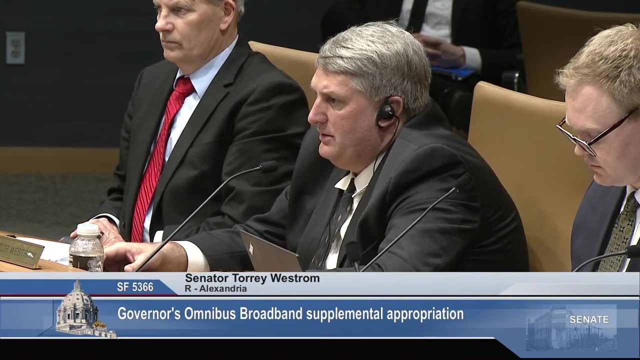 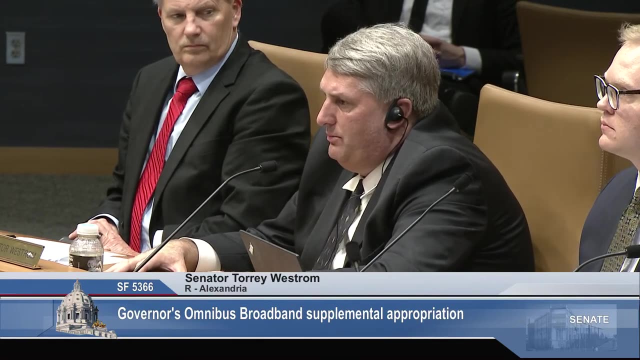 applications there, maybe strong applications with a good more match so you could stretch the money further, getting more households. and so am I understanding that right, you're going to make that kind of be nimble to make the best financial decision, the best number of homes we can reach. 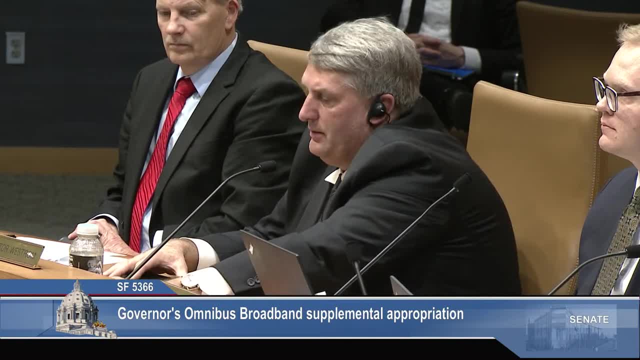 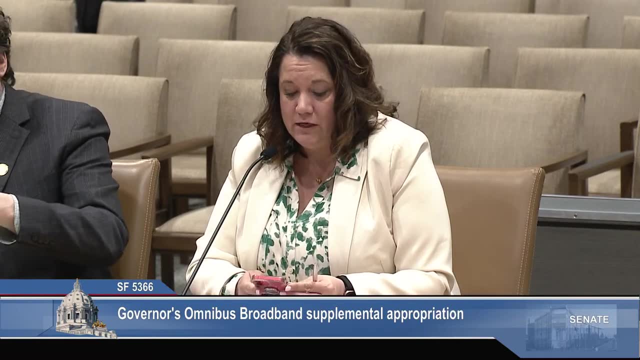 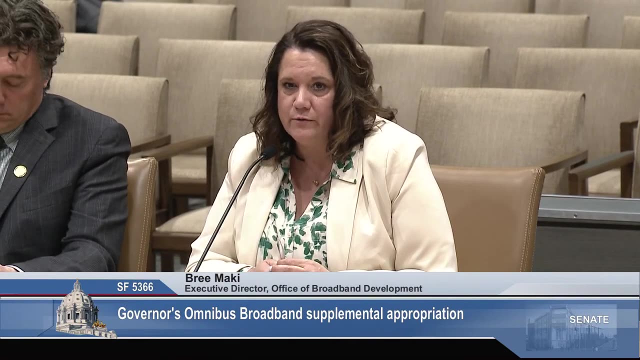 with the with the fewest dollars, if you will, Ms Mackey. Thank you, Chair, and thank you, Senator. so, yes, it's allowing that flexibility, because the last thing we have to do is not fund an application that really is solid and meets all of the goals. the 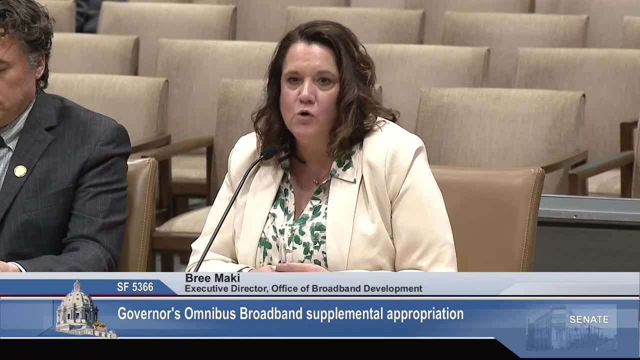 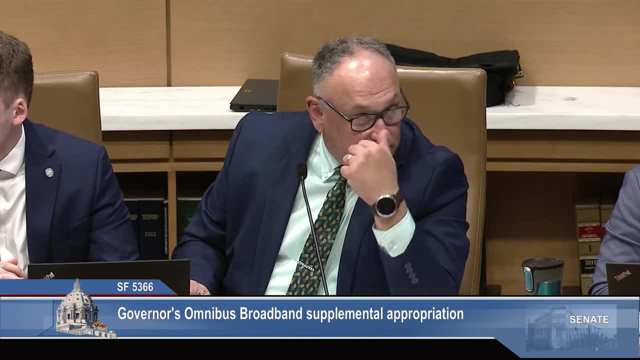 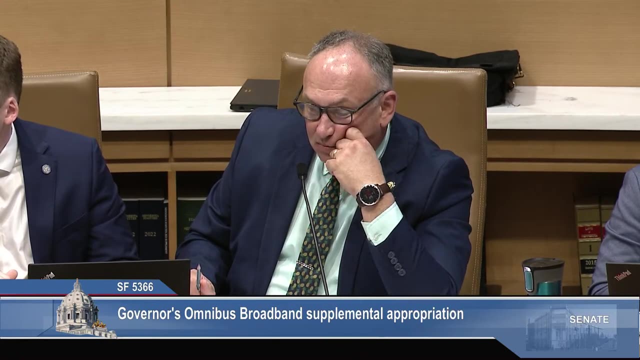 requirements and ultimately, you know, affecting the most people with the resources that we have. Senator Kunish, Thank you, Mr Chair and thank you, Ms Mackey. can you tell us approximately like: where is the greatest need? where is the least? what area has the least access? 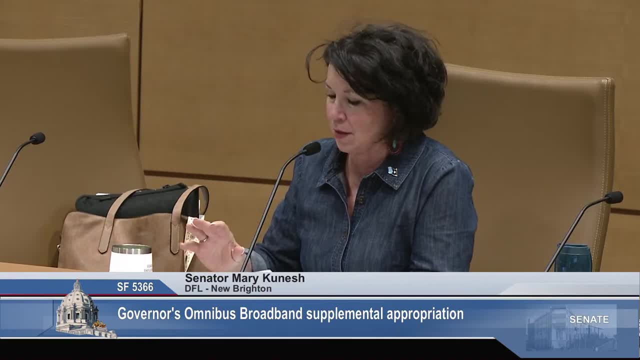 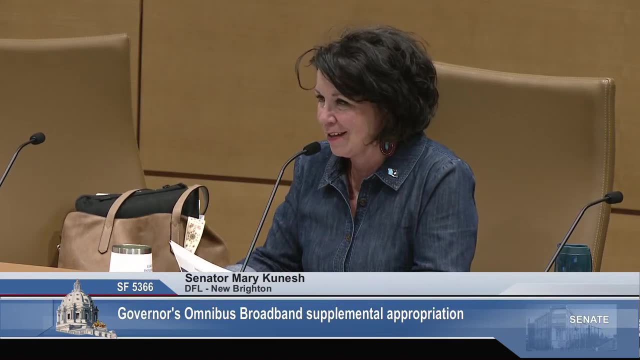 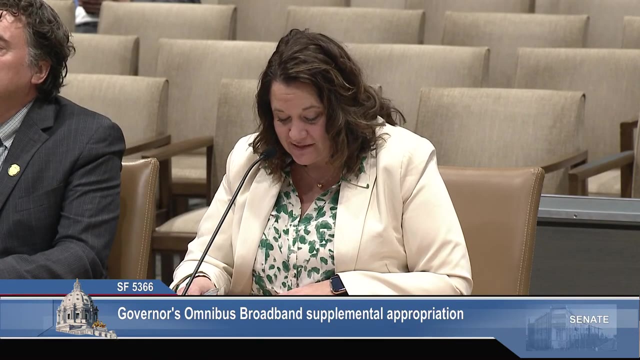 to broadband. I think it depends on whether business-wise or is it this map. I'm sorry, it's just a little small for me to see here. Is it the pink, Ms Mackey? Yes, thank you, Chair, and thank you, Senator. yes, this map is very tiny. 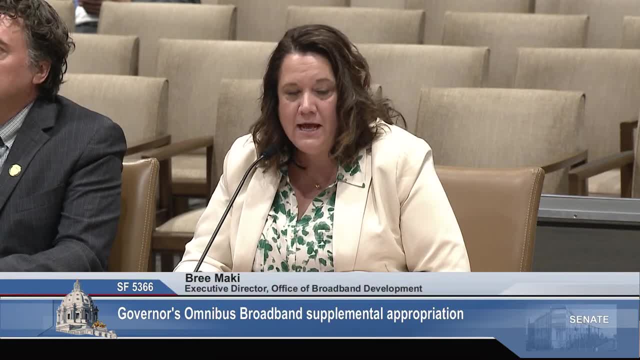 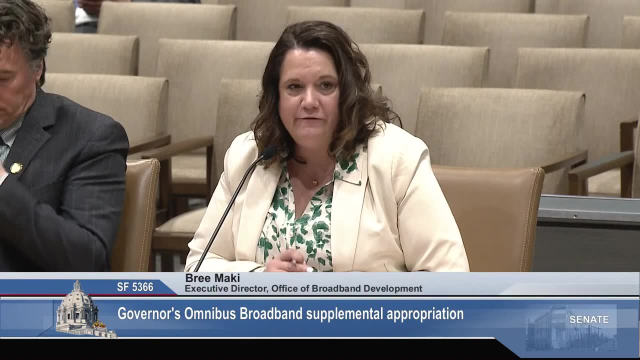 and I apologize for that. but yes, the red areas are locations that have the under 25 by 3, and we are more than happy to put together specific maps based on district if that is helpful to you. but yeah, we have a very interactive map for you to see, and so, again, just 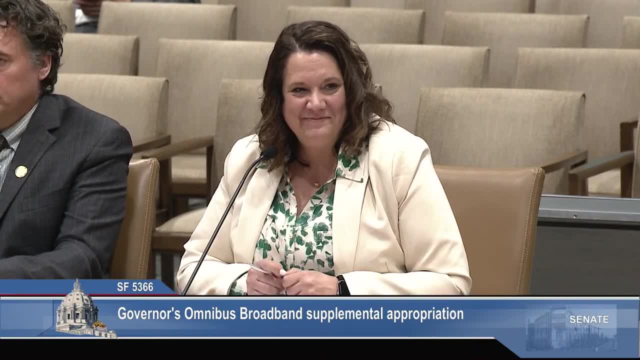 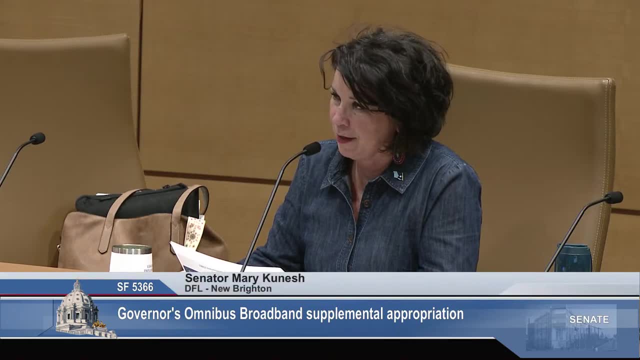 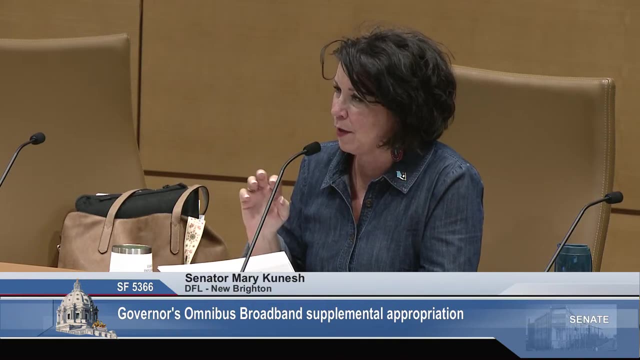 apologize, I know it's very small, Senator Kunish, So is there any? does Minnesota work with any of its neighboring states that we border? Are there federal dollars that go? you know that are interstate broadband access. do we partner with any of our neighbors- not Canada, but the rest of them. 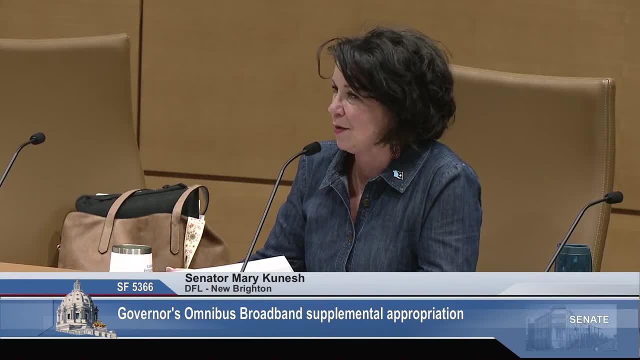 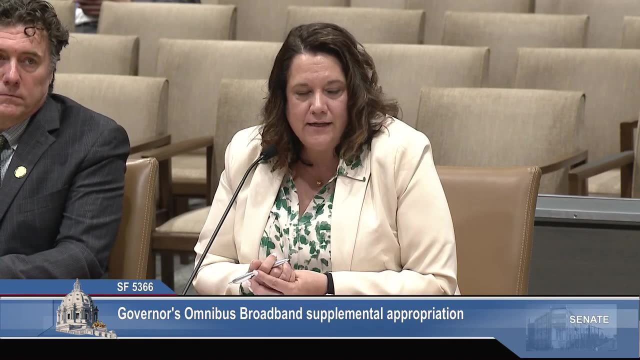 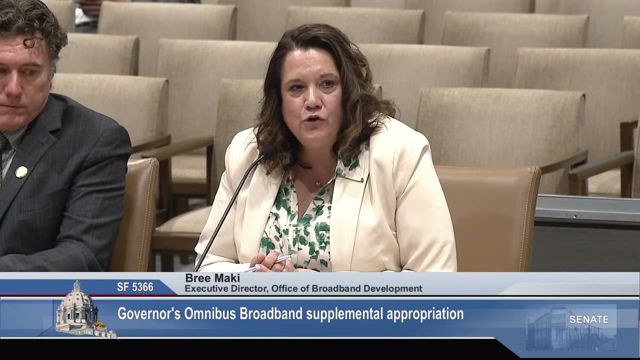 just to you know, use those dollars the very best, those federal dollars, especially Ms Mackey. Yes, thank you, Chair, and thank you Senator. I think that's an excellent question, I think you know. just remember that our broadband grants go to internet service providers, and so they're really the ones that 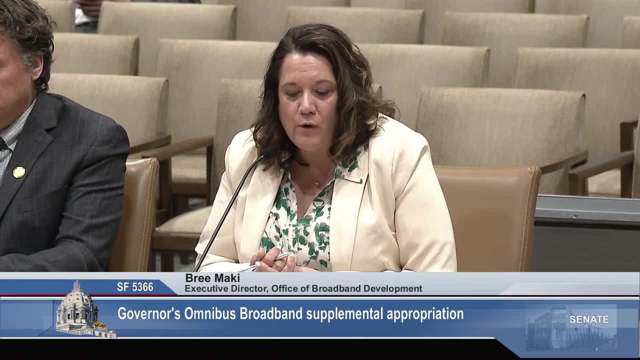 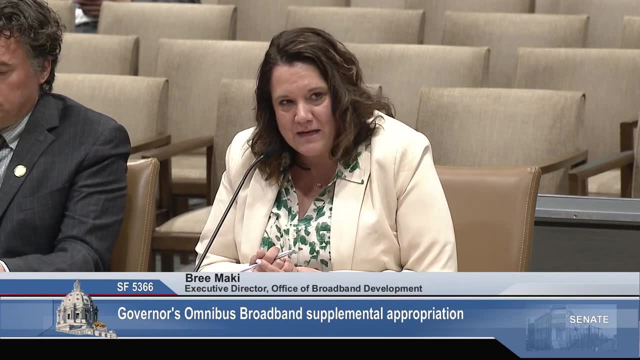 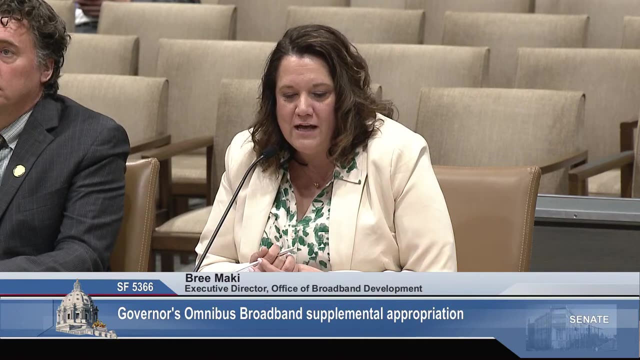 are developing the plan and working with each state individual. however, we, especially with the B dollars, are finding ourselves working very closely with all of the states, understanding best practices, what's working for them. you know how can, how can we learn from each other, and so, as far as dollars itself, 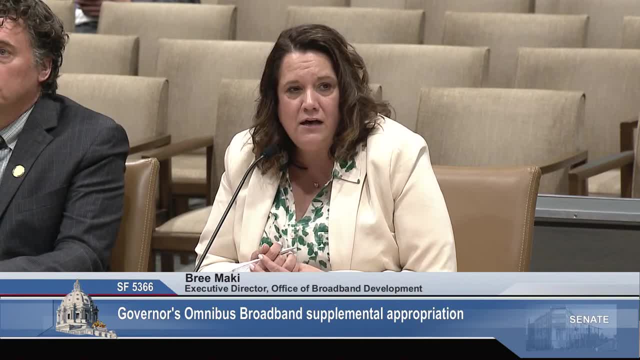 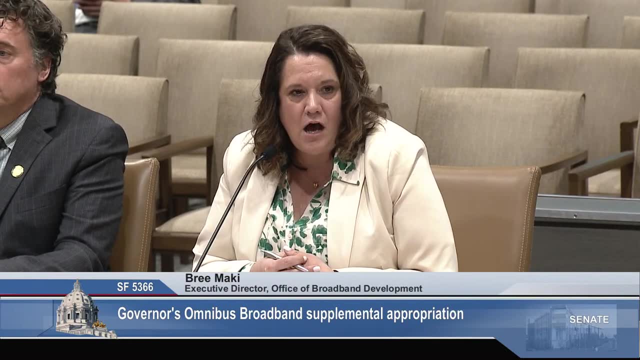 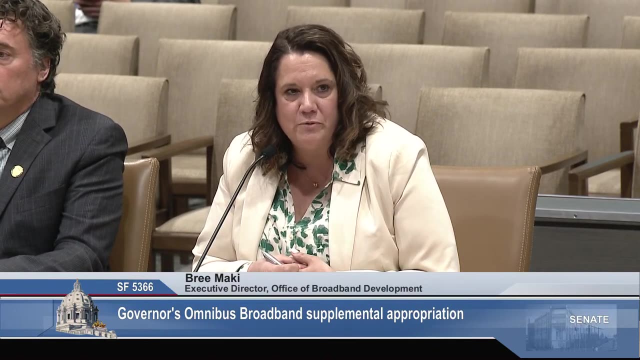 the USDA may do some of that, especially when we're working with our tribal partners, when it's the jurisdiction is a little bit partnering a little bit more. but ultimately, you know, the state dollars are the state dollars and we rely on our internet service providers to put those applications. 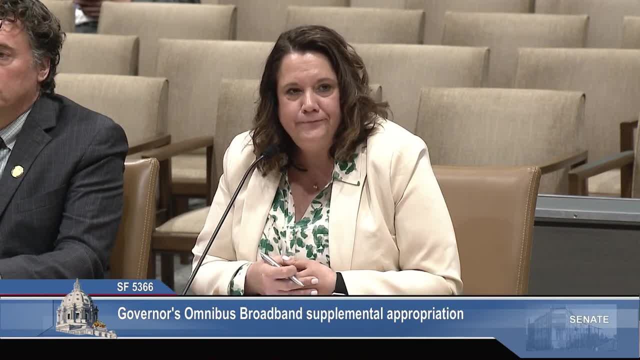 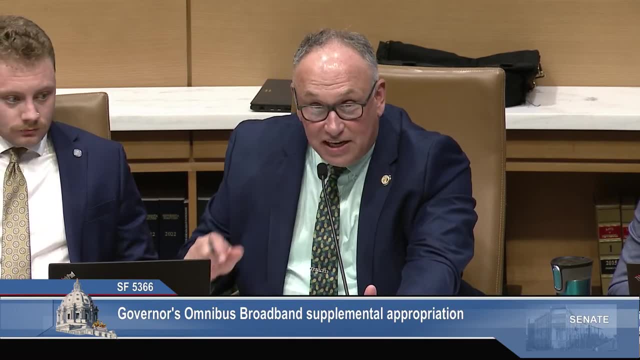 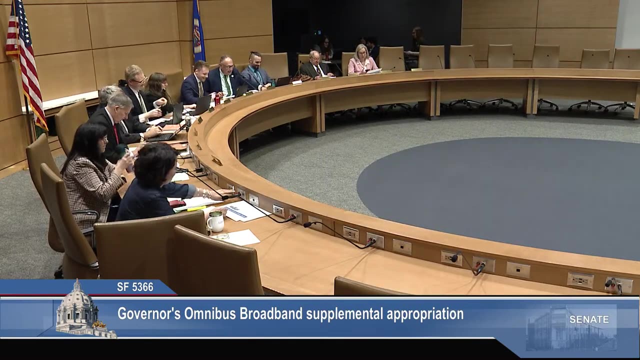 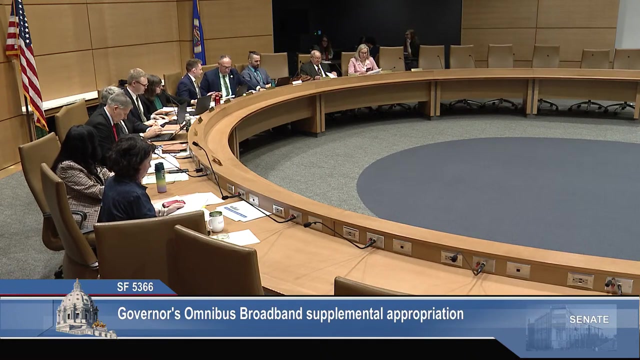 in for Minnesotans. Thank you, Any other member questions? If not, thank you for your presentation. Any closing comments, Senator Putnam? Thanks, Mr Chair. You are welcome And we will be. So we're laying this bill over and. 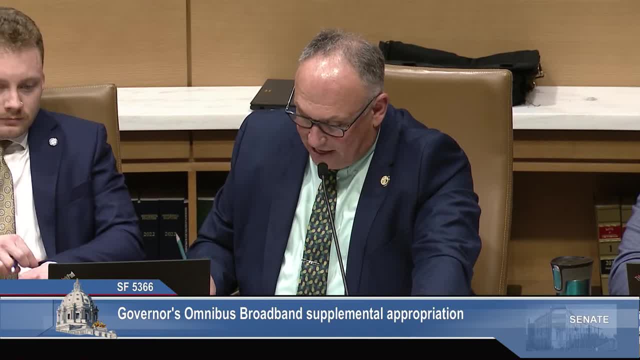 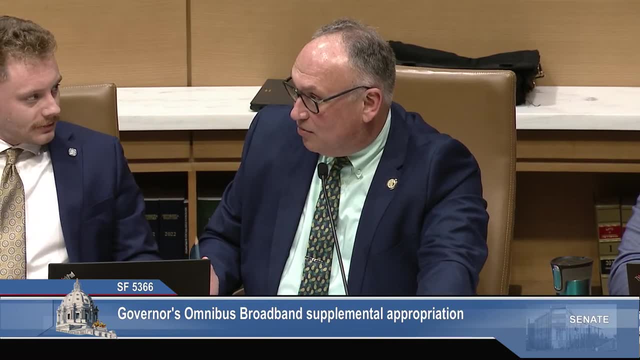 then this brings us to Senate file 3955, which is the omnibus supplemental agriculture finance bill. and just as a reminder, we are just doing a walk through today and then we will do member discussion and a few amendments on Wednesday. We do have testimony today. 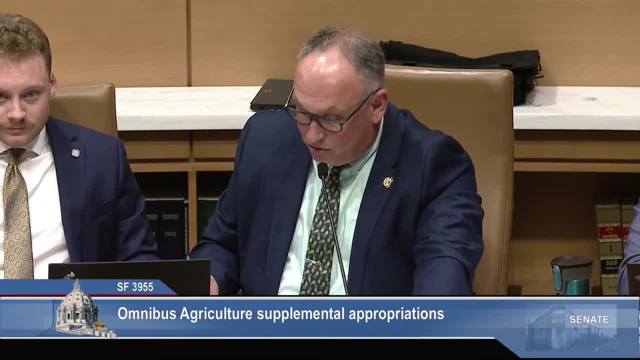 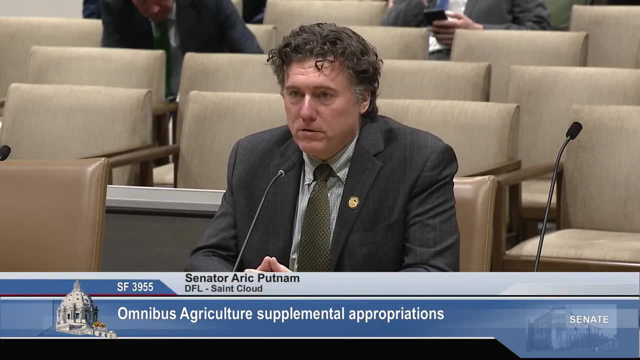 So to that, Senator Putnam, would you like to start us out? Thank you very much, Mr Chair and members, I just am going to say a few things very briefly and then we'll turn it over to Ms Painter to walk it through and also to Mr Olofsson to talk about. 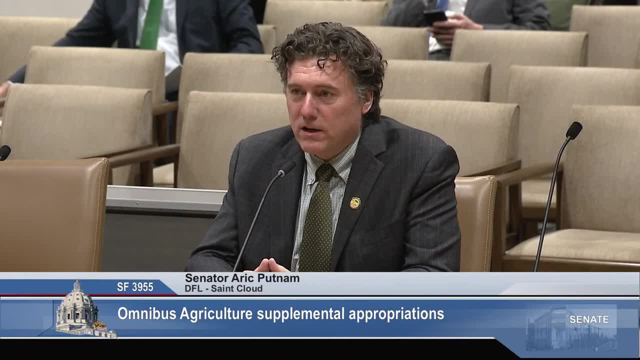 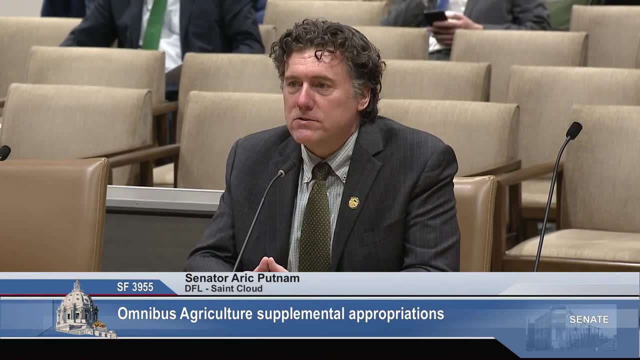 how much everything costs. and then we have a couple testifiers here who are here to say great things about the bill. I hope Members, this bill is, I think, incredibly balanced. if I had to pick one word to describe our approach to our supplemental budget this session, I 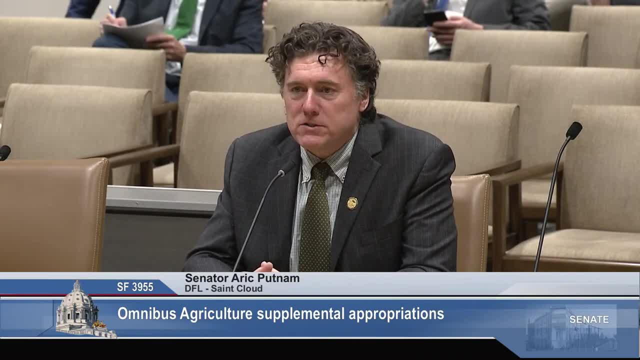 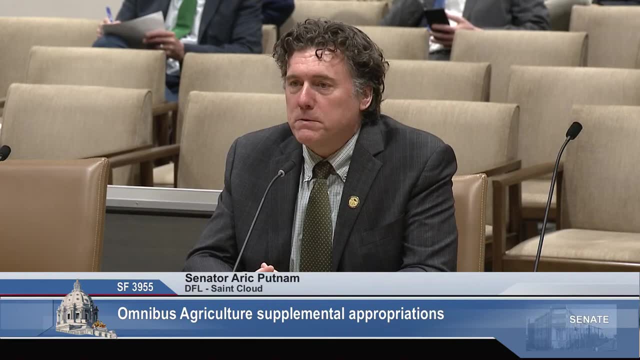 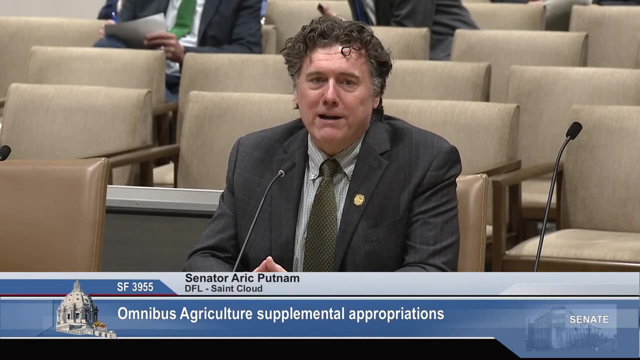 would use that word- balanced. It's balanced between immediate, pressing, acute concerns and the long term vitality of Minnesota's agriculture that is our responsibility to grow. It's balanced between dairy corn, soy, big producers and small producers. There's something in this bill for. 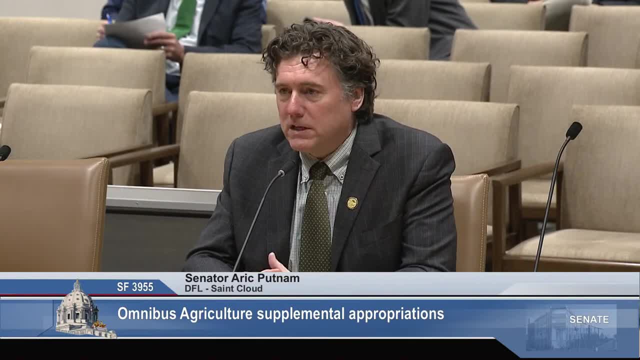 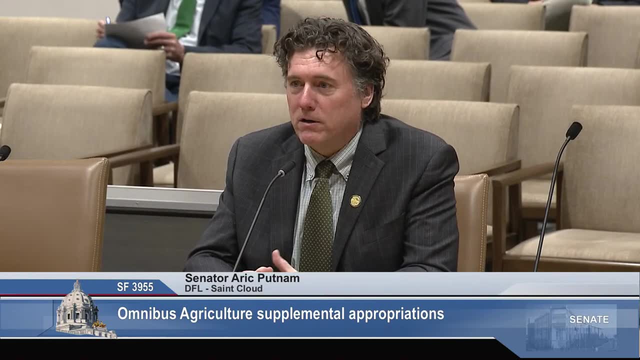 everyone in Minnesota- agriculture- and there are a couple in particular initiatives I'm especially proud of. Of course, one of them has to be turkey lasers. I'm very glad that we are going to be thinking about the long term health of Minnesota by doing the appropriate. 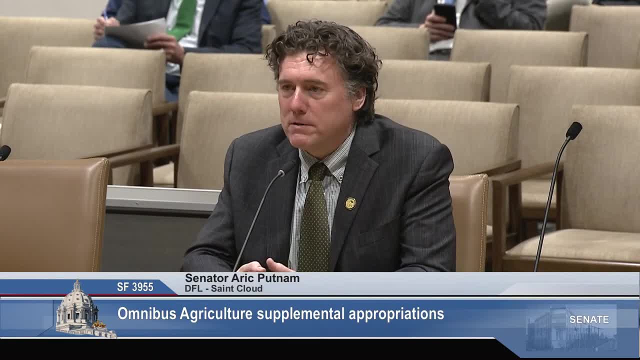 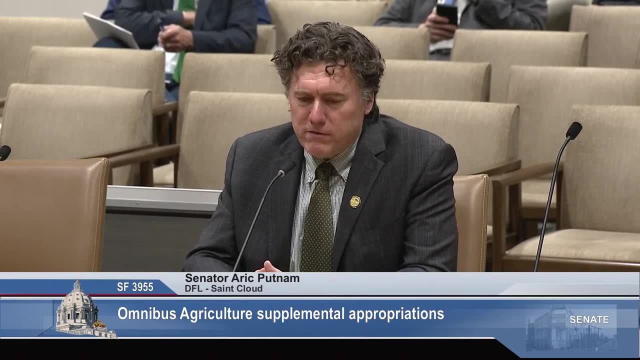 move, which is to anticipate a problem before it happens and take care of it before it occurs, Which is one of the things that our turkey laser initiative will do, Also in terms of investment in the future. in terms of workforce, we have Senator Dornick's 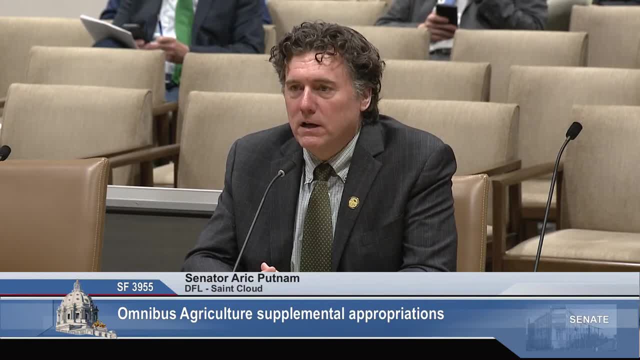 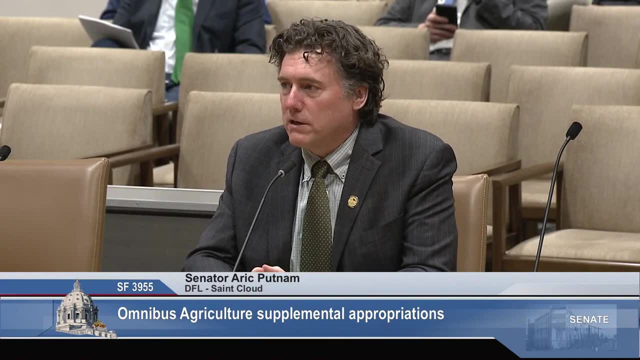 bill for meat packing, meat cutting. getting more people into that industry is another thing that I think is an essential dimension of this bill, But ultimately, one of the issues that we're probably going to talk the most about is the nitrate concern in the Carson region. 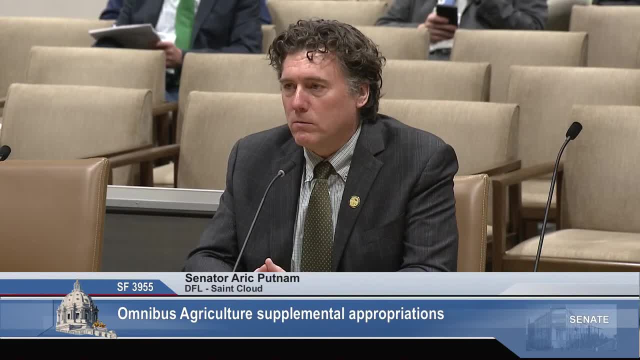 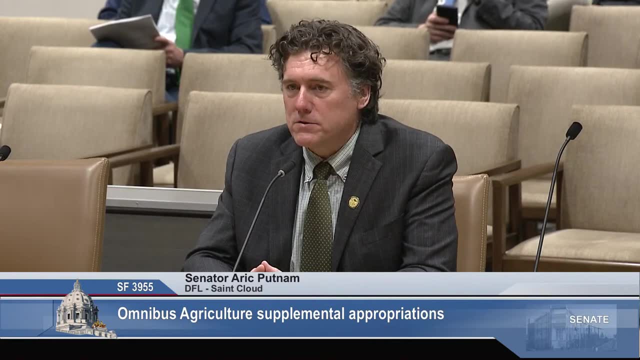 and I'm especially proud of how we've approached that. Given the resources that we were given, we were tasked to dedicate some of those resources to the Department of Health, who will take care of some of those concerns, but we also took some left over of the rest of our money. 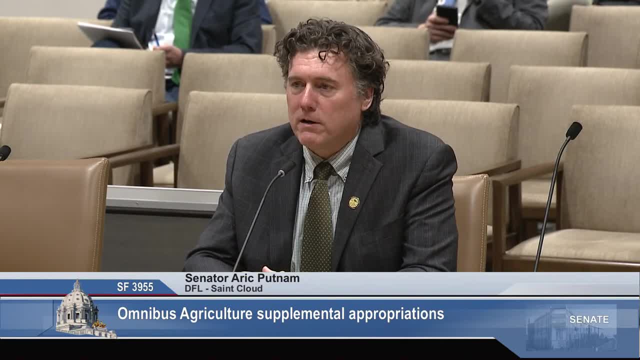 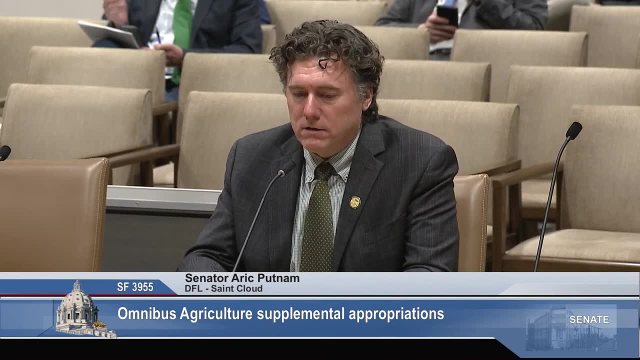 and we articulated it to those folks with wells who are in the greatest need. So the $750,000 for nitrate remediation in the Carson land is going to be dedicated to folks who make less than 300% of the federal poverty level- Folks who have the greatest needs. 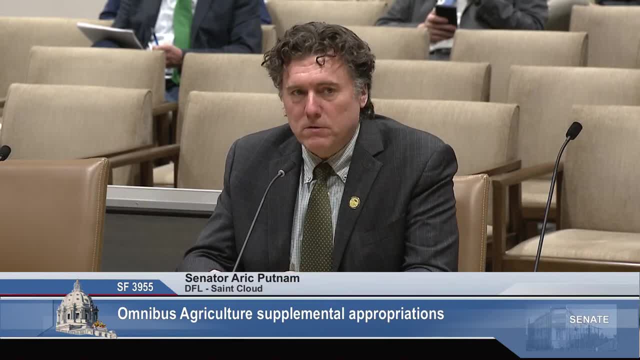 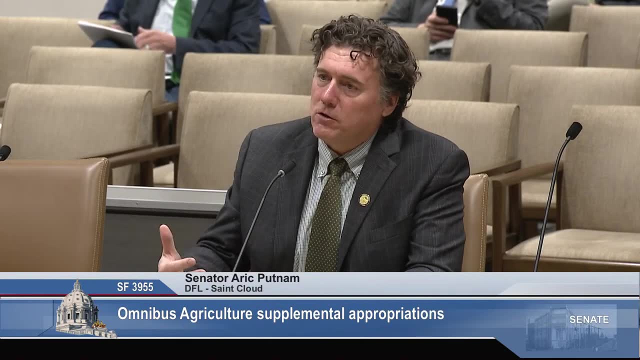 will get the help we want to give them. But there's something else that we're doing, which, again, is something I'm particularly proud of, and that's our investment in soil health And instead of just adding to the soil health program, which is already over, 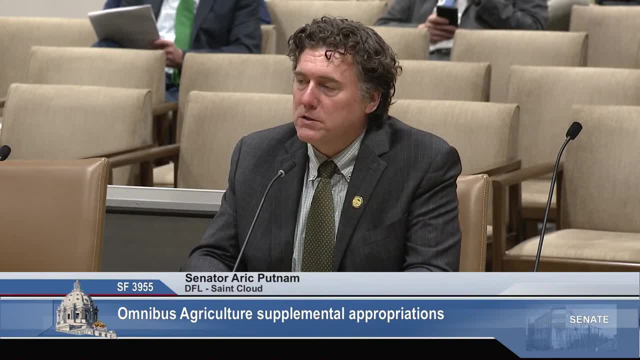 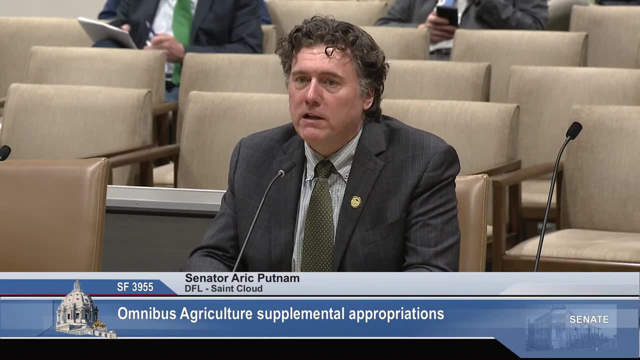 subscribed, we've decided to dedicate those resources to those who want to do soil health practices in the Carson region specifically. So, all told, we're putting 3.25 million dollars towards this pressing concern that is directly in front of us, but we're doing so in a responsible way. 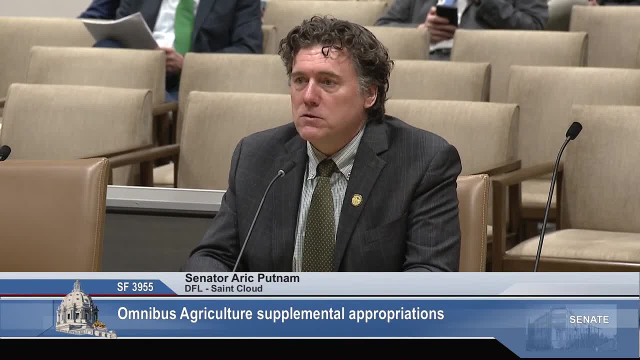 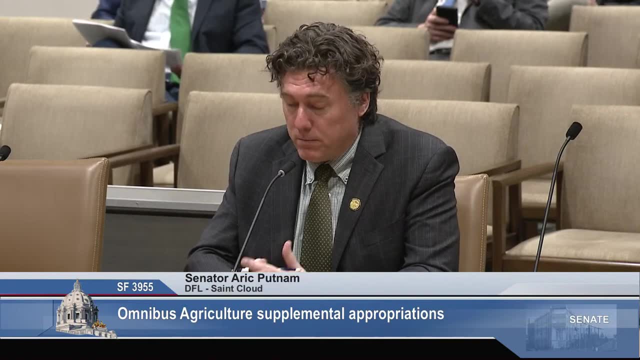 that will help people do new practices so that this problem that we've got right now will not still be a problem in 20 more years. So, Mr Chair members, I'm very proud of this bill and eager to talk about it. Great Thank you, Senator Putnam. So, 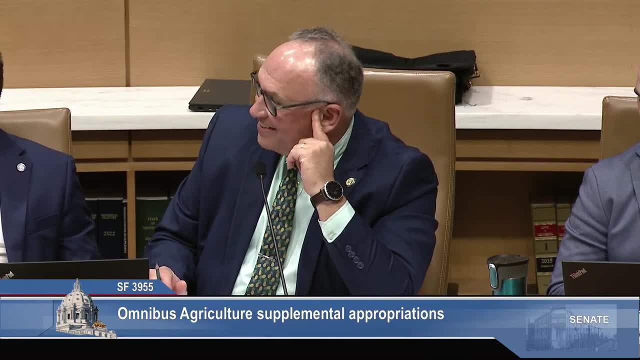 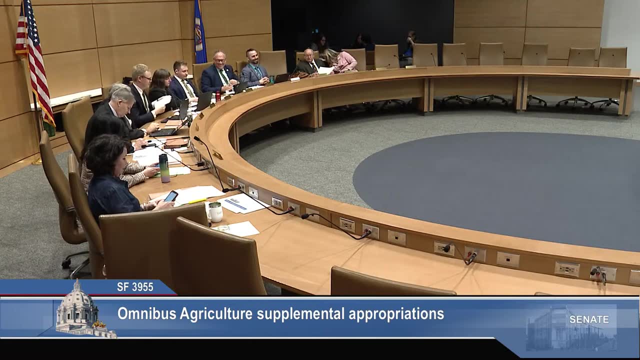 with that, we will turn, I think, first to Ms Neera Olson, who will do a walkthrough of the financial side of it. Thank you, Mr Chair. Members of the committee, in your packets you should have a spreadsheet with a date and time of 4-13. 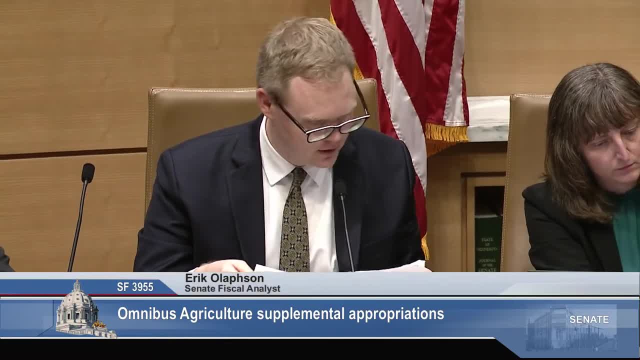 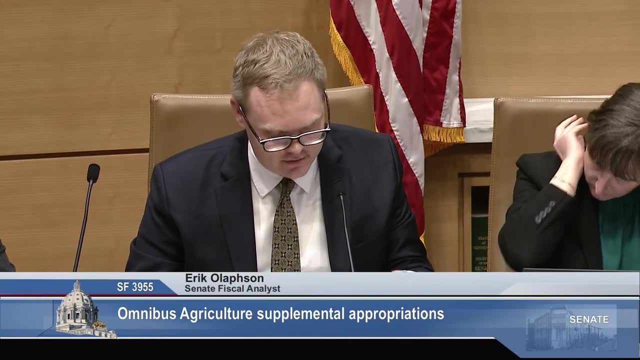 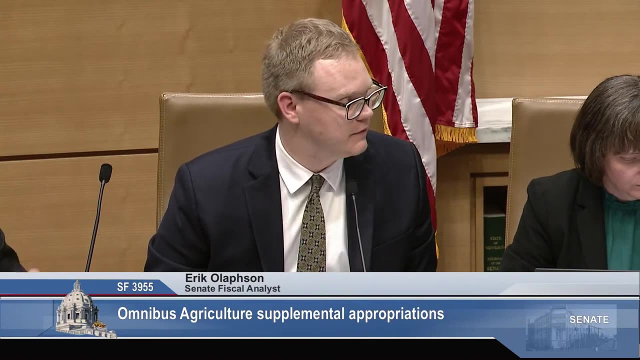 2024, 1052 AM in the top right corner. And this is summarizes, primarily summarizes article 1 within the senate file 3955 DE amendment. So just to give you a basis. so the Ag committee received the target for the 24-25. 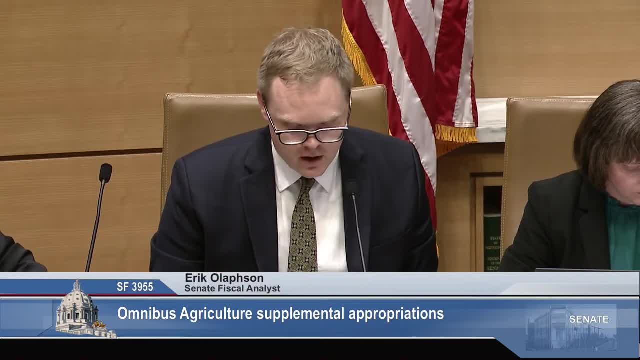 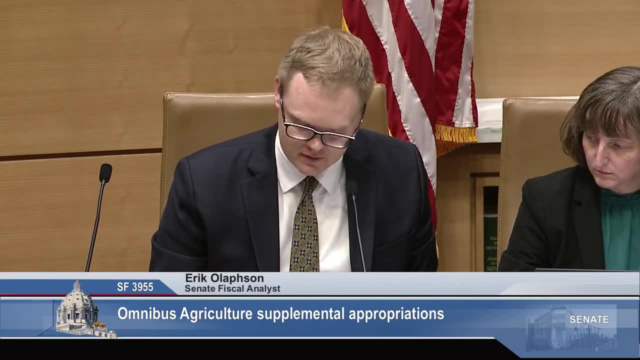 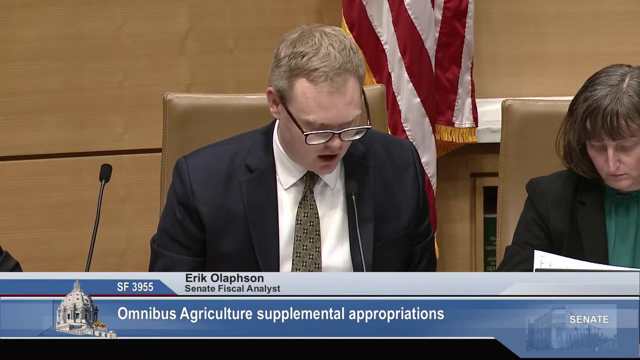 biennium from the general fund of 4,545,000 dollars And in the tails of 2,576,000 dollars. This bill in front of you meets those general fund targets. So in the spreadsheet in front of you, column A discusses the different appropriation. 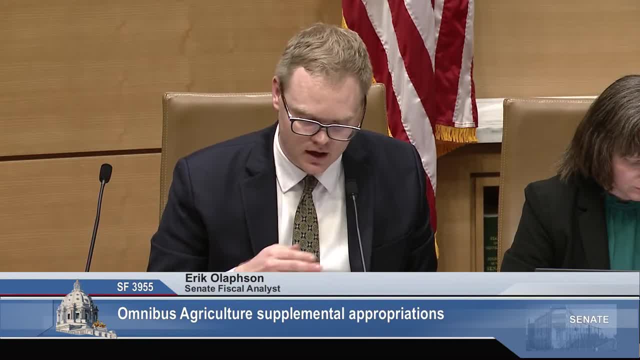 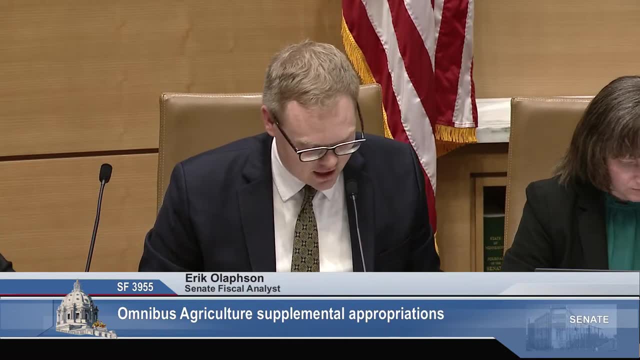 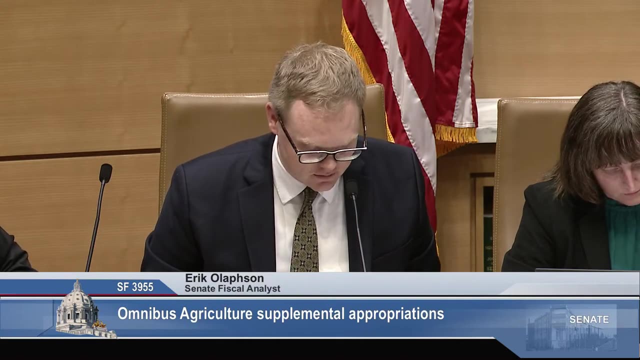 items, and then columns F through K, summarizes the senate position before you. So, starting with the department of agriculture, on line 8 of the spreadsheet for nitrate treatment, specifically for reverse osmosis systems in southeastern minnesota counties, with priority given to households up to 300. percent of the federal poverty guidelines and for households with infants and pregnant individuals, There is 750,000 dollars one time funding in FY 2025, with extended availability through FY 27.. On line 9 for soil health equipment grants specified in southeastern minnesota counties that's. 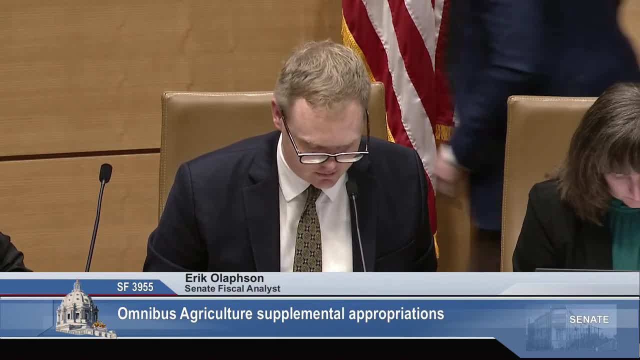 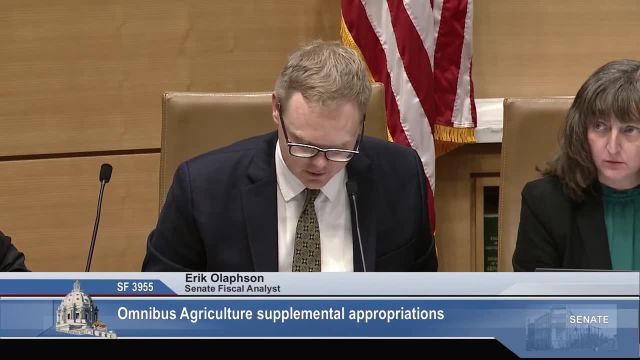 500,000 dollars one time in FY 25, again with extended availability. On line 10 there's an increase to the elk depredation payments. this modifies chapter 43 from last year of additional 75,000 dollars from the general fund. 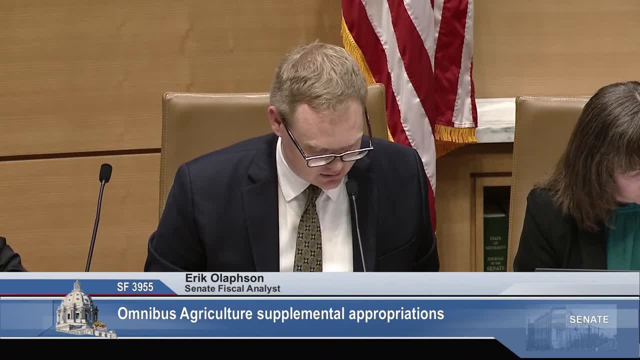 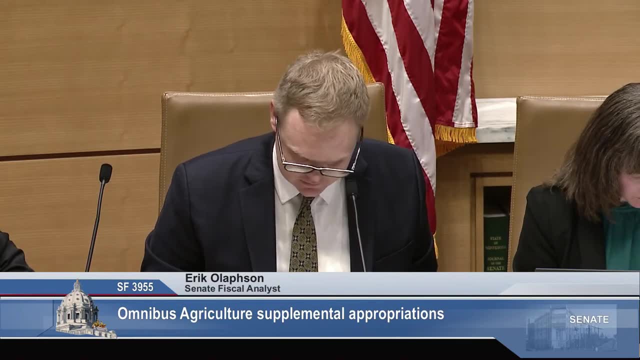 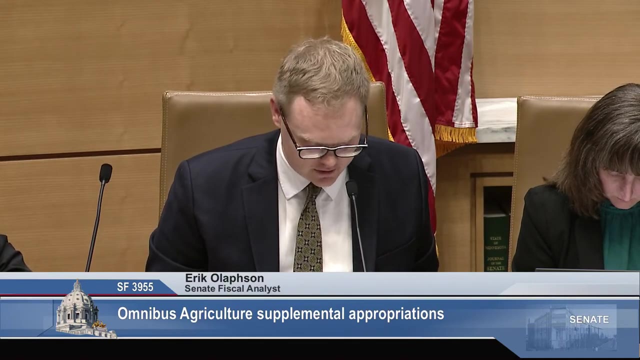 On line 11 for server day abatement. this is for a report on server day abatement and crop and fence damage. so it's 50,000 dollars one time in FY 2024, with availability through fiscal year 25, to get that report done. 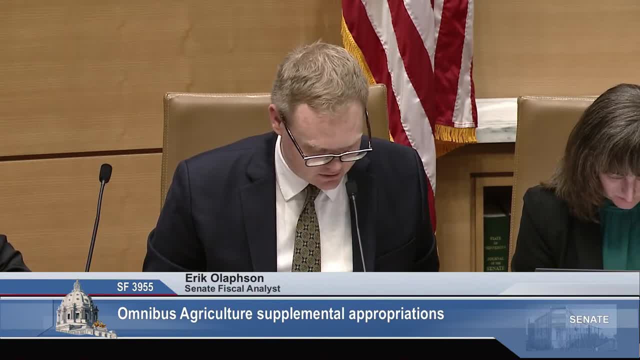 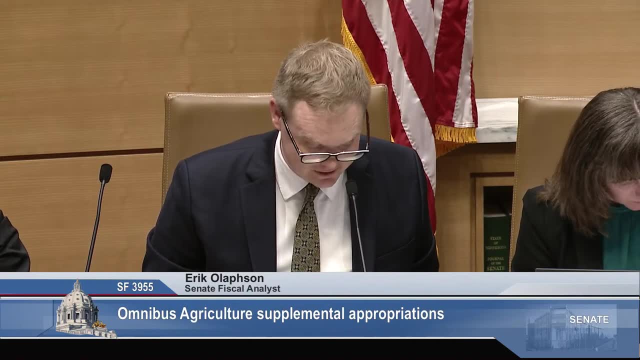 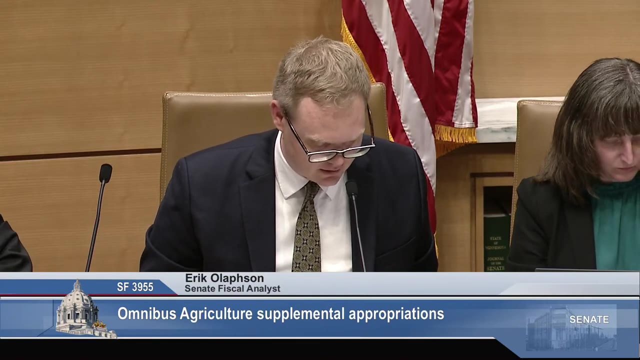 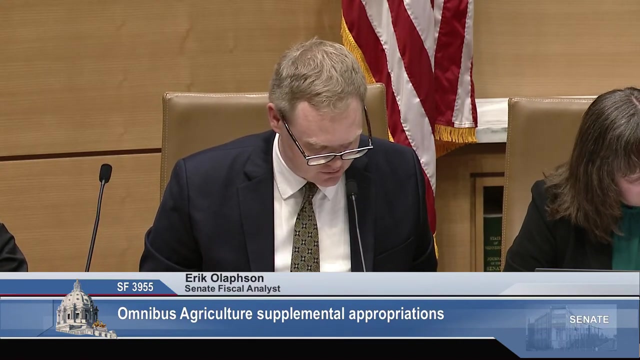 Moving on to promotion and marketing within MDA there's a modification to the dairy development and profitability teams. this actually happens in a later article, but the appropriation is within article 1, so that's a budget neutral item. On line 15 there's another budget neutral item is 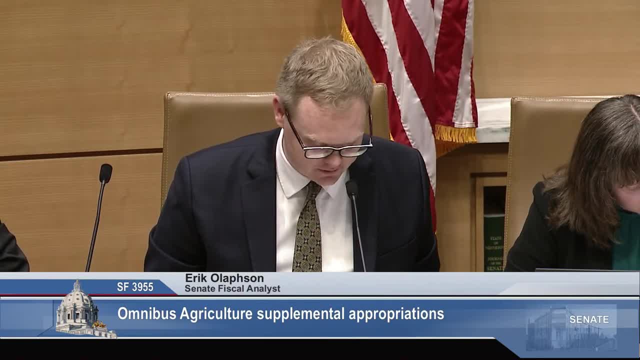 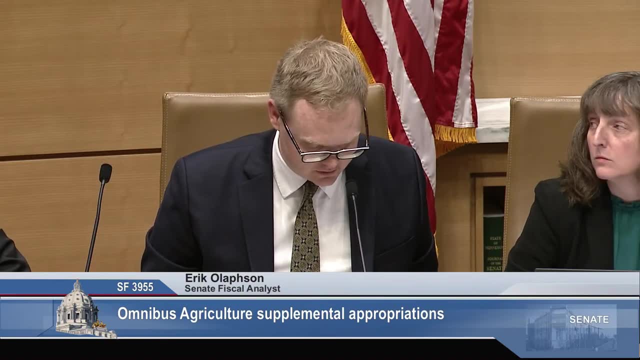 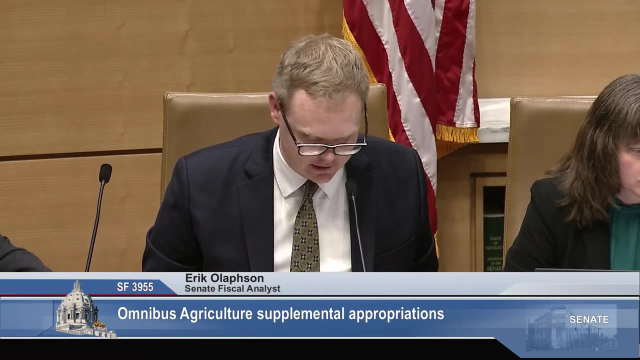 technical changes to the farmers market grants. this comes from senate file 3404.. On line 16, following the governor's budget language in senate file 5635 there's a tails increase for maintaining current service levels of 20,000 dollars in fiscal year 2026 and 20,000. 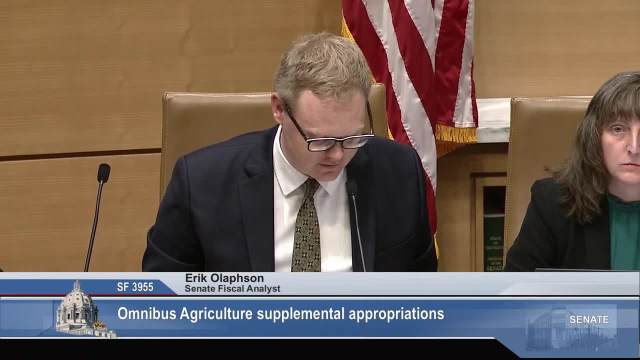 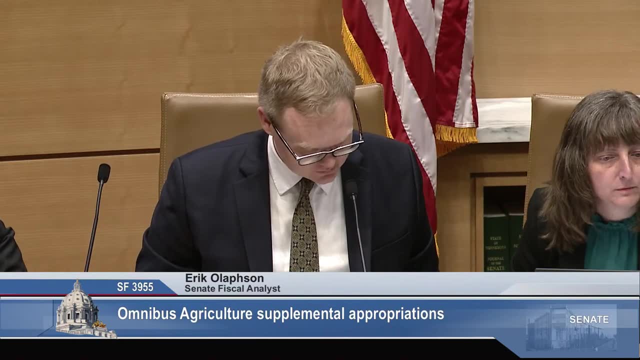 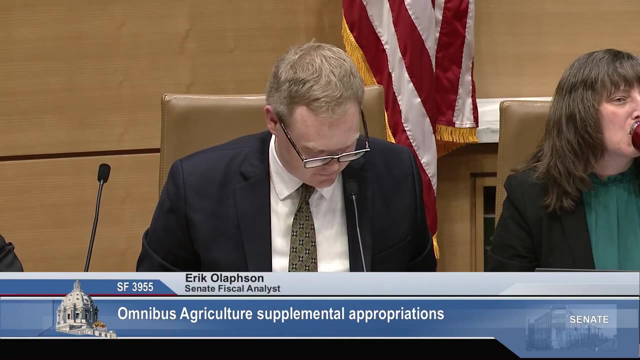 dollars in fiscal year 2027 there's a corresponding decrease that I'll mention in the administration financial assistance division at MDA, Moving on down to line 19, that's the budget neutral item for the farm to school program to also include early care providers. that expansion. 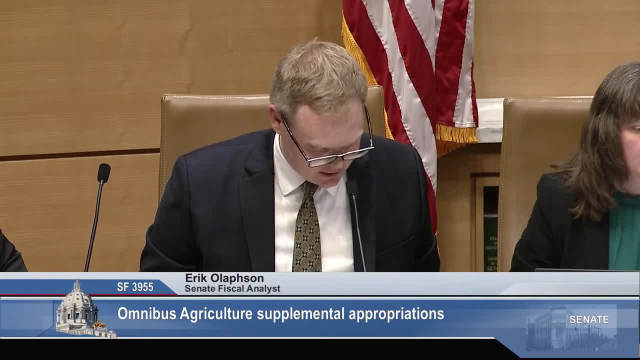 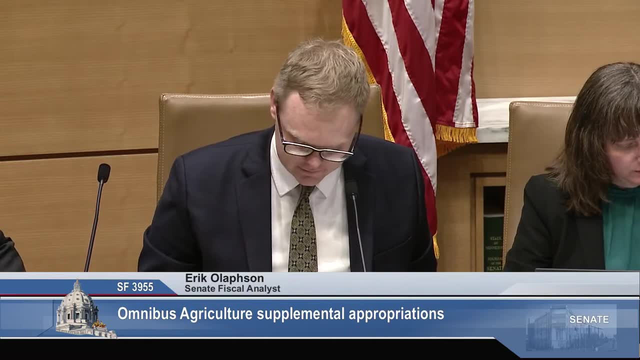 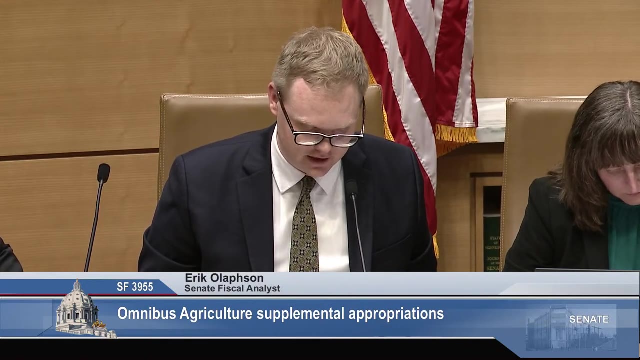 which is budget neutral. On line 20: this is a one time increase to farm to school of 100,000 dollars from the general fund in fiscal year 25. if those funds are not fully utilized by the end of fiscal year 25, they can be used. 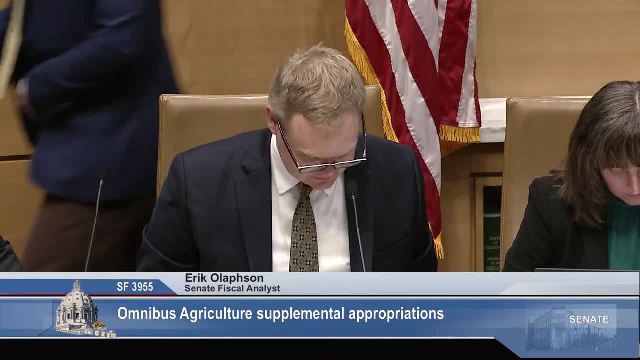 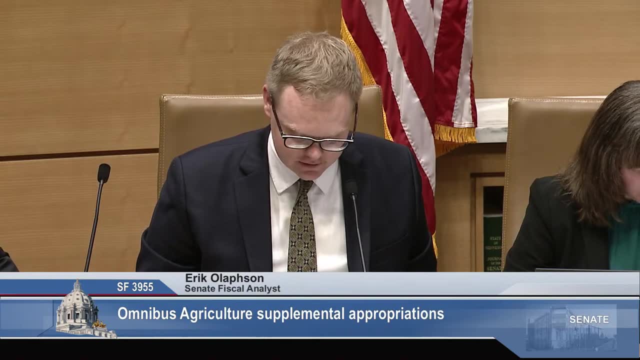 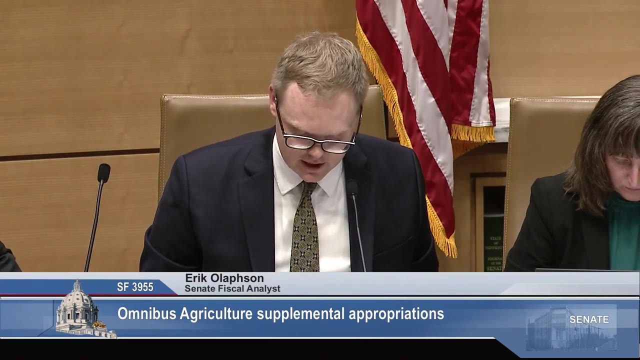 for other purposes under AGRI On line 21. this is the additions to AGRI's undesignated funding. so there's an additional 345,000 dollars in fiscal year 25, then an additional 1.288 million each fiscal year in the tails. 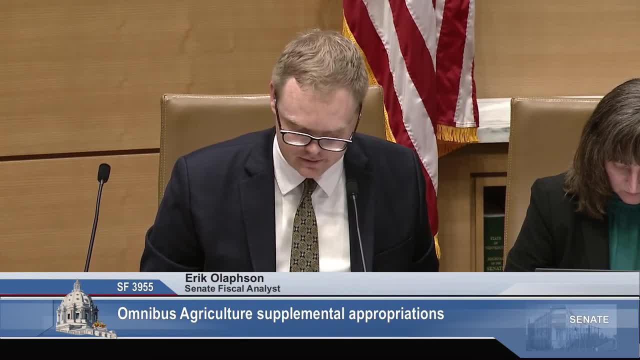 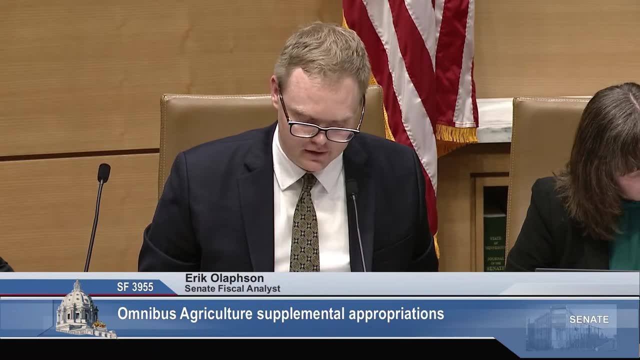 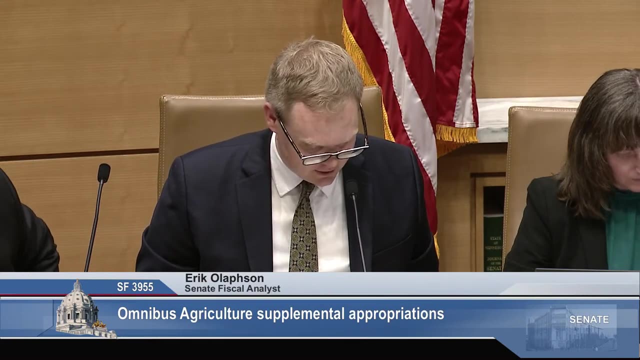 for a total of 2.576 million from the general fund to go towards undesignated funding within AGRI. So that's the entirety of the tails target goes towards that purpose. On line 22 there's the dairy cancellation in fiscal year 2024. this is due to us. 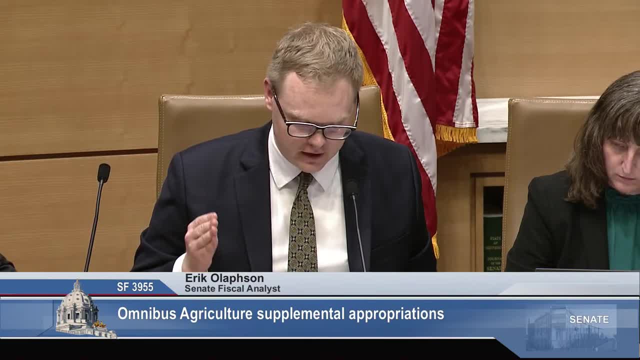 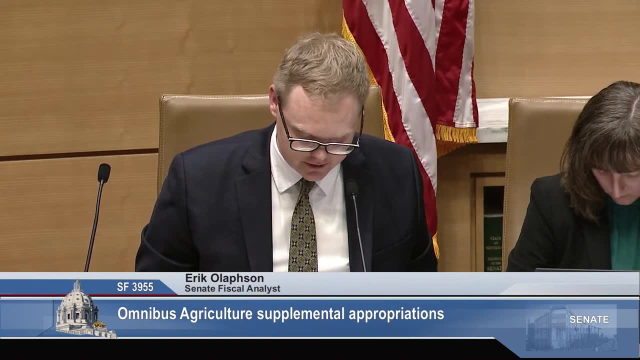 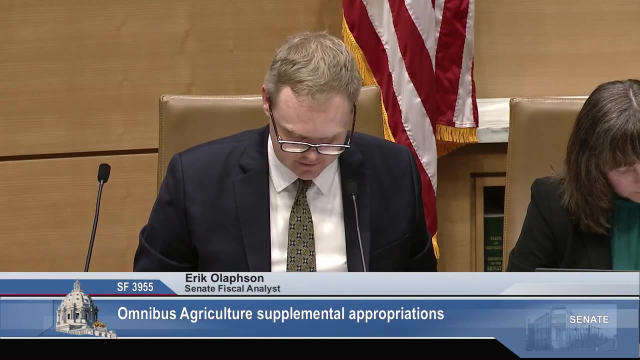 canceling the AGRI program in FY25 and then reappropriating it all with extended availability. that gives MDA additional flexibility. So on line 23 you can see dairy with an I program is reappropriated with extended availability. that 4 million dollars. 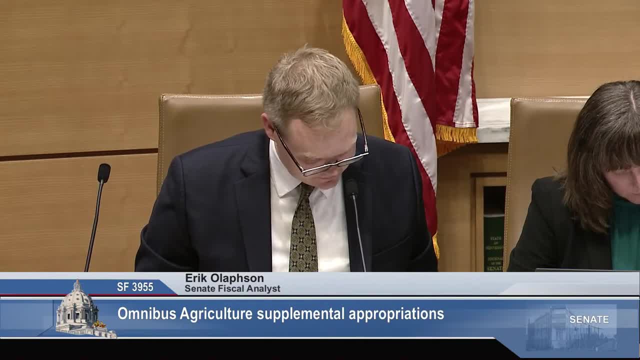 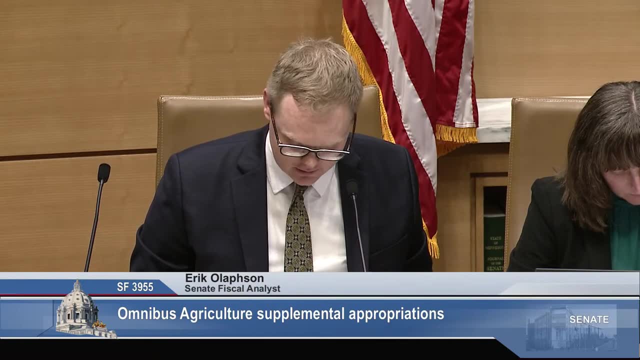 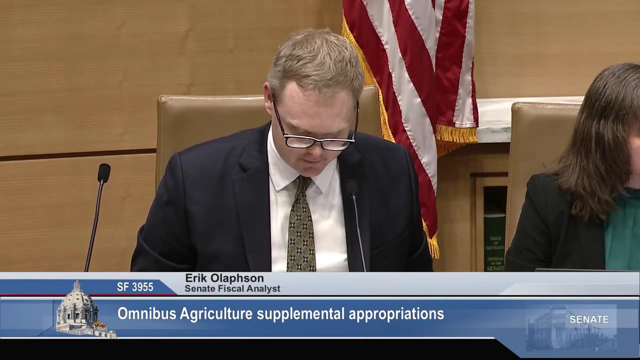 is reappropriated on line 23.. Line 24 shows the cancellation of the 23.107 million from AGRI in FY25, but on line 25 it's reappropriated for the same purposes, with extended availability of the same 23.107 million. 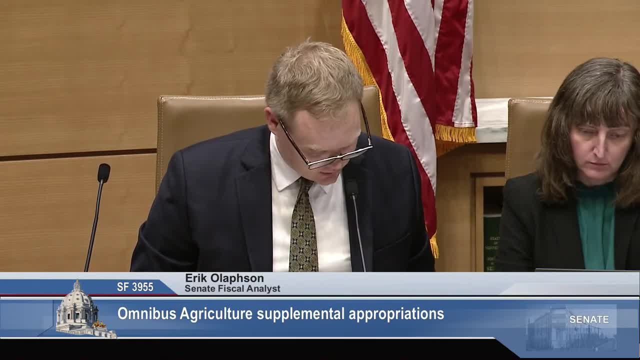 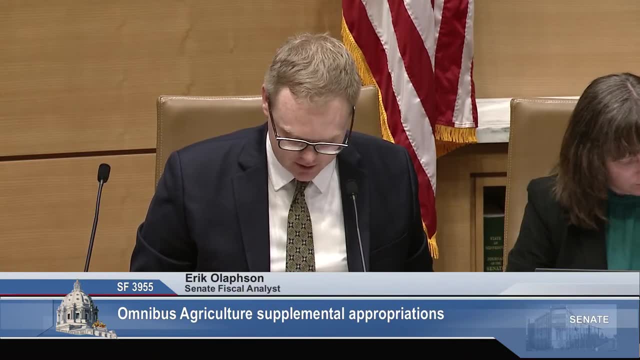 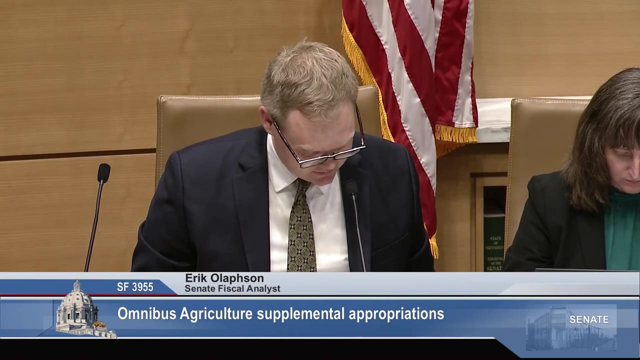 from the general fund. On line 26, this is the livestock protection grant specified for avian influenza: one time appropriation of $300,000 in FY25 with extended availability. On line 27, this is $375,000 in FY24 for the meat processing. 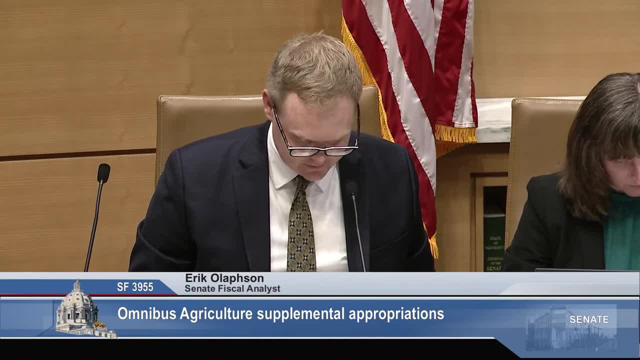 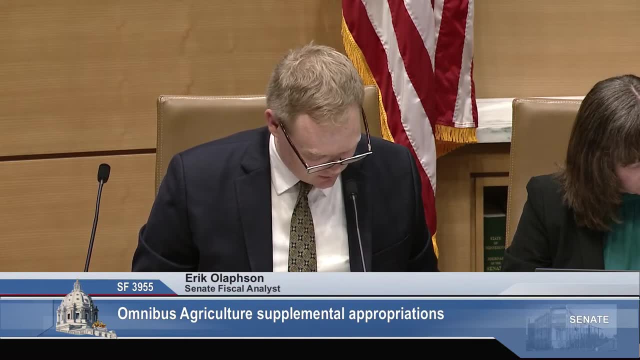 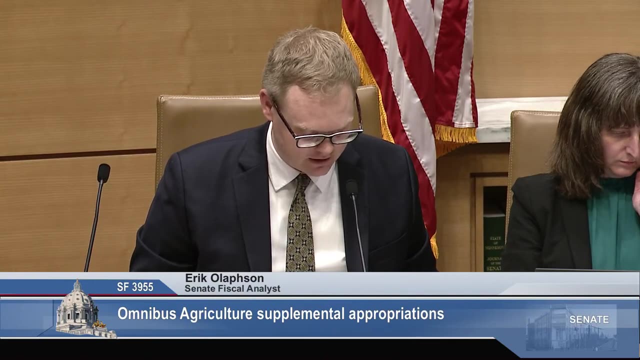 education grants. this is Senate file 4069, with. the only alteration is that it's now within the AGRI program On line 28. these are the items that we are now designated funding within AGREET for wild rice: natural stands of $200,000. 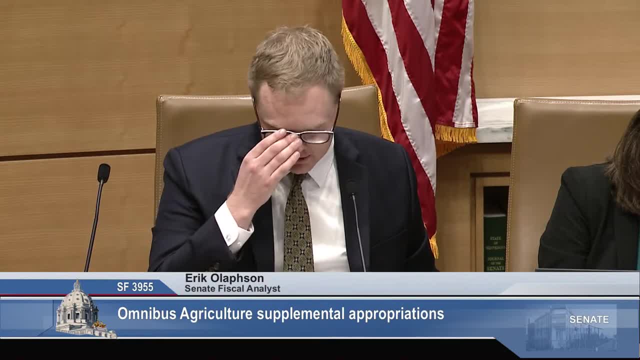 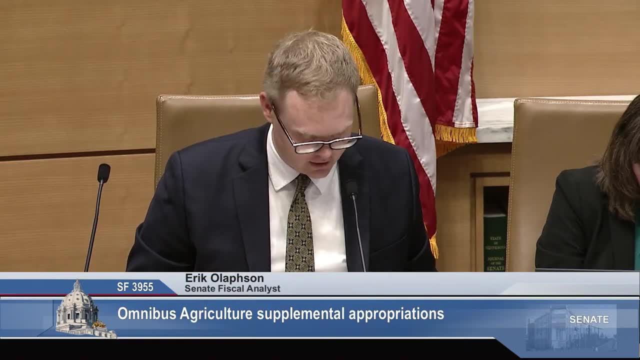 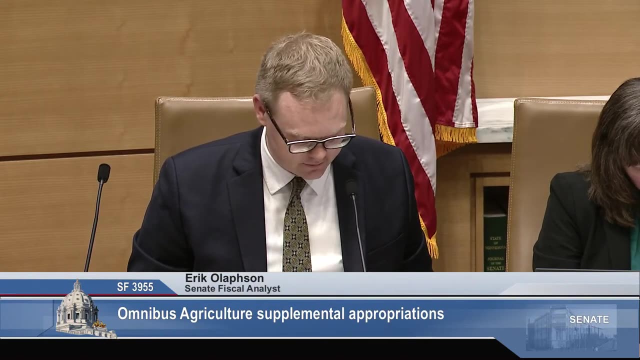 each fiscal year beginning in FY25.. This was already within the AGREET appropriation but now it's being designated so it's not adding to the general fund target. Again on line 29, this is for the wild rice forward selection part of AGREET. there's $250,000. 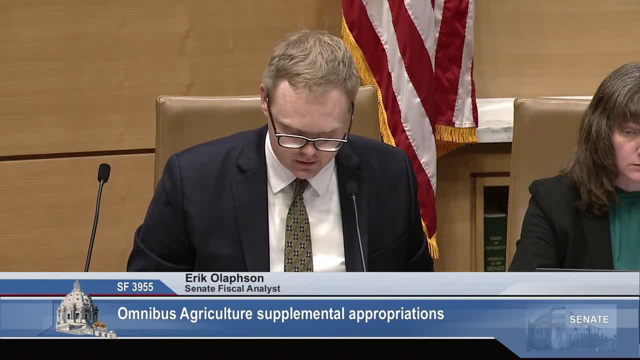 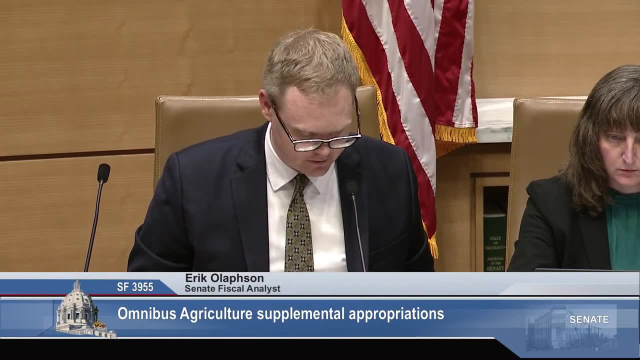 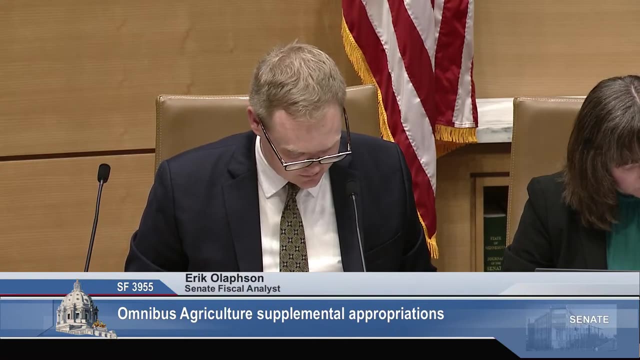 ongoing designated towards that purpose from the general fund beginning in FY25.. Again, it's designating funds that are already within the AGREET program. On line 32. this is the budget neutral item that just summarizes the down payment and assistance modification to now being. 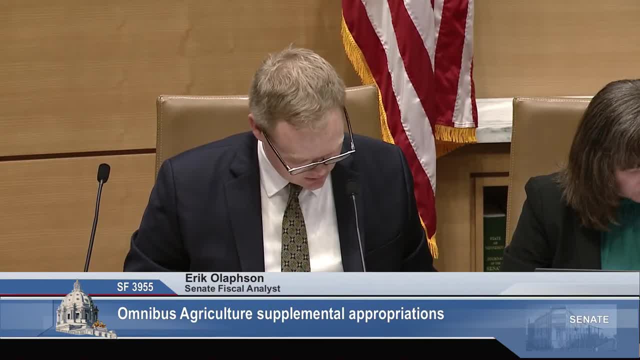 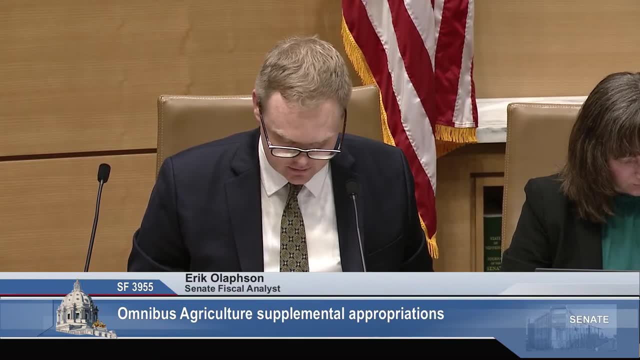 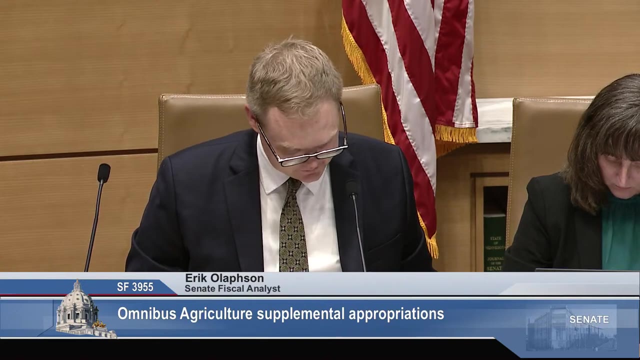 for farmers experiencing limited land access. On line 33 for an agricultural land trends report. this comes from Senate file 3913. it's $50,000 one time funding in FY24 with availability for the second year to finish the report. On line 34. 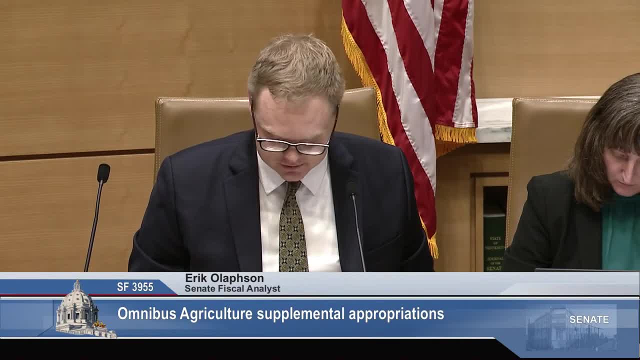 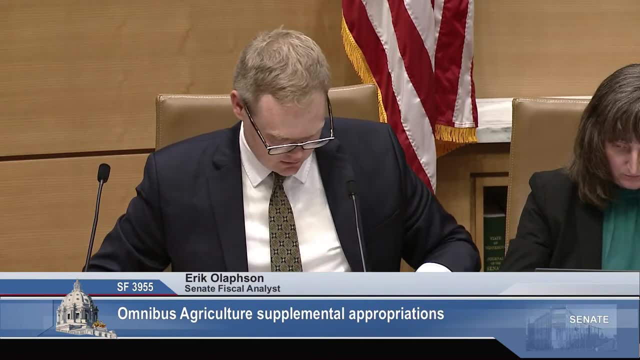 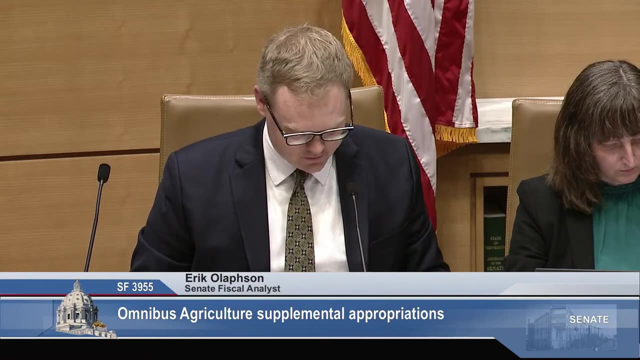 this is that corresponding maintaining current service levels tails reduction of $20,000, reduction in FY26 and FY27 each year. So moving on to page 2, just to summarize all of the Department of Ag, you can see for the 24-25 biennium there's 2.5. a net additional spending from the general fund of $2.545 million in the 24-25 biennium and $2.576 million in the 26-27 biennium, Moving on down to line 55 for the Department of Health. 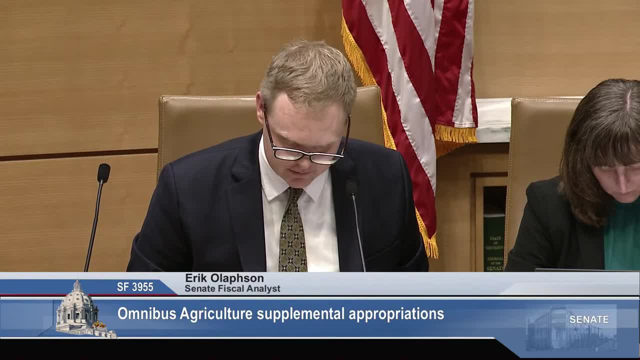 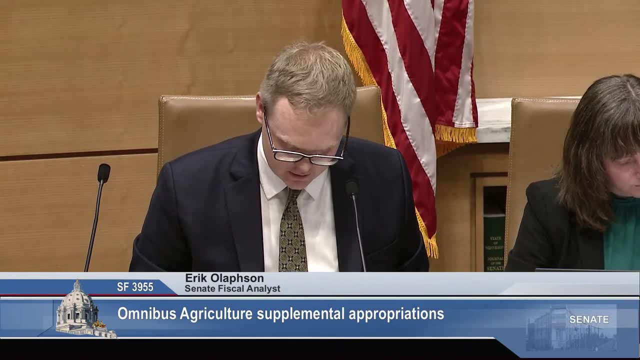 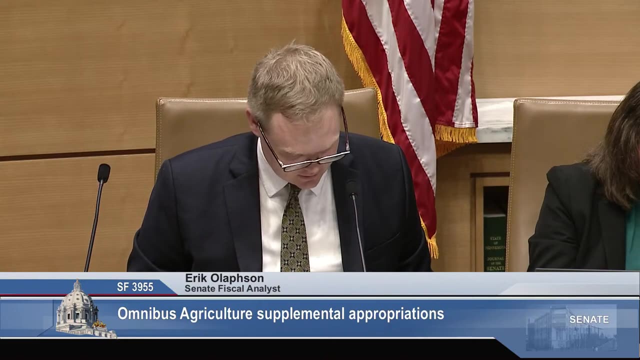 there's additional $2 million, one time in FY25 with extended availability, specifically to address nitrate contamination in private wells in southeastern Minnesota counties, So to so. on line 66 you can see the general fund appropriation that meets our targets of $4.545 million in the 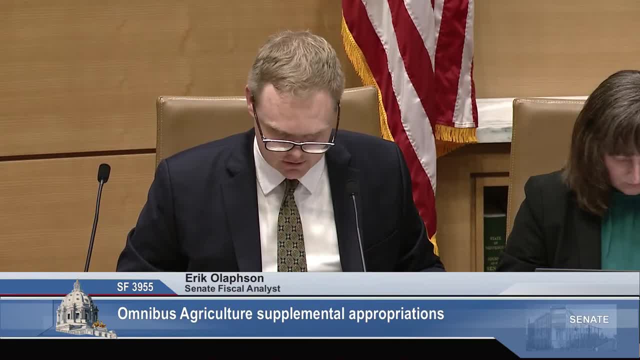 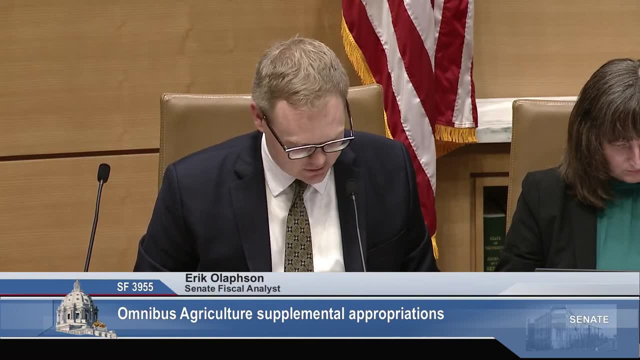 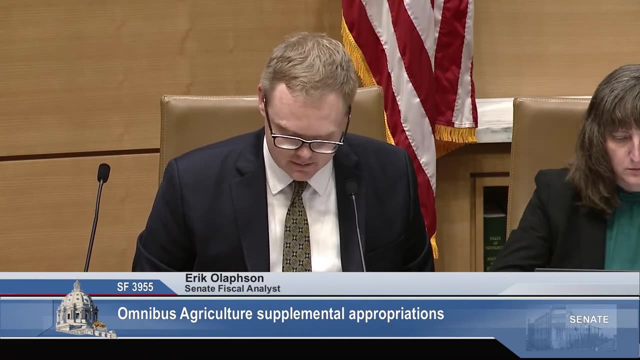 24-25 biennium and $4.576 million in the 26-27 biennium. Just moving on to non-general fund expenditures, there's a typo on this spreadsheet and I will update the spreadsheet for Wednesday's committee. but the amounts for the AFREC 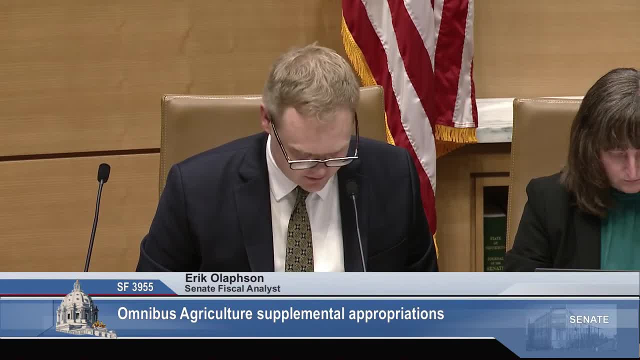 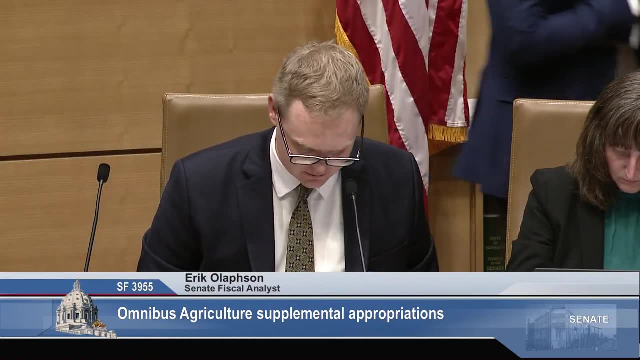 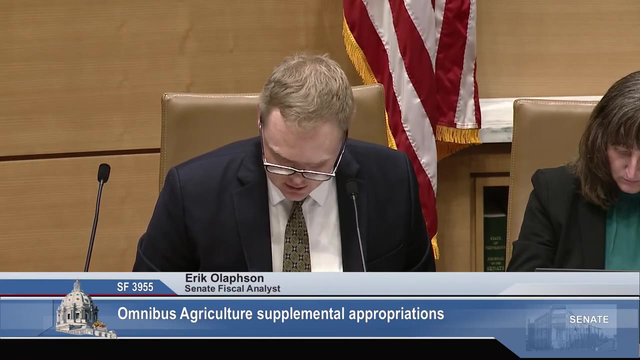 extension on line 74 through the bottom should be $1,270,000 not $1,240,000, so I apologize for that typo and it will be corrected. So for additional expenditures for AFREC it should be $1,270,000. 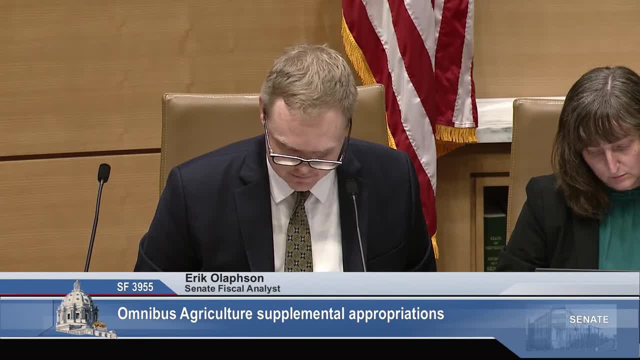 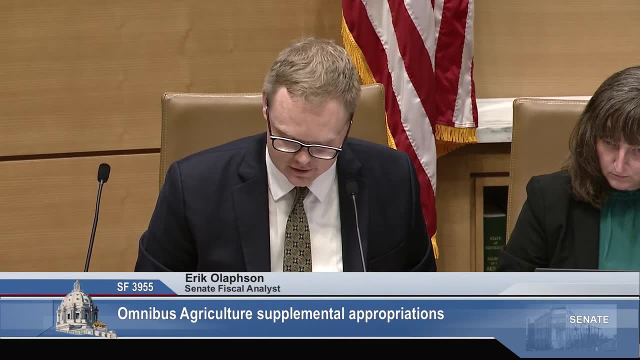 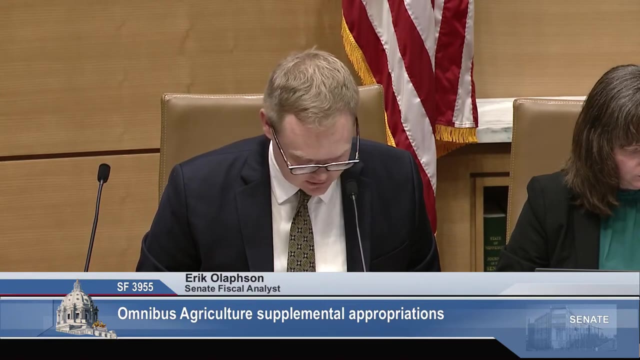 additional from the Ag Fund in the beginning of FY26 with the extension, so for a total of $2,540,000 for the 26-27 biennium And then moving on down to line 80, again it should be $1,270,000. 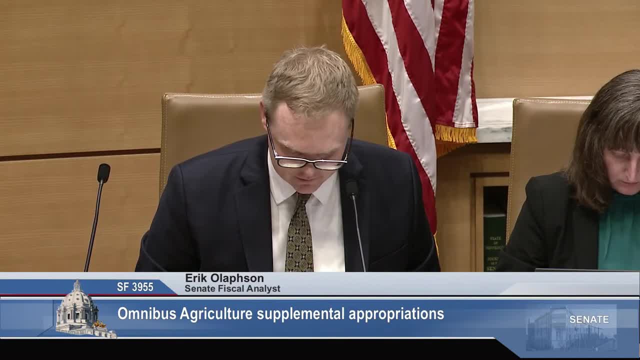 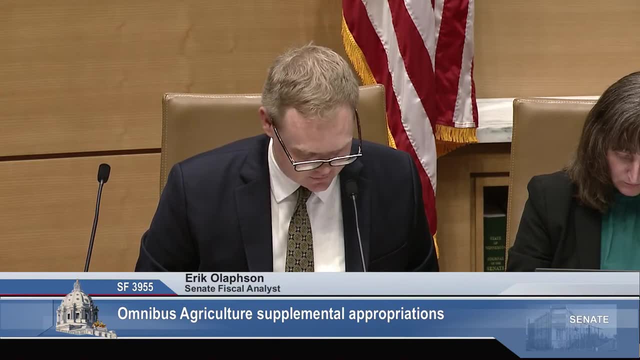 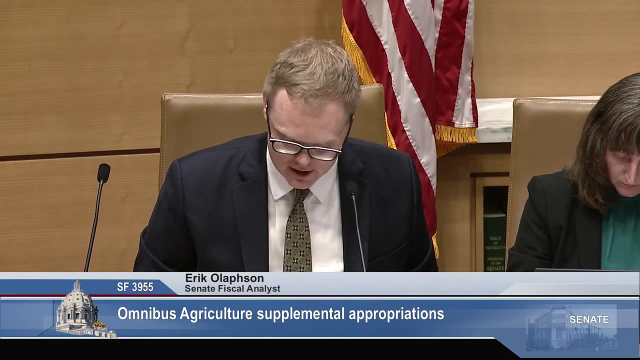 for the additional revenue for AFREC beginning in FY25 and ongoing, So it should be $1,270,000 of net savings on line 83 in the 24-25 biennium and then the expenditures and revenues for the AFREC extension cancel out. 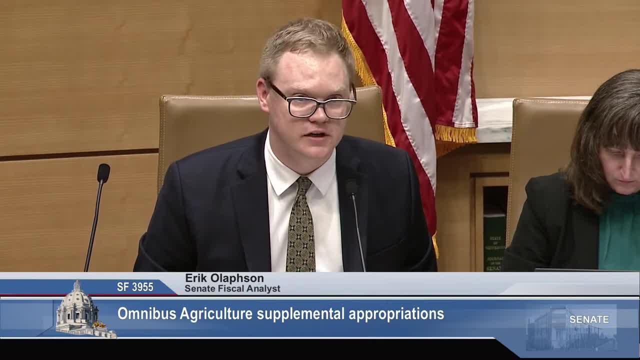 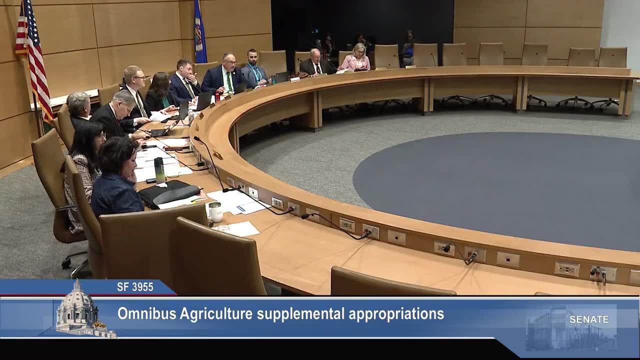 in the 26-27 biennium And with that I would be happy to answer any questions. Thank you, Mr Olofsson. and while we are doing discussion and amendments on Wednesday, anybody members have any specific questions? on the part we just heard. 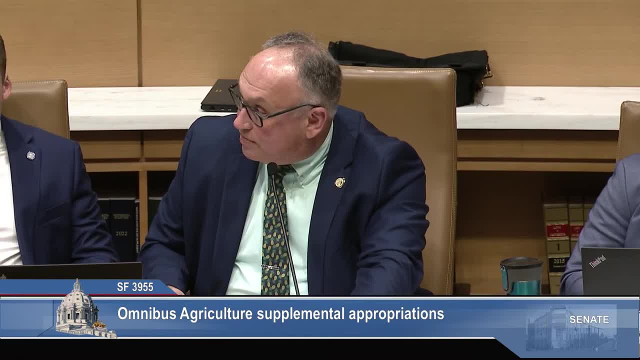 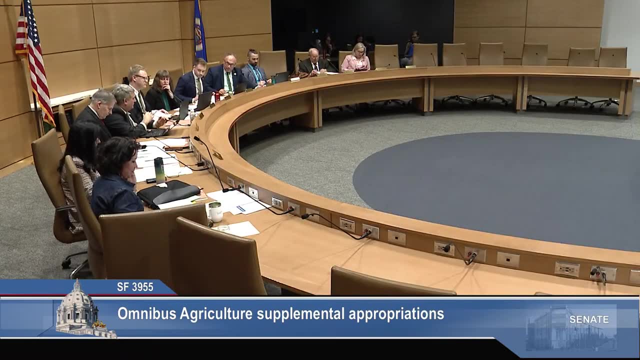 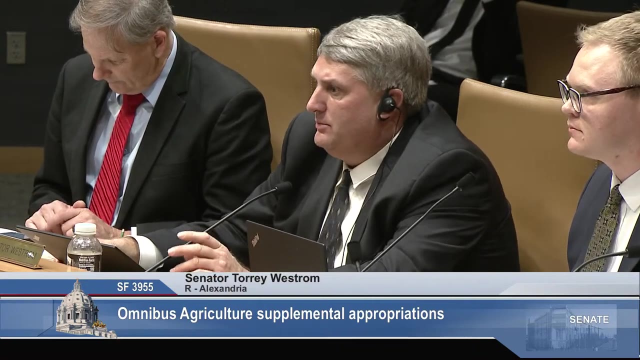 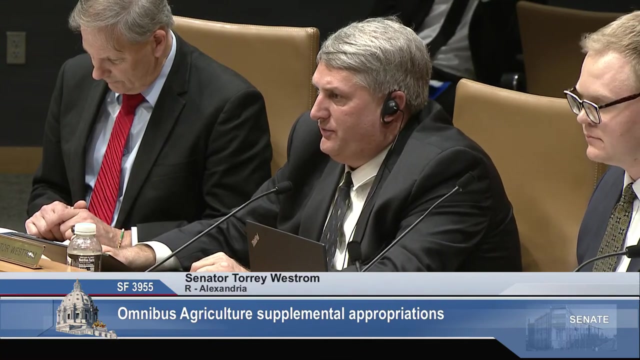 we can certainly entertain those now And if not, we will move on to Ms Painter, Senator Westrom, Mr Chair, the expenditure- probably you, Senator Putnam, the expenditure on the RO systems. one of the testifiers talked about $2,600,000. 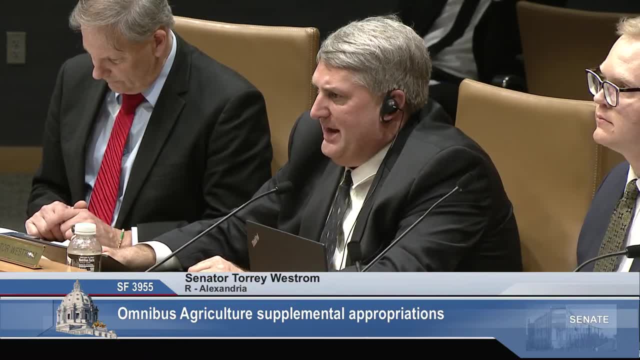 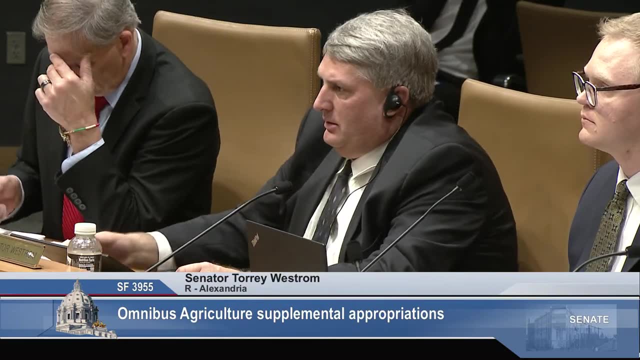 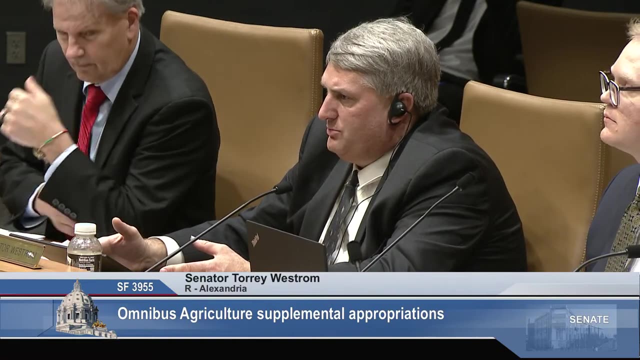 are they all going to be a match, so each applicant would put up some money and it seems like $2,600,000 is higher price than most RO systems out there. are these special, unique? do they do other things that other RO systems don' t do? can you talk about that? 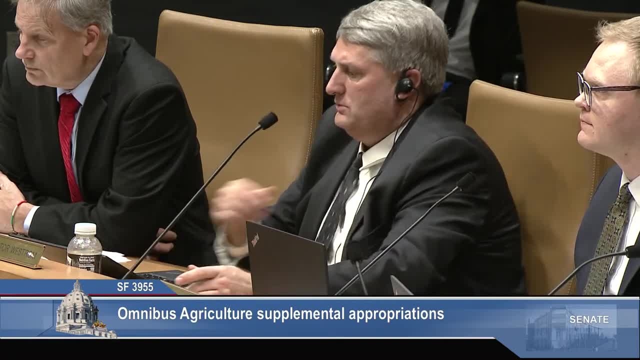 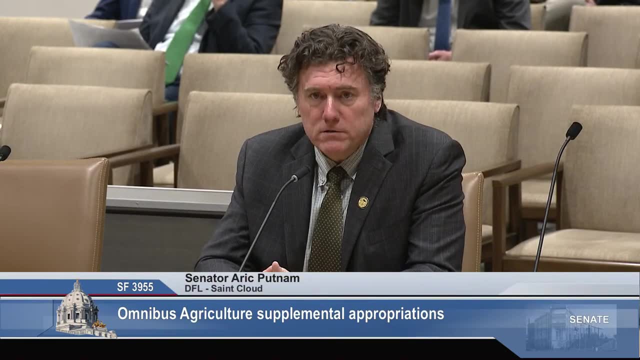 just a little bit more, or one of the testifiers? Senator Putnam, Mr Chair, Senator Westrom, it' s an excellent question. I' ll sort of explain the best of my ability, which is meager, so there' s a good chance that we might have to. 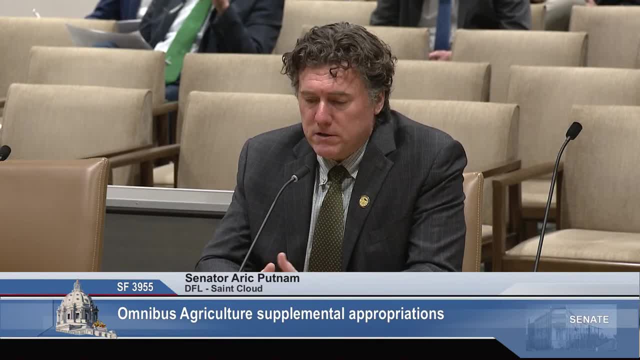 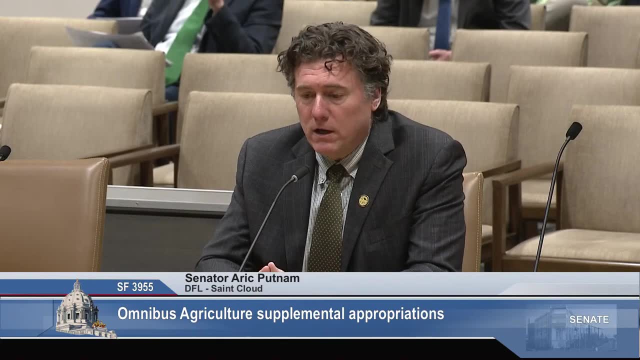 ask someone else to come up here and explain a little bit better, but my understanding is one: within that $2,600 is a year's worth of maintenance and upkeep, so that might be a part of that additional expense also that hopefully the program will be tiered. 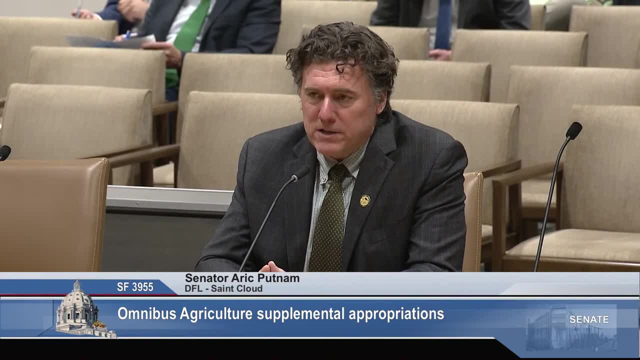 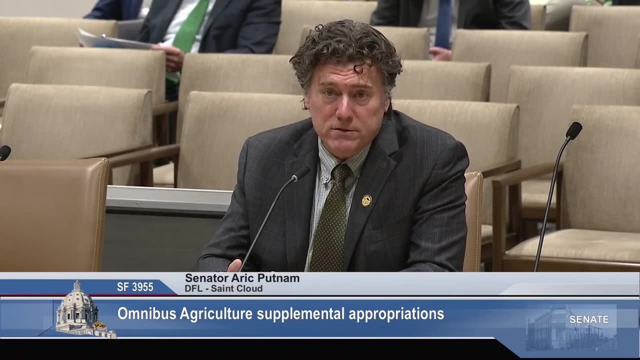 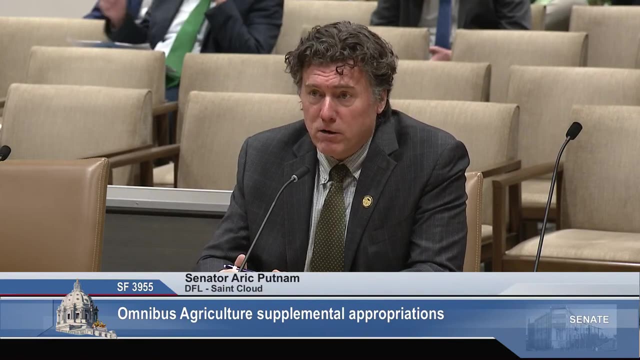 to a certain extent, in that it will be means tested and that there will be matching for folks at a certain level of income and different matching for folks at different levels of income. that' s my understanding, but perhaps our friends from MDA, maybe Ms Medina, would like to explain that and correct. 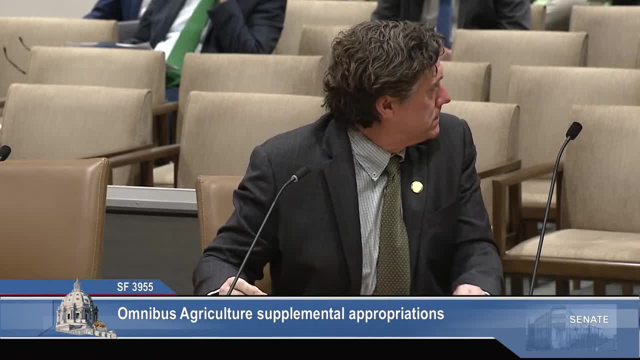 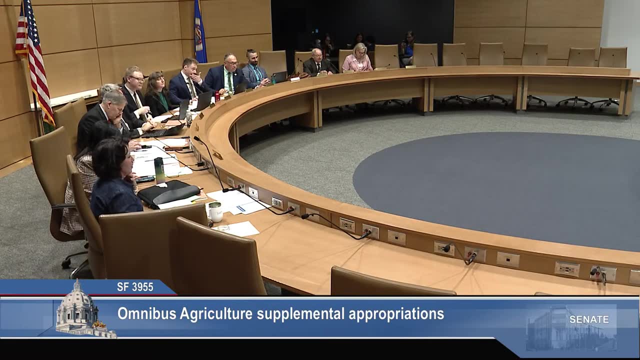 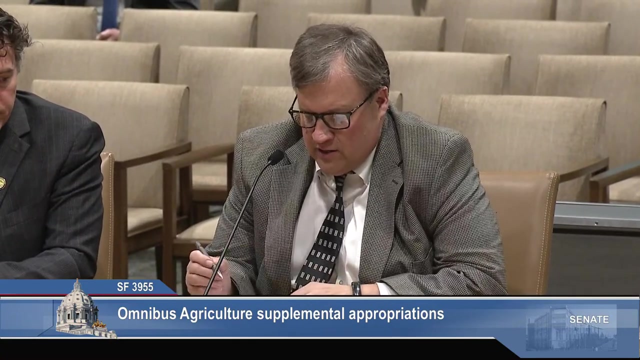 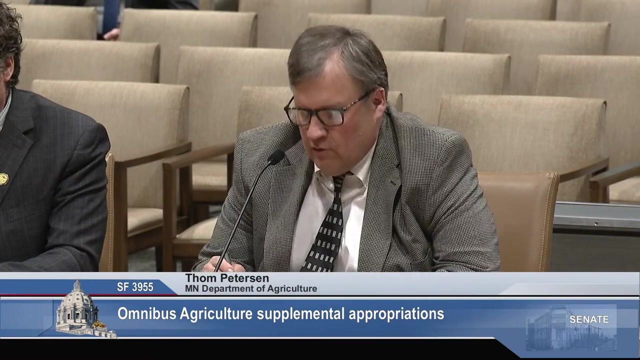 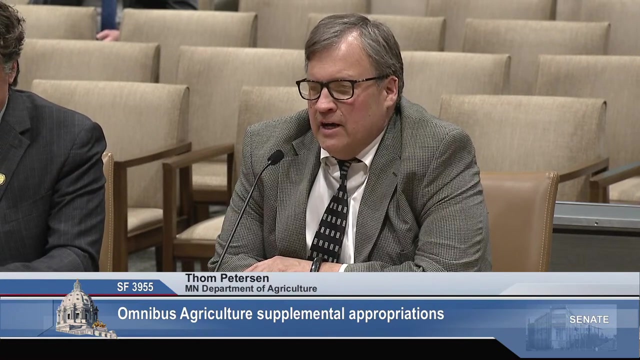 all the stuff that I just said. Sure, absolutely, Commissioner Peters, Mr Chair and Senator Westrom, just looking at the language too, and everything, we would look at this. I think, in looking at this kind of a new thing too, and not knowing exactly what the need is going to be, 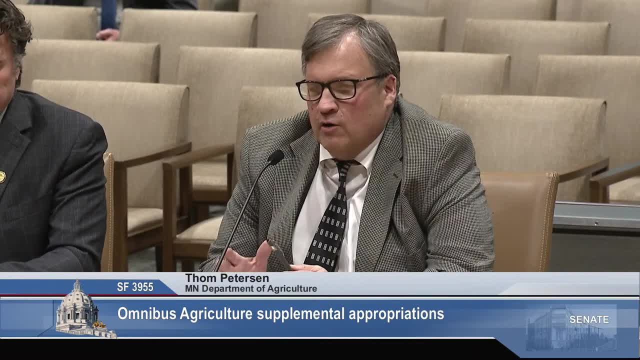 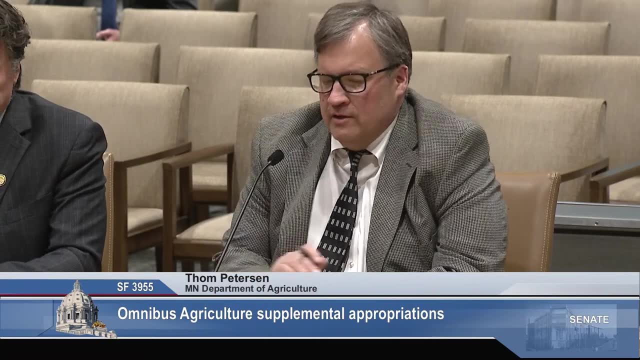 and how this is going to go. we' ll continue to look at this. right now we' re putting out a pilot program ourselves in the department. we' re just kind of formulating that with a half a million dollars that we put together within our own budget for this year. 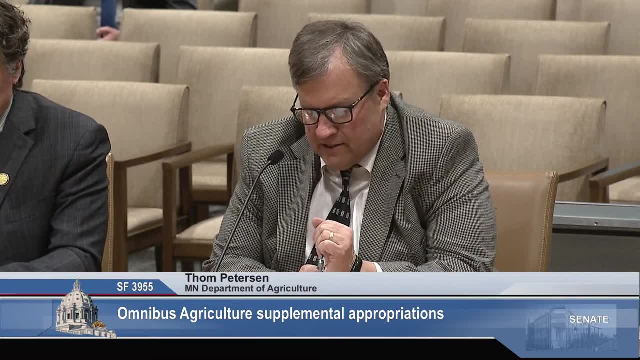 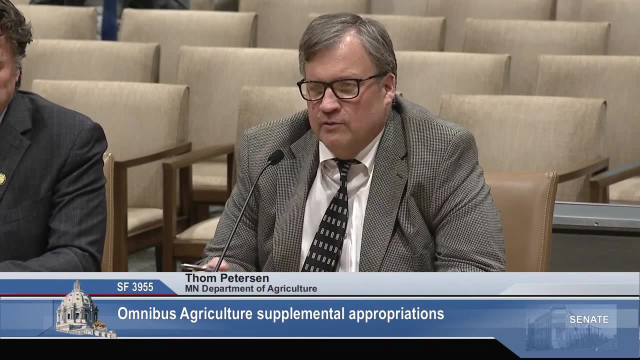 and so this would go on top of that. so we' re looking at, as the bill says, up to 300%. we could do up to 100%, but at a lower level. we would probably do a cost share or something on applicants like that, if that makes sense. 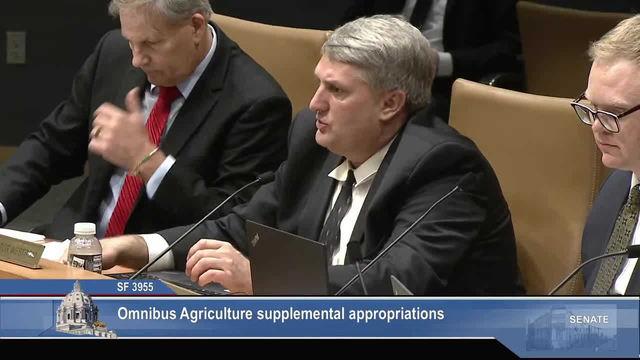 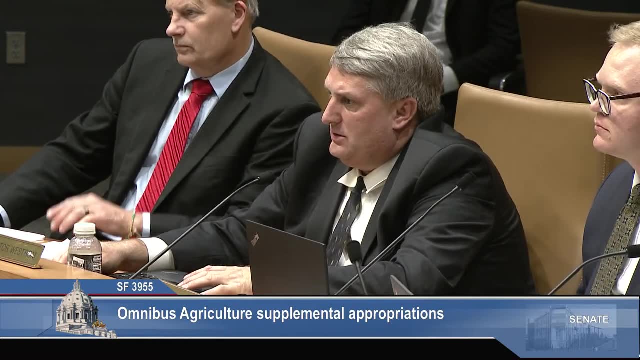 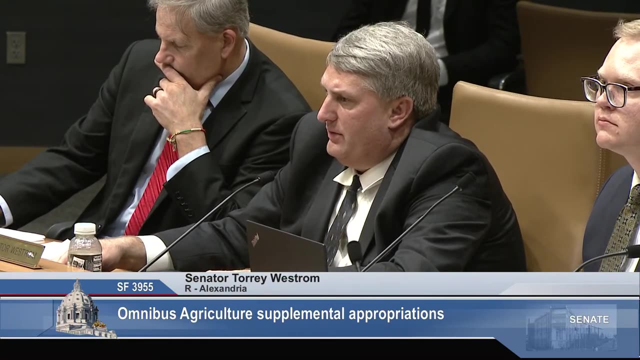 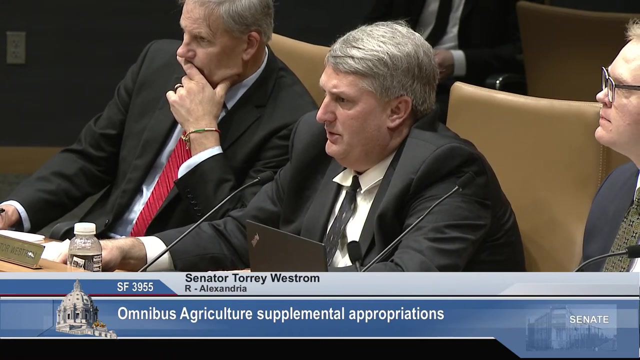 Senator Westrom, Mr Chair, Commissioner Peterson, do you anticipate getting a quantity contract or would they just be reimbursed by any local RO dealer, wherever the consumer buys them, or would there be kind of a set fee? do you anticipate and do these systems have anything more? 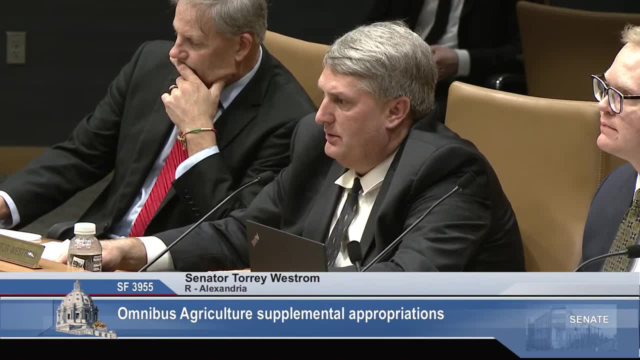 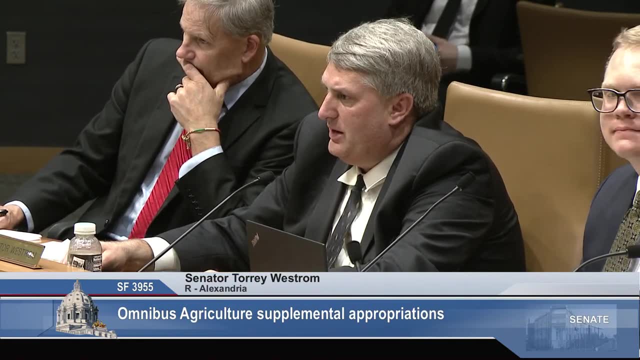 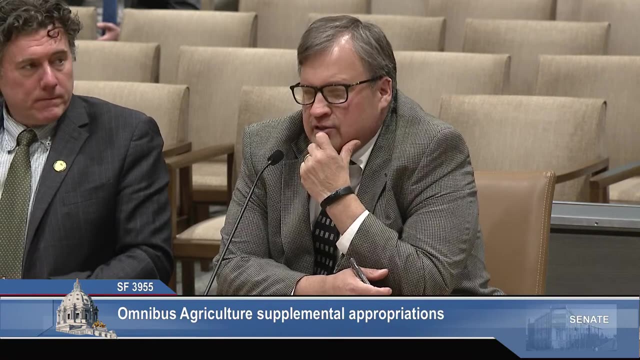 unique than what an RO you know, Culligan or I don' t know some of the other brands that are out there. do they all do the same kind of effect? Commissioner Peterson, Mr Chair, and you know, 2600 RO systems vary- I myself, Mr Chair and Senator Westrom. 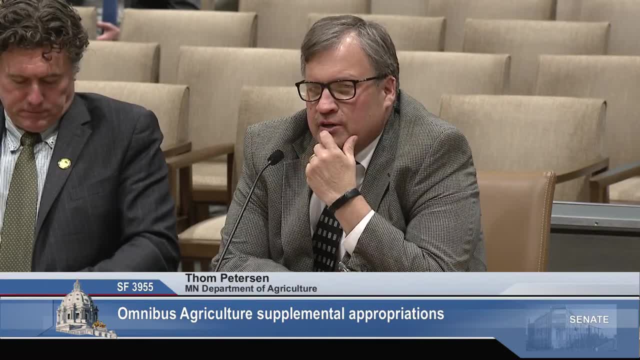 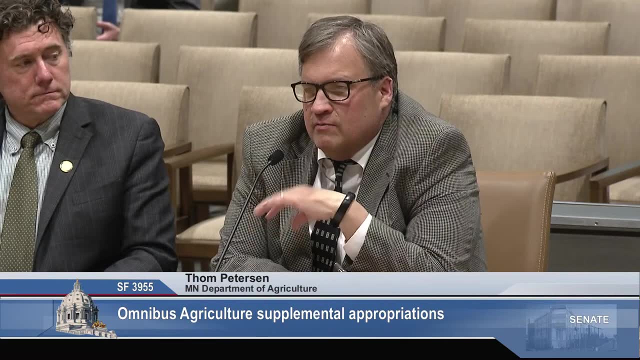 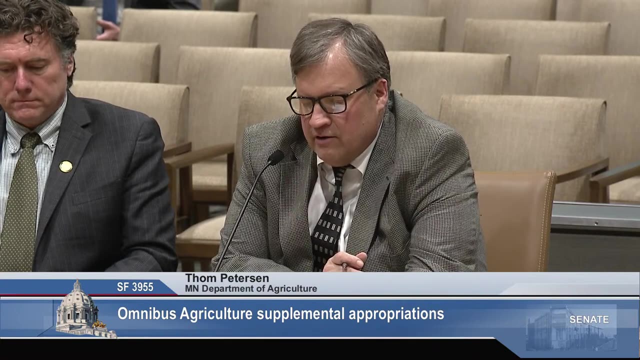 have met with the well drillers actually do also put in well, most of them do RO systems- and met with them and they said, as you' re kind of saying, there' s different varieties and things like that, but they really do. by the way, you know, they say we' ll take care of the. 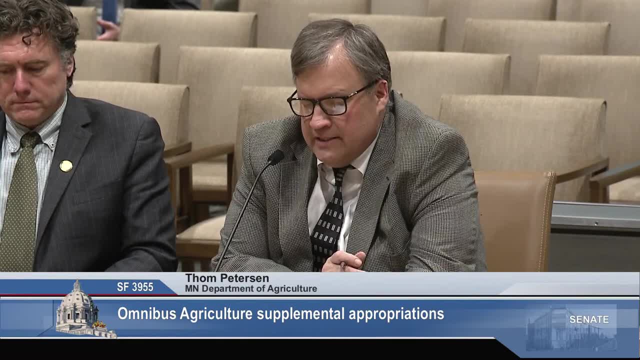 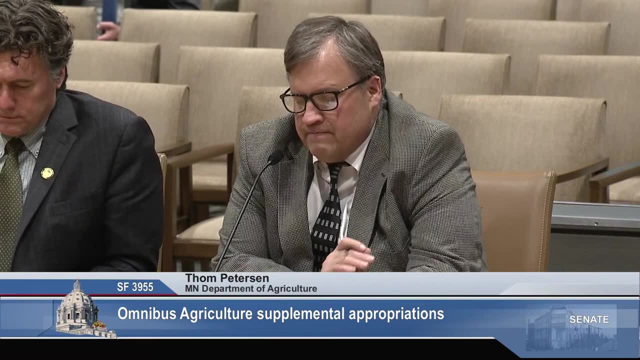 issue too as well. but I also have Ms Wagner here and she can provide. she' s been working on this issue and she can provide more background on the RO systems. A little bit, Mr Chair and Mr Commissioner, that would be helpful. I mean, I just 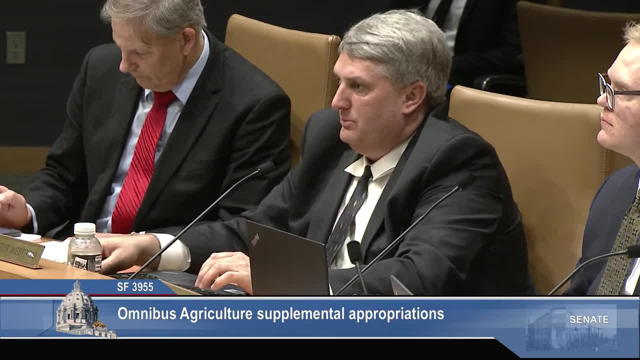 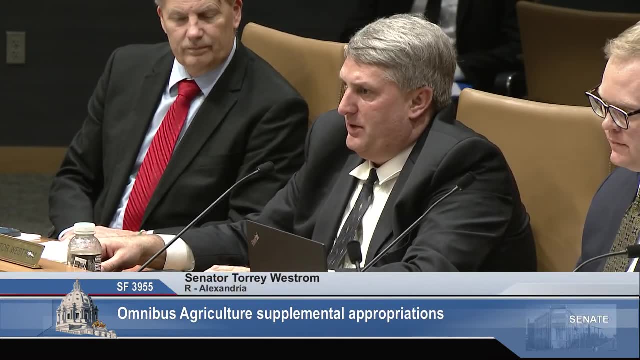 I assume you' re that' s kind of what you' re digging into, but it would be helpful to know. I want to make sure we' re getting the best bang for the buck and spreading it to the most farms or property owners affected as we can. if we' re doing this, 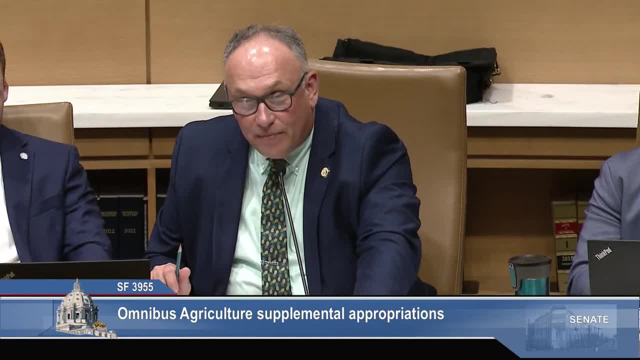 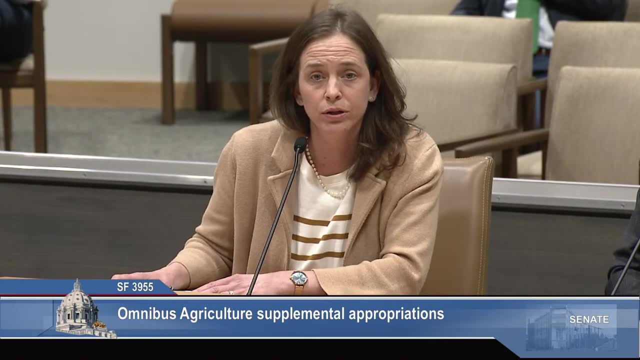 Ms Wagner, do you want to just state your full name and then you can go? Mr Chair and members of the committee. my name is Margaret Wagner and I' m the manager of the fertilizer and on point section at the Minnesota Department of Agriculture. Senator Westrom, to answer your questions. 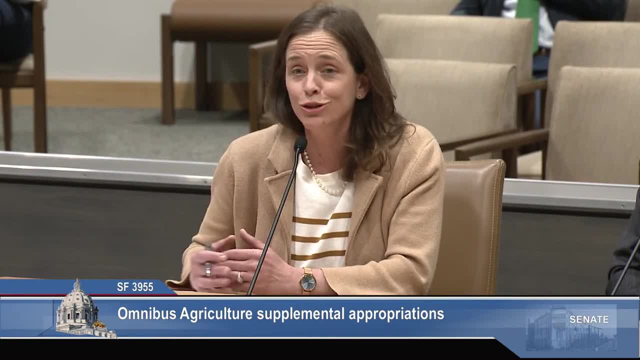 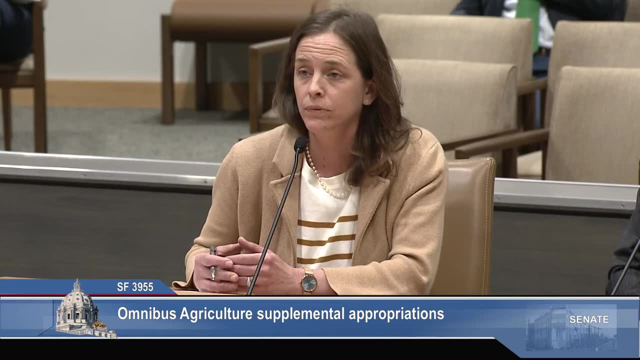 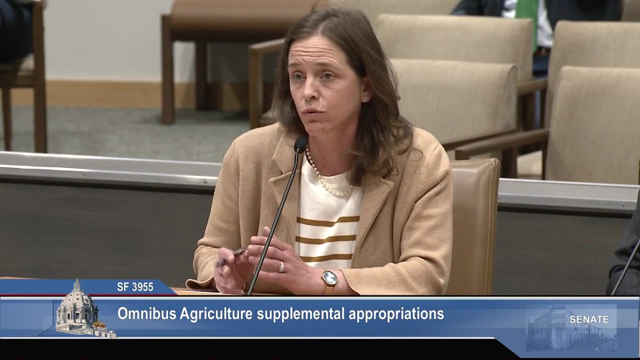 there is some variability in the price, but we' re using information through pilot programs that have occurred in southeast Minnesota through the tap in initiative, so similarly working through a local partner like Olmstead County to help administer this program. so their experience is generally $2500 for. 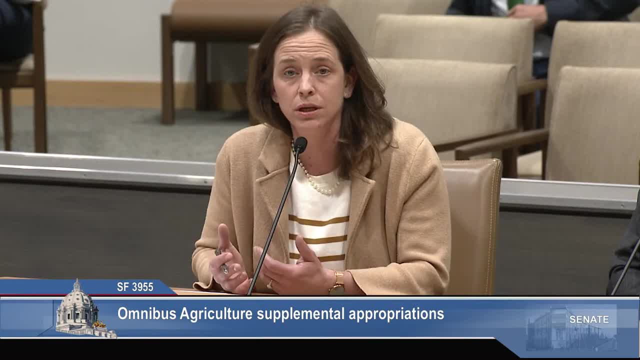 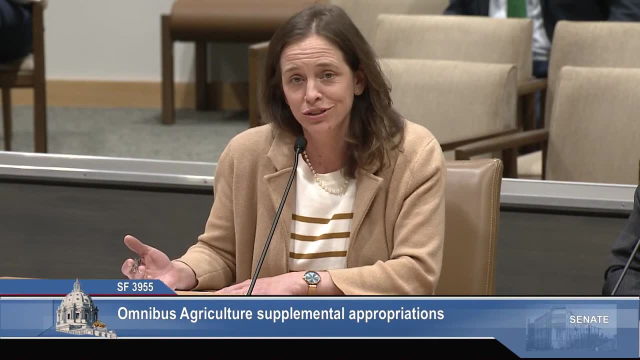 those systems with installation, then, as mentioned, a year of maintenance on top of that. so what we know is, if the cost comes in lower than that, then we would be able to buy additional systems through the program, but this is our initial estimate based on purchasing and installing these systems. 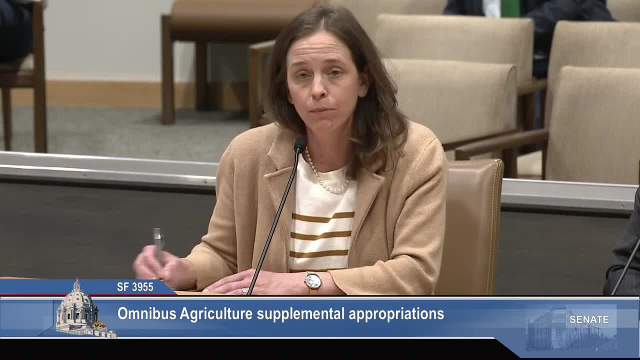 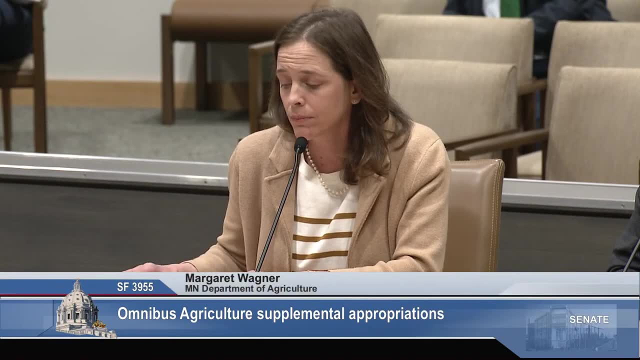 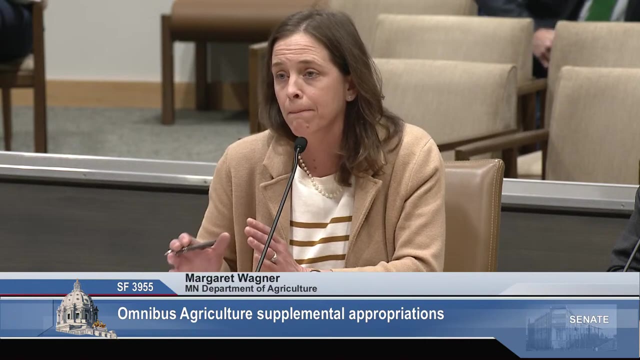 in that general region and right now we' ve identified 100% caution cost share for demonstrated economic needs. so those, those households that fit that criteria and from there we would scale back that cost share, looking at some type of match. so it may be 50- 50. 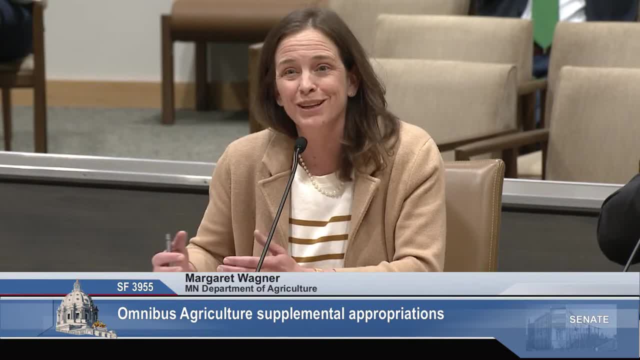 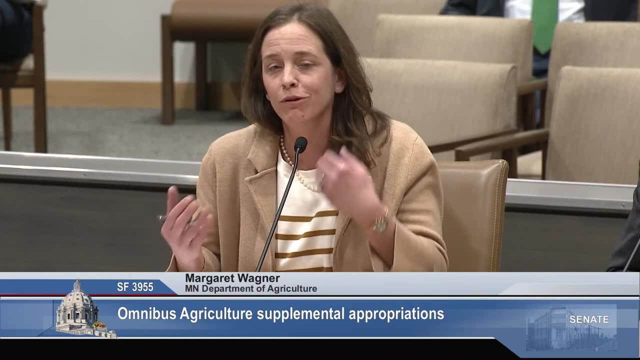 and those are the types of details we' re working out and as we put together those estimates, we kind of scale we can obviously purchase more and install more systems if we are providing less of the up front cost and then, as far as batching, we will again want to. 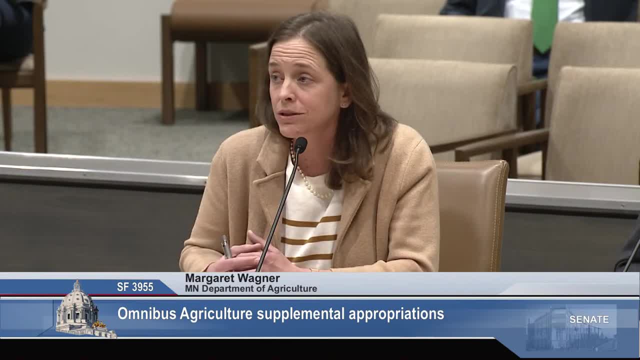 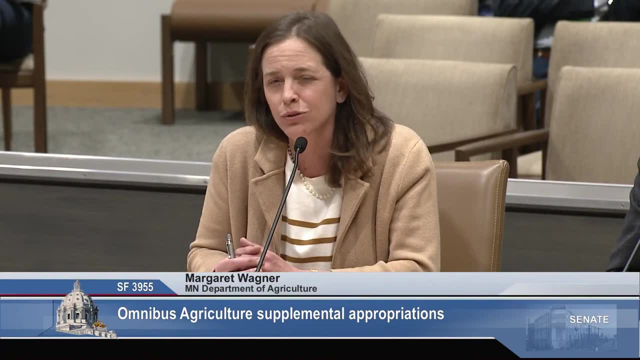 partner with local through a joint powers agreement or another mechanism with a local partner to help deliver this and we will be working then through professional plumbers for the installation. so yeah, I think there are opportunities to have those discussions and think about installing multiple systems in this geographic area. 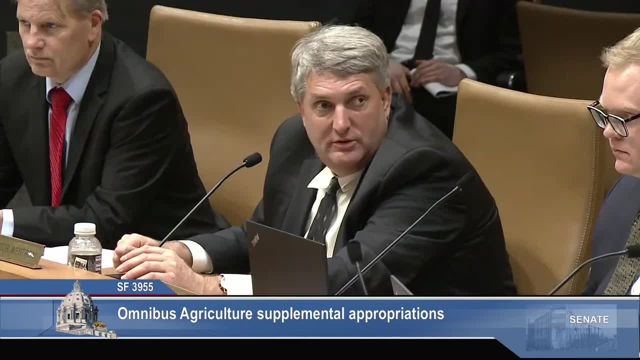 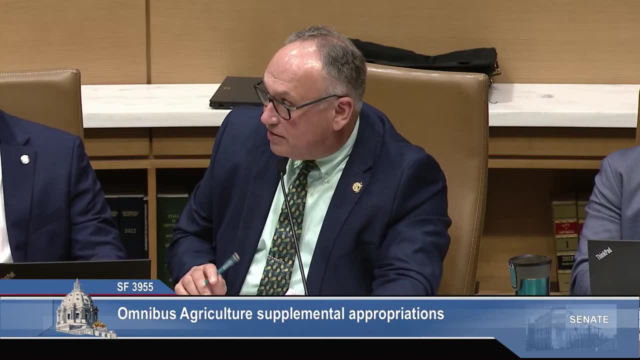 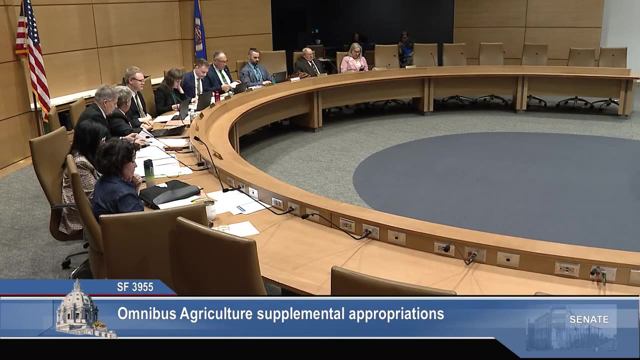 Senator Westrom. Thank you, Mr Chair and Ms Wagner. thank you, that' s all for now. Okay, seeing no other questions, we will move on to Ms Painter for the technical walk through. Mr Chair and members, I will just quickly walk you through articles 2 and 3. 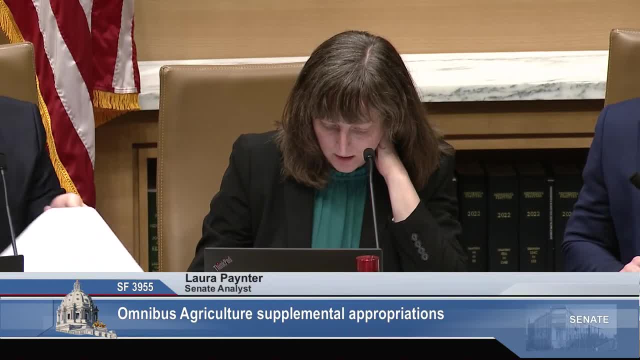 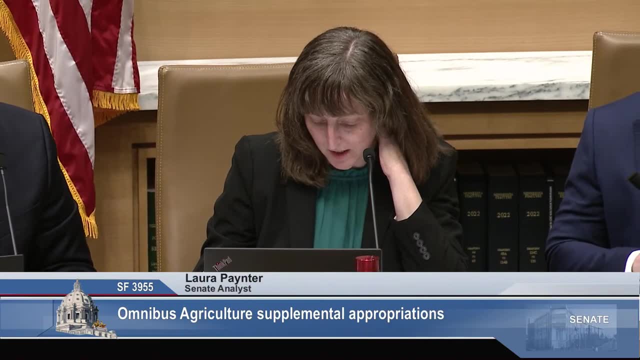 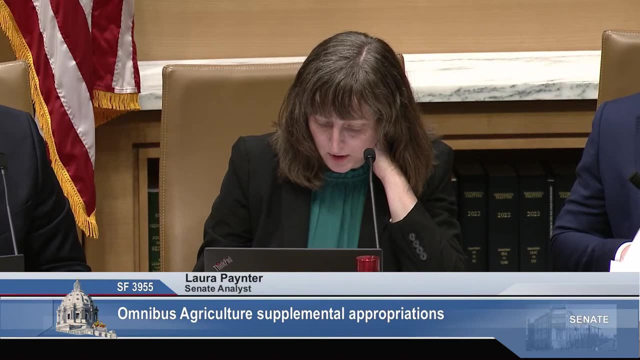 Article 2 is agriculture policy. Section 1 amends the beginning farmer equipment and infrastructure grant program to give preference to farmers experiencing limited land access. this is from Senator Putnam, Senate file 5049. Section 2 expands eligibility for sustainable agriculture demonstration grants to add certain organizations. 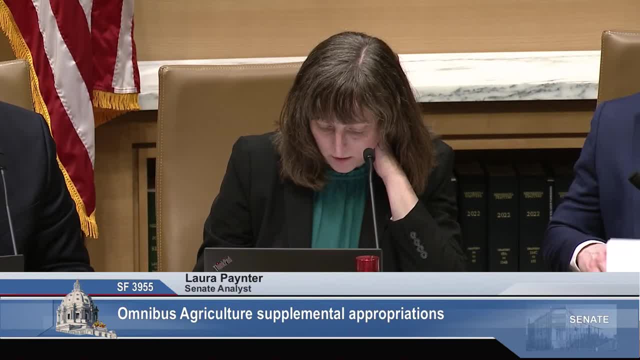 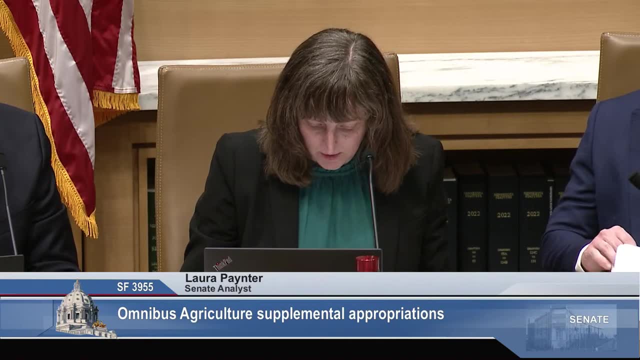 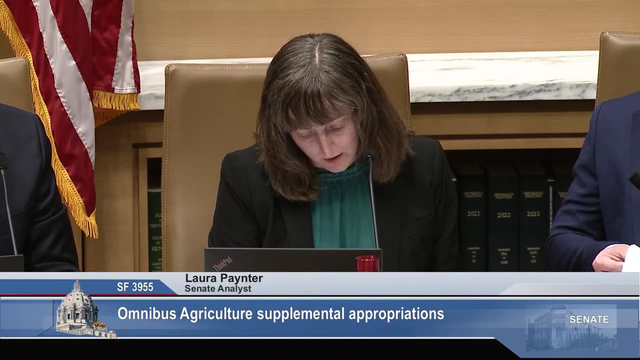 this is from Senate file 5125, Senator Kunesh's bill. Section 3 amends the farm down payment assistance grant definitions. the definition of eligible farmer would add a requirement that a farmer has at least three years of experience farming. and in this section there is also. 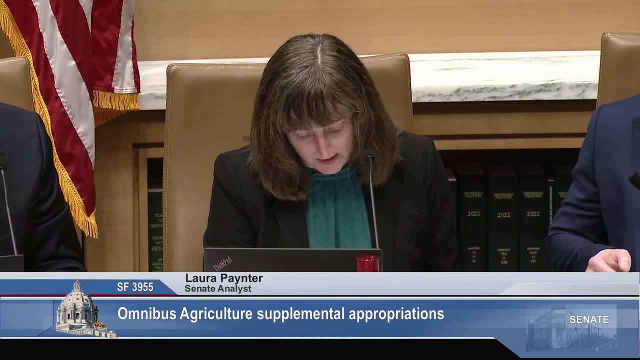 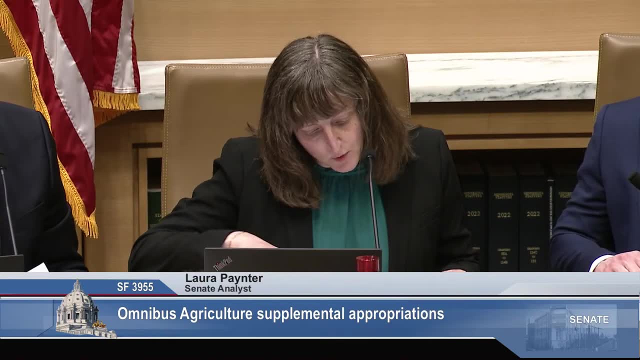 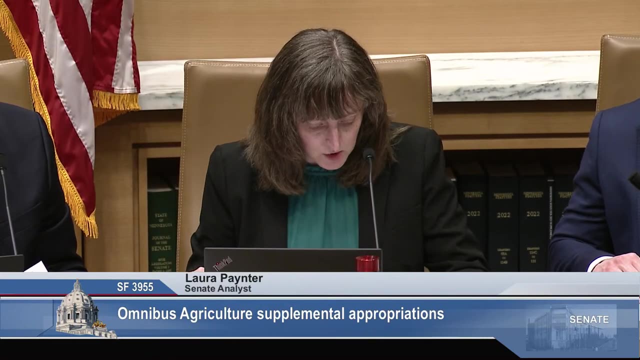 definitions added for incubator farm and limited land access. this is all from Senate file 5049 from Senator Putnam. Section 4 amends the reporting requirements for the farm down payment assistance grant. again that's from Senate file 5049. Sections 5 through 8 are the 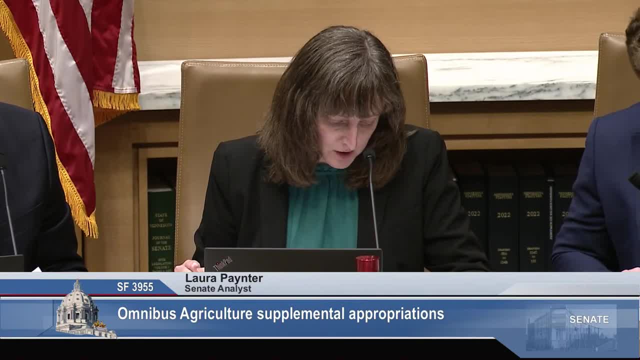 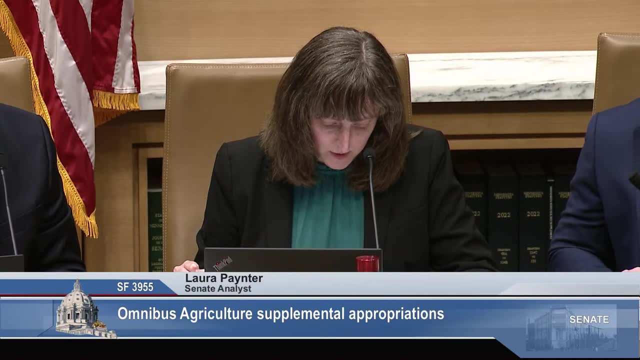 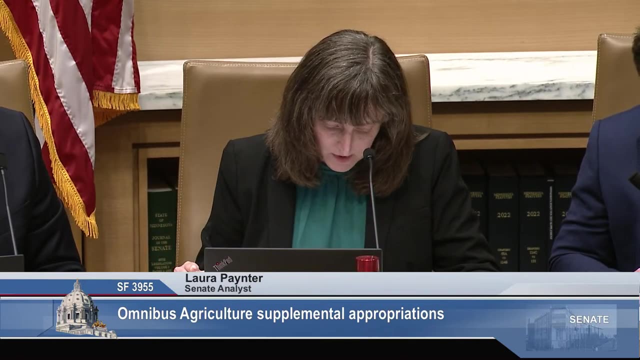 extension of the Minnesota agricultural fertilizer research and education council until June 30, 2035. this is from Senate file 3719 from Senator Putnam. Section 9 removes some obsolete language. this is from Senator Gustafson, Senate file 4187. Section 10 extends the Minnesota. 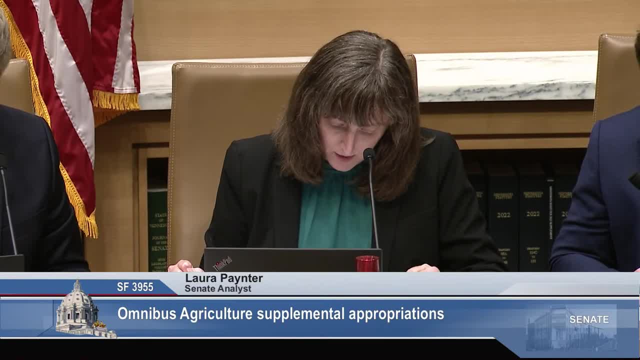 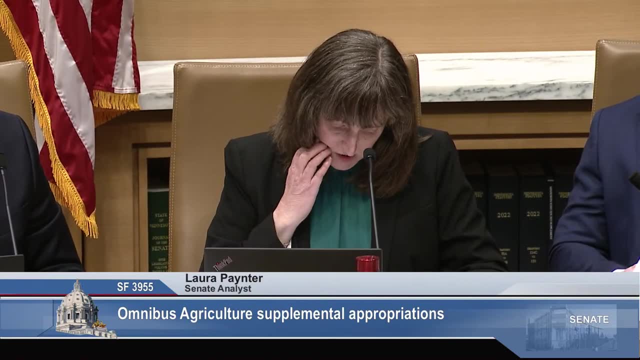 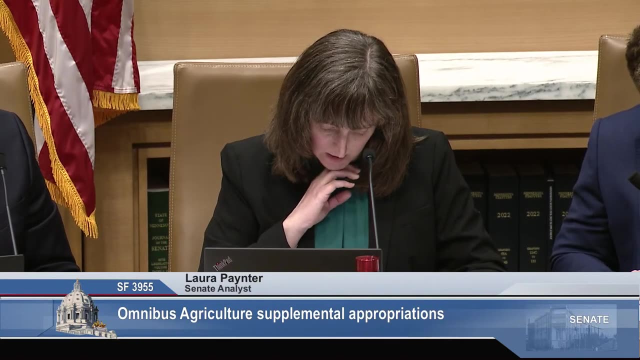 organic advisory task force to 2034. this is from Senate file 5365 from Senator Putnam. Section 11 makes some changes to the dairy development and profitability enhancement program to allow more flexibility in the program delivery. this is also from Senate file 5365 from Senator Putnam. 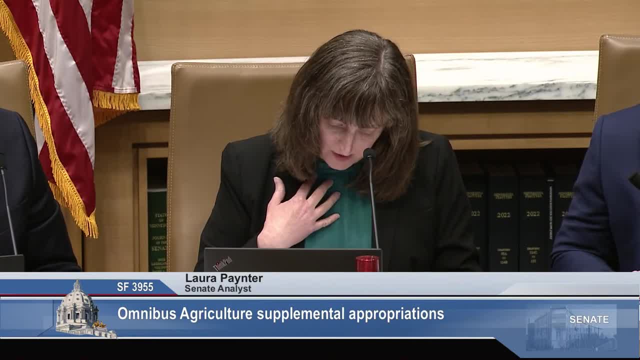 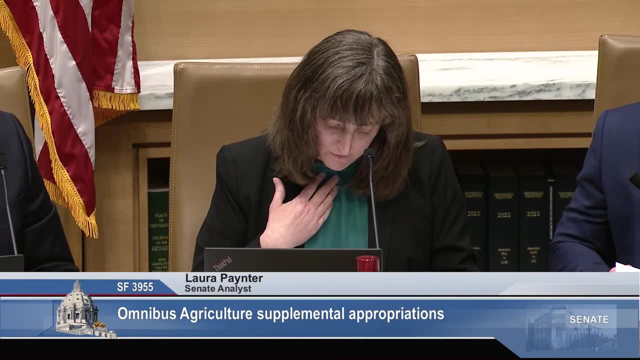 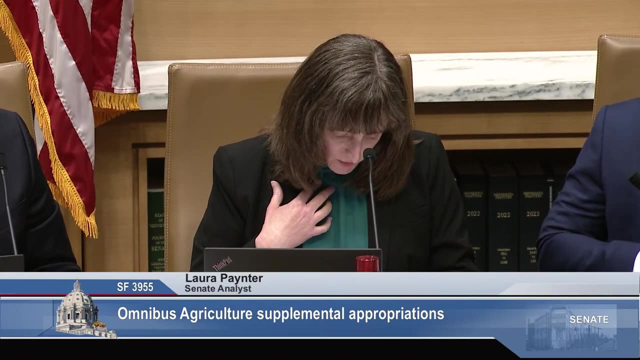 Section 12 adds a reference to the limited land access definition in the beginning of farmer tax credit definition. this is from Senate file 5365 and also Senate file 5049, both of them from Senator Putnam. Sections 13 through 15 makes some changes to the beginning. 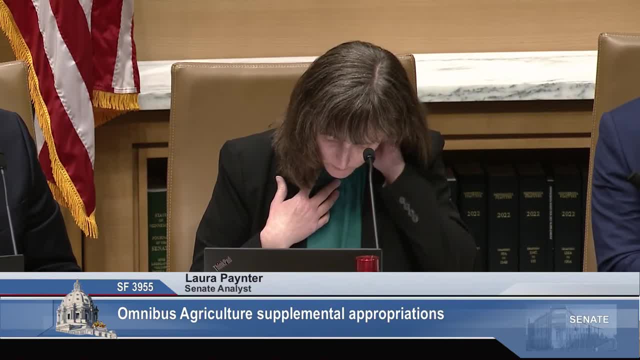 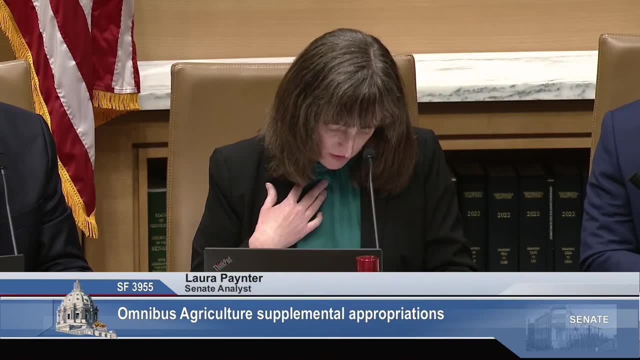 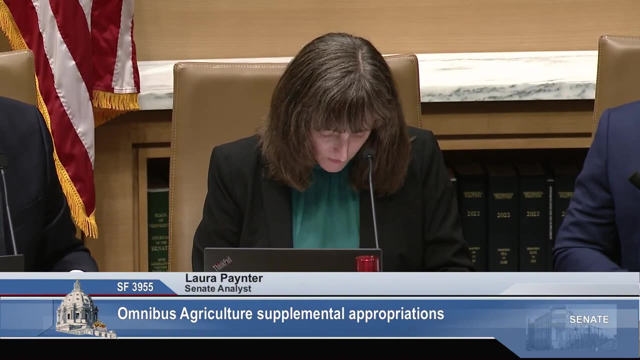 farmer tax credit program. these are all from Senate file 5049. Section 16 amends the disaster recovery loans to allow them to be used to purchase feed during a drought. Section 17 repeals the beverage inspection account. this is from Senator Gustafson, Senate file 4187. 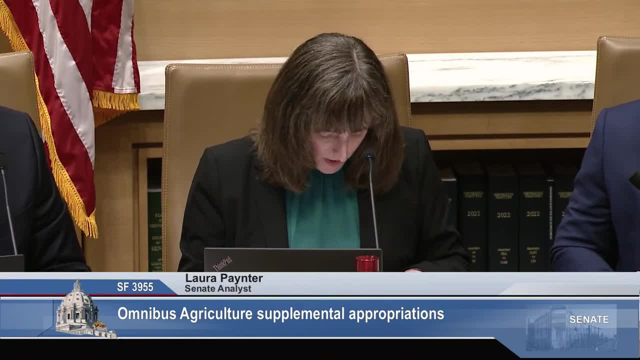 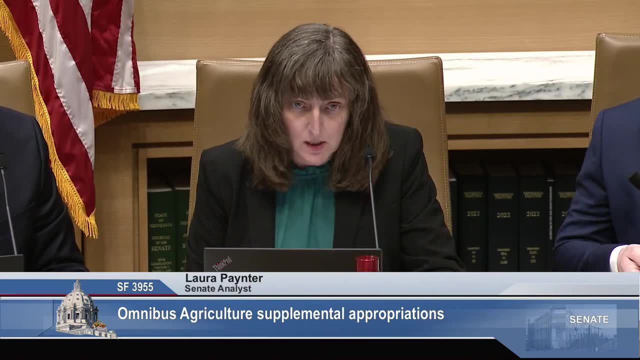 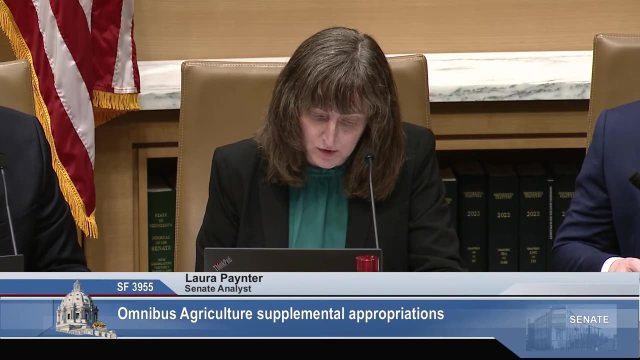 and then Article 3 relates to broadband, and both of these sections are from Senate file 5366, which we heard today from Senator Putnam. Section 1 allows the Commissioner to transfer up to $5 million between three different programs: Section 17 and Section 2. 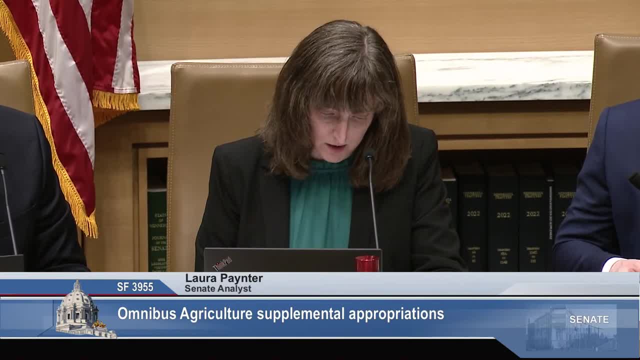 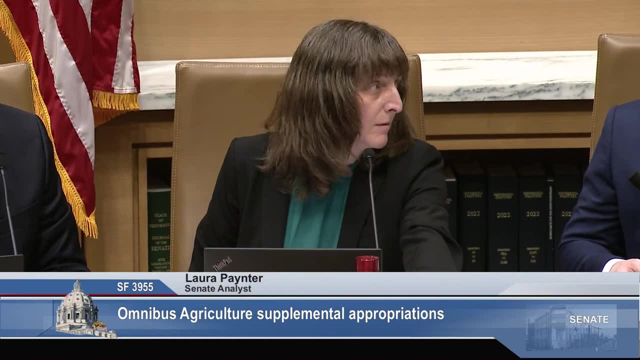 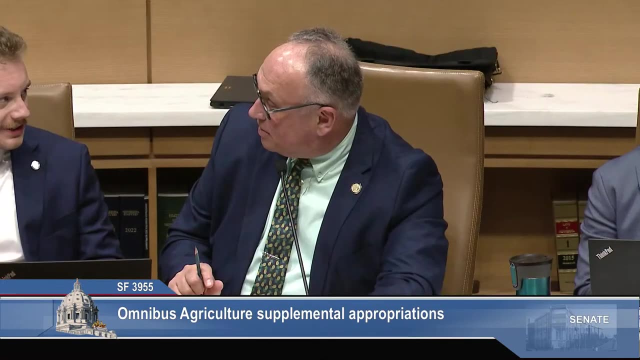 requires the Commissioner to apply for federal grants and use the money for the purposes in the Minnesota digital opportunity plan. Thank you, Ms Painter, and with that we should have some testifiers who would like to, if there are any other questions for Ms Painter? Seeing none. 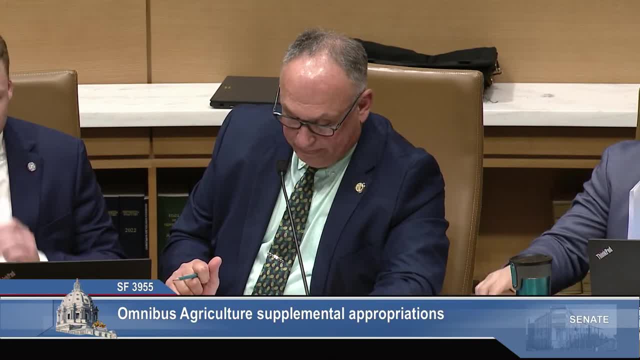 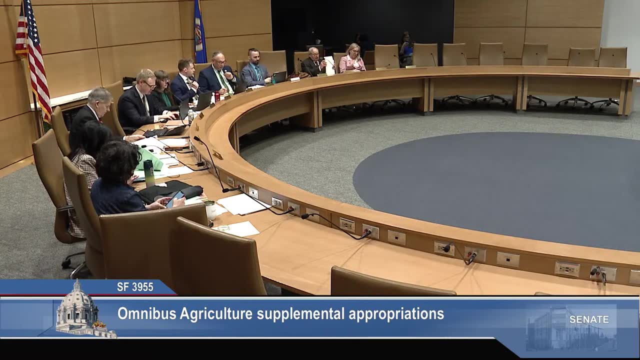 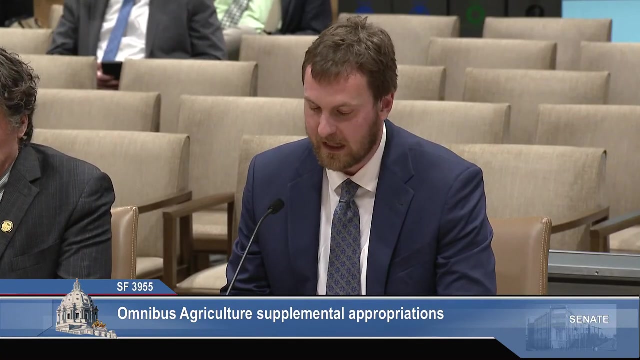 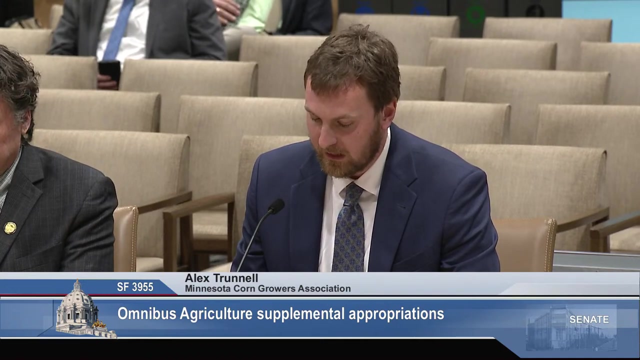 then we will go to. first on my list is Alex Tranel. Please do the many first graceful, And you may state your name to begin when you are ready. Mr Chair, members of the Committee, my name is Alex Tranel. I serve as the Public Policy Manager at the Minnesota. 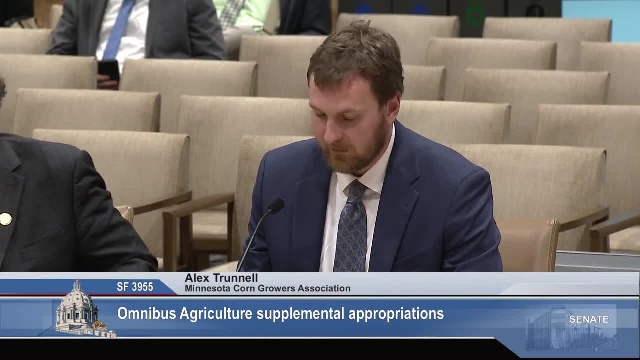 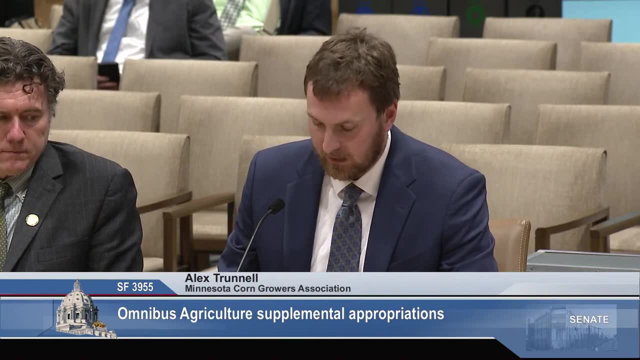 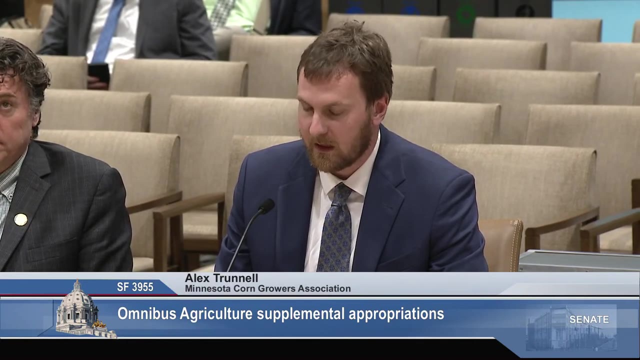 for SF 3955 forward and addressing specific needs in response to the EPA petition related to nitrates in southeast Minnesota. MCGA is committed to addressing nitrogen challenges in southeast and other vulnerable groundwater areas through partnerships, research policy and best management. 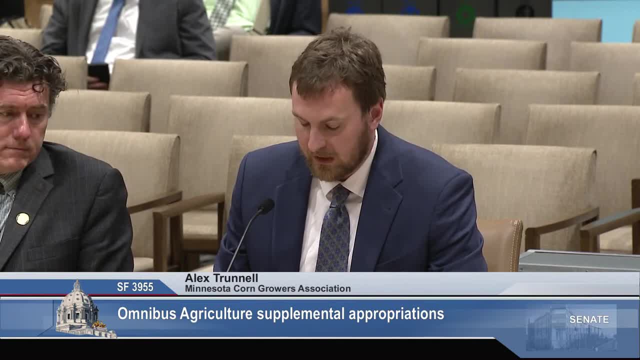 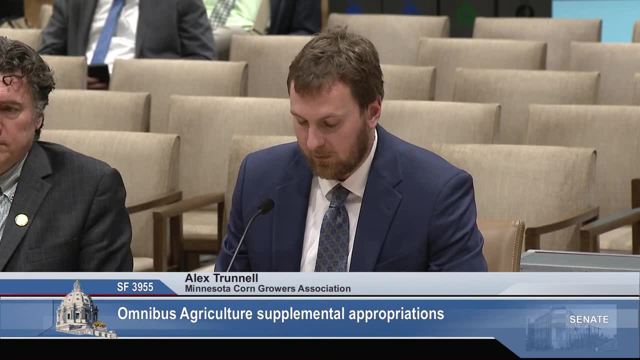 practice adoption. We support the funding to MDA to help provide clean drinking water to those with private wells that have tested for high levels of nitrates. We also want to thank the committee for looking at existing programs to address nitrates in southeast, where the karst 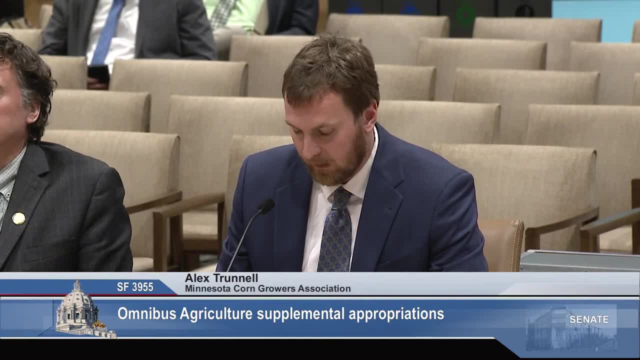 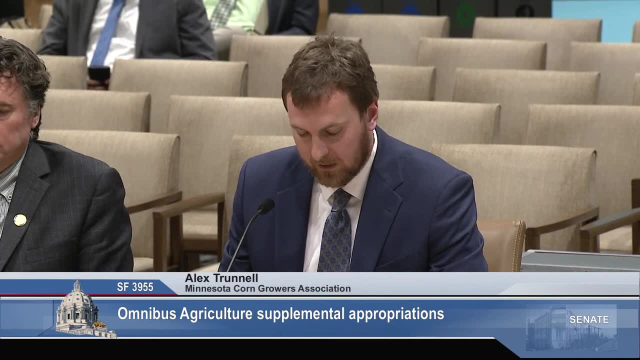 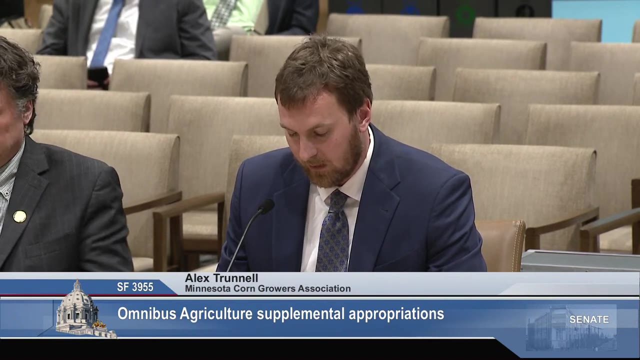 geology is particularly susceptible to nitrate contamination. The Soil Health Financial Assistance Program has strong support by Minnesota farmers and that is demonstrated by the overwhelming number of applications that the program has received the last two years, with demand far outpacing available funds, and has shown how interested Minnesota farmers are in exploring. 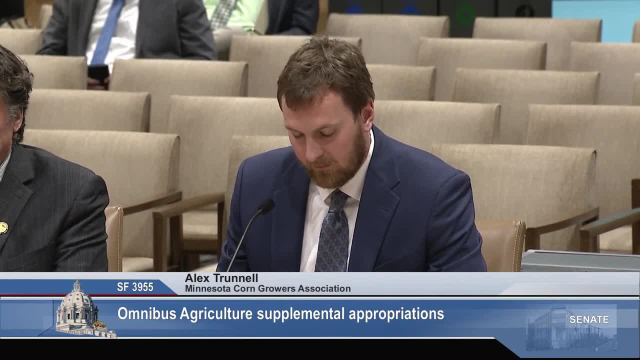 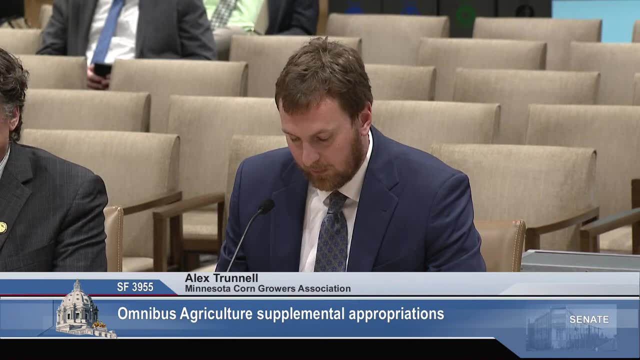 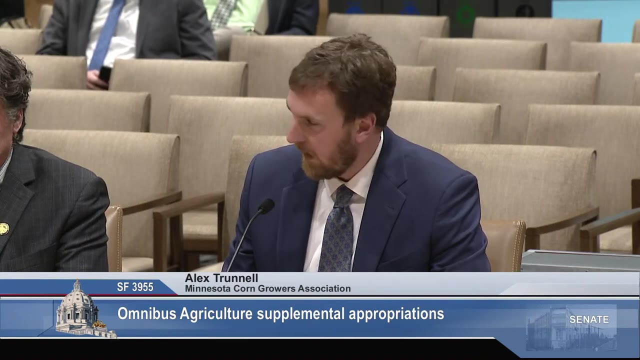 and implementing practices to improve soil health. The $500,000 appropriation targeted at southeast Minnesota and the flexibility of the types of projects that are eligible to apply will allow the department to award grants to farmers to implement practices that will improve soil and water and begin to address nitrate levels in drinking water. Finally, we'd also like to express 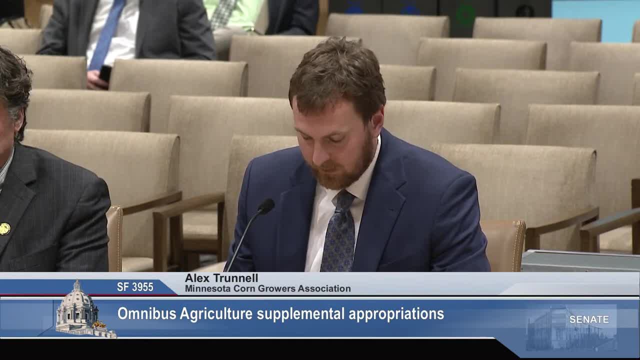 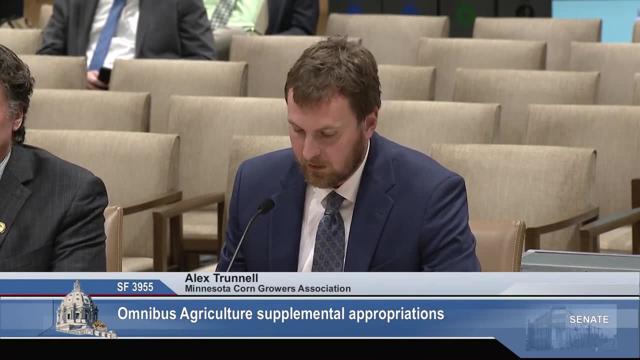 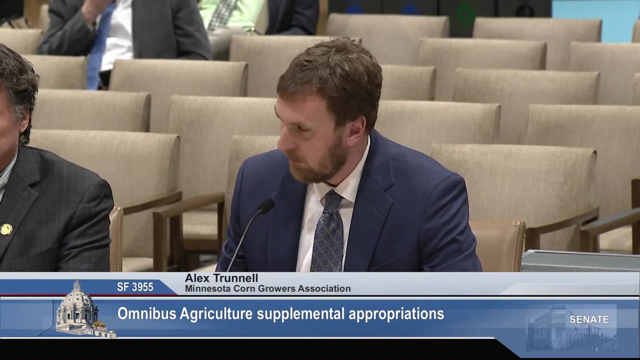 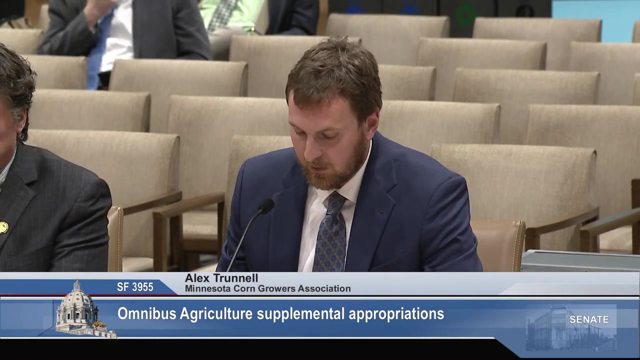 our support for the extension of AFREC to allow farmers farmer funded research that gives Minnesota farmers up to date, scientifically reviewed information to help optimize nutrient use, And this research is also a valuable tool as we look to address nitrates in the state. Once again, we want to thank Chair Putnam for bringing this amendment forward And, given the target and the parameters that the committee was working under, the amendment goes a long way toward addressing the APA petition and help the agencies implement the work plan that they've developed. Thank you, 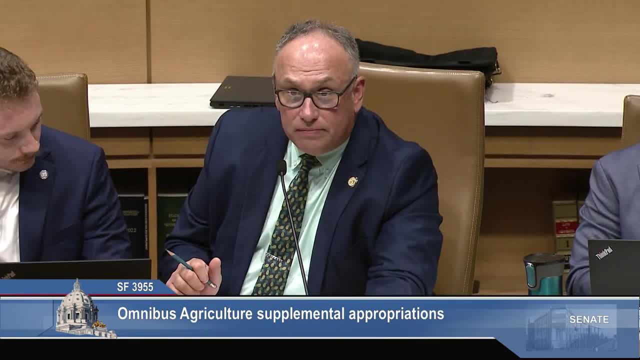 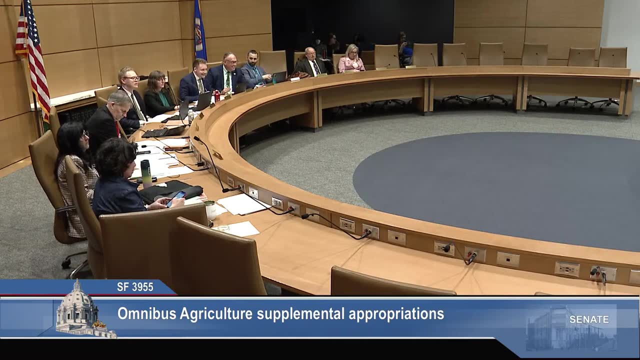 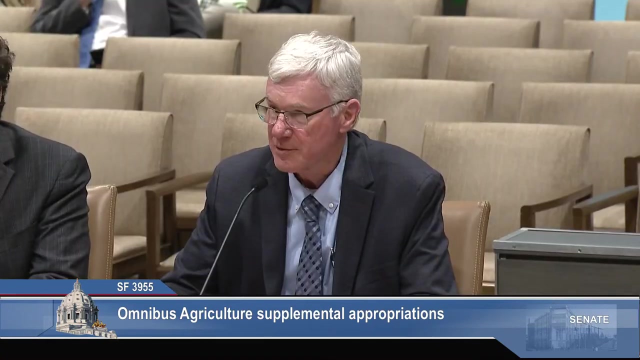 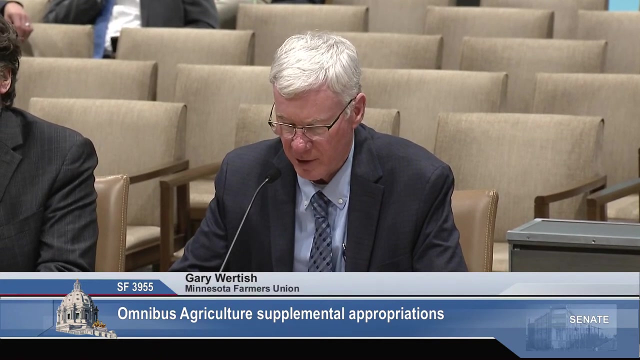 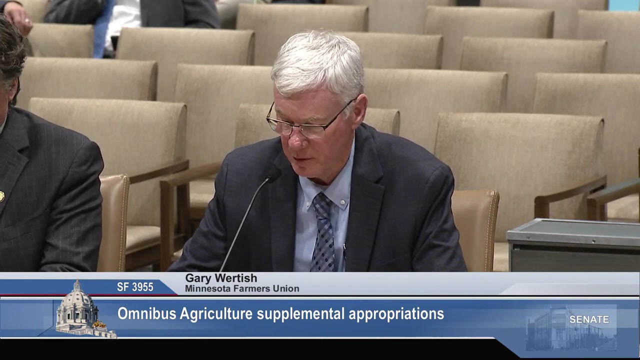 Thank you, Mr Turnell. Next up, Gary Wardish. Thank you, Mr Gorrie. Thank you, Thank you, And you can say your name and fire away. All right, Thank you, Chair Kupec and members of the committee. For the record, my name is Gary Wardish and I'm president of the Minnesota Farmers Union On behalf of our grassroots membership across the state. I'm glad to share our strong support for your for Senator Putnam, in the committees for your supplemental budget proposal and to thank you and your team for your hard work and crafting it. 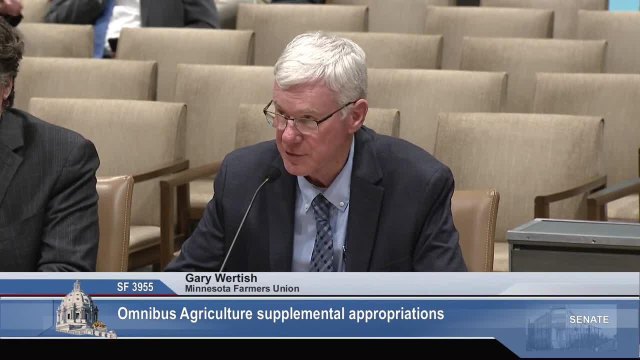 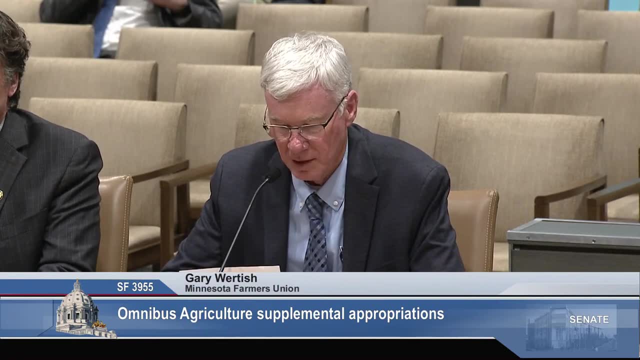 Thank you, One of the Chairman's strength. Thank you, Thank you, Thank you. The strength of this committee is that you listen directly to farmers and we see that reflected and then in this proposal, In reviewing it, I can't help but think about the listening session chair Putnam attended in Zambroda before a session. 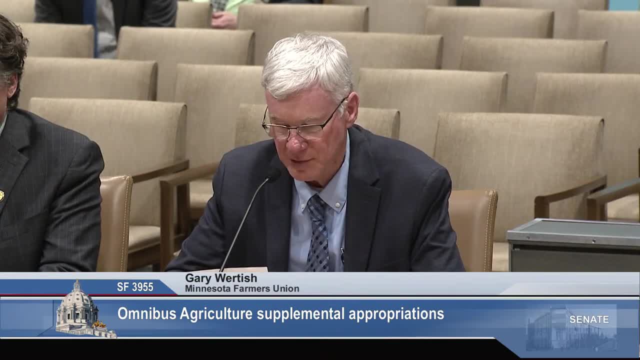 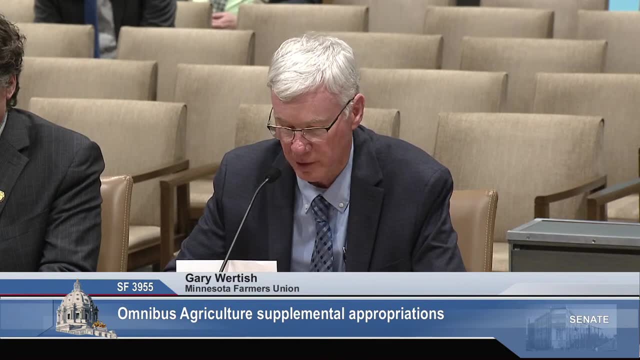 there were well over 100 farmers there of all different sizes and production types, and For probably two hours He took comments and feedback and what they had hoped would inform your work, And now, at a limited budget target, you've addressed many of the issues farmers raised that day. 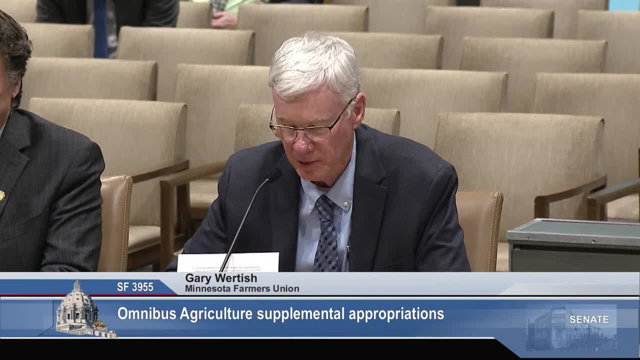 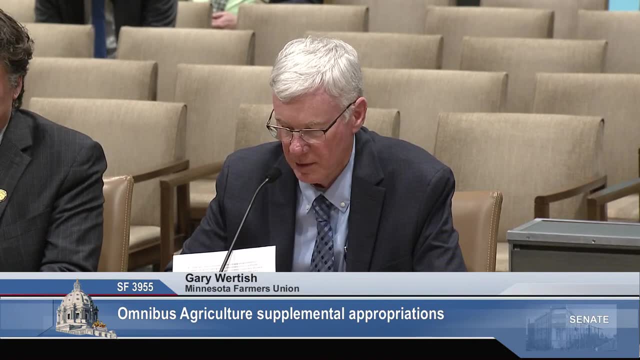 I'll talk about a couple that are particularly important to farmers union and we have a longer letter that it's included in your packet. First, thank you for addressing a shortfall in agri. That program is a cornerstone of our Department of Agriculture and a big reason other states look to us as a leader. 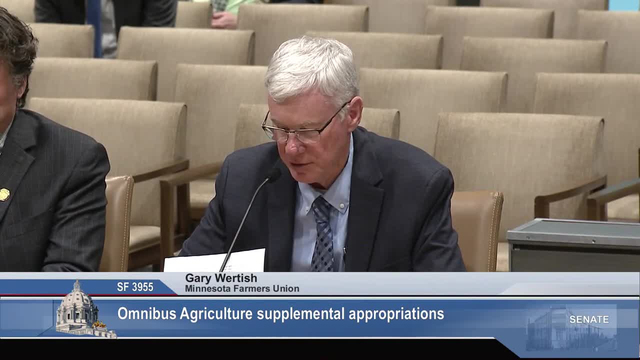 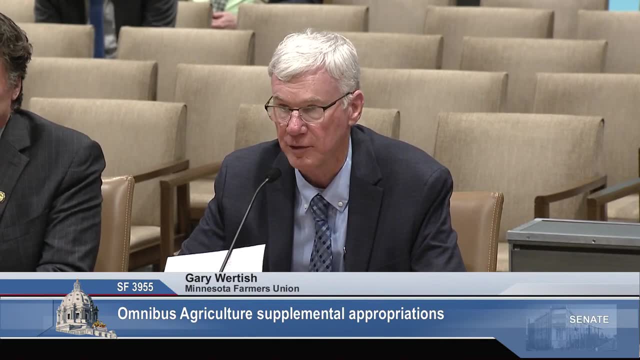 Importantly, those under undesignated funds that you replenish in this bill. allow MDA to respond quickly to challenges Like when the meat, like when the large packing plants shut down during kovat Second we have. we support your approach to a list to addressing nitrates in southeast. 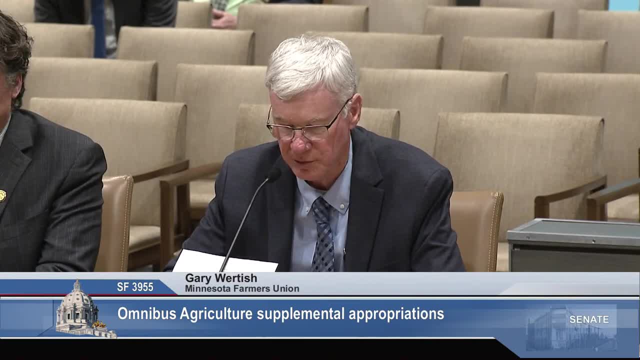 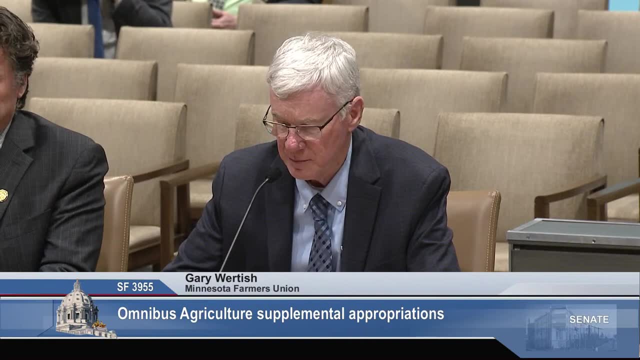 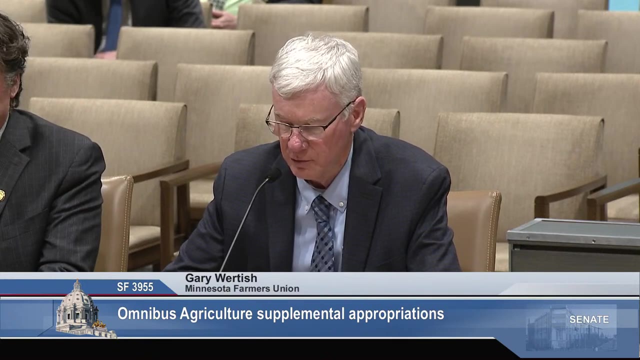 Minnesota and share this committee's interest in ensuring that every Minnesotan has access to safe drinking water. Investing in in the reverse of most of systems and upgrading substandard wells, Along with helping farmers make investments in soil health equipment, reflect the two prongs of the state's response to this issue, and 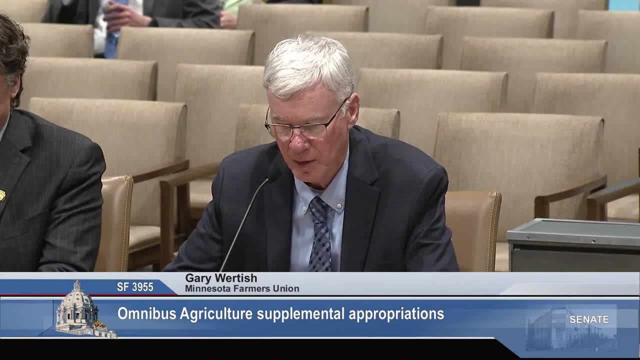 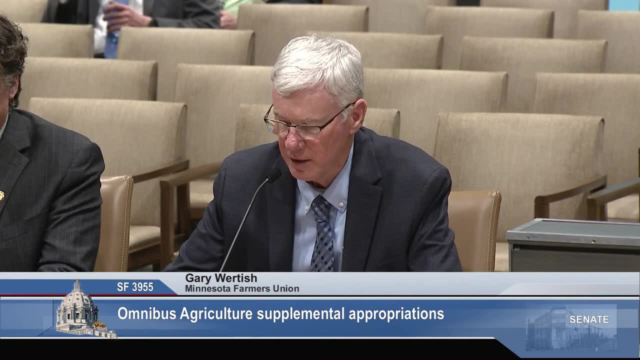 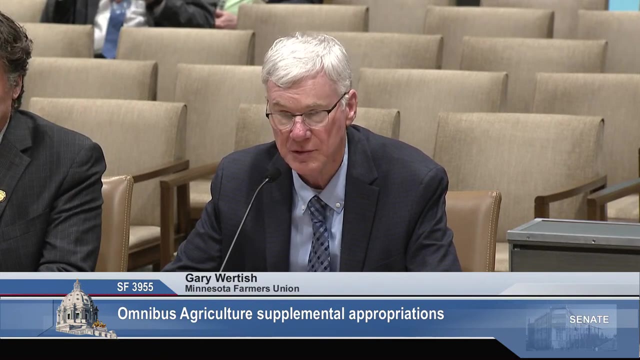 We'll supplement funds made available through the clean water fund. We look forward to continuing to partner with you on this. Third, and because it's something that I've been spending a lot of time in farmers union has Personally, is thank you for reinvesting in grants that help Kate to throw out schools teach meat cutting. 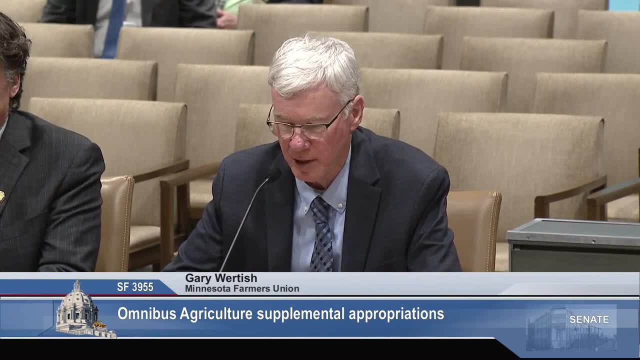 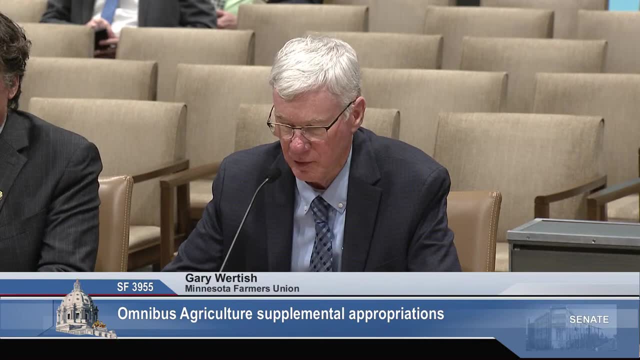 Minnesota farmers union just celebrated the delivery of to meat processing modules to the Central Lakes College to help them continue to build their college program. this enough initiative will help the Train the next generation of meat cutters, creating a pipeline to these programs and ensuring the future of an industry our members rely on. 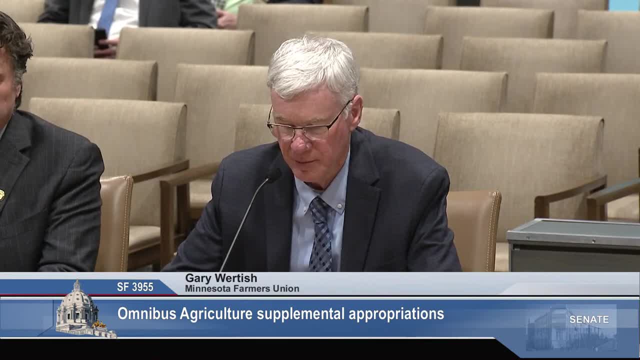 There is of course lots more to discuss, which is outlined in our letter, And I want to thank you to this committee, chair Putnam into this committee, for your partnership at MFU and others in crafting it. But all in all this is a good bill and I'm glad the farmers unit led there lend our support of this bill. Thank you, 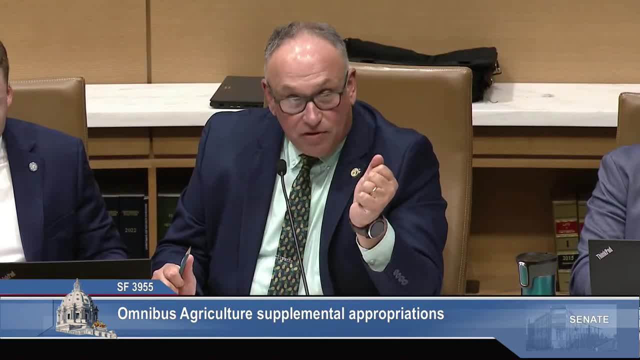 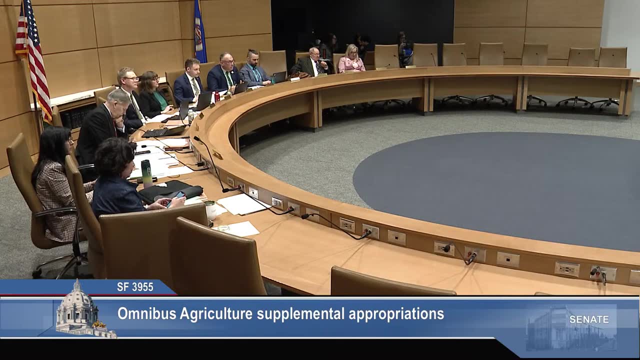 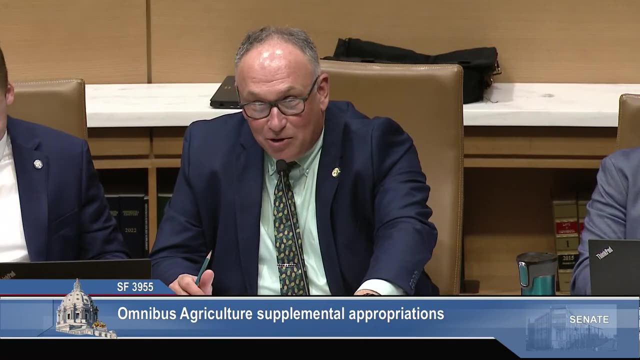 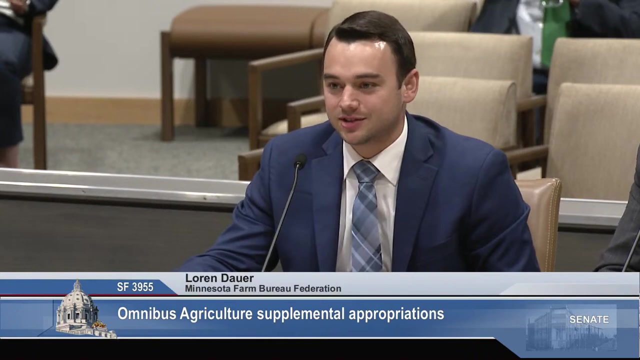 Thank You, Mr Wardish. next up is Lauren Dower from the Minnesota Farm Bureau. Thank you, Chair. You know the drill. I'll go ahead. You can say your name and go away. You know, then you know the drill absolutely. chair COUPAC and members of the committee. My name is Lauren Dower. I'm the public policy specialist for the Minnesota Farm Bureau Federation. 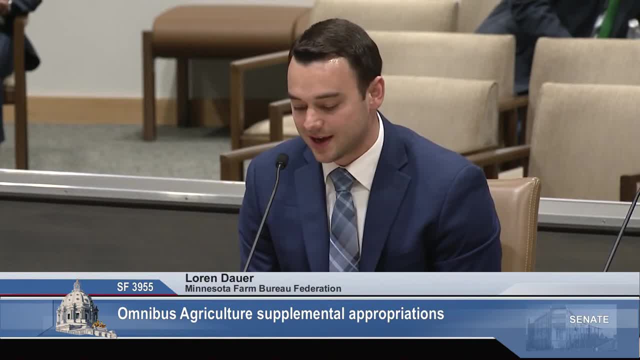 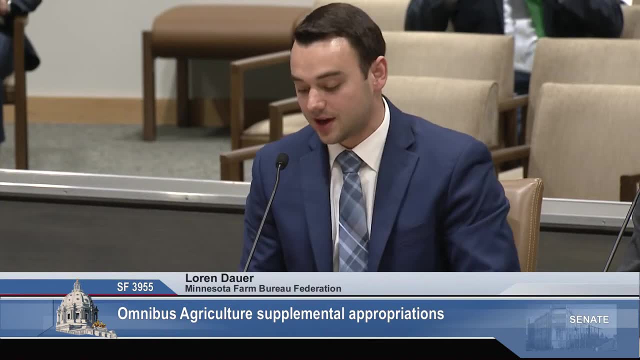 And half of the privilege of representing over 30,000 farmer and rancher members across the state. appreciate the opportunity to testify in support of Senate file 3955 with the DE amendment. I wanted to take this time to thank the author and each of you or. 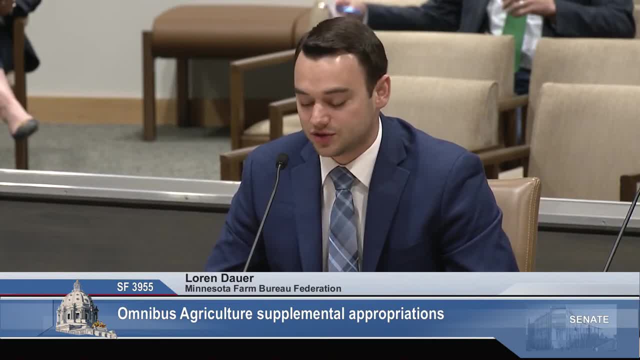 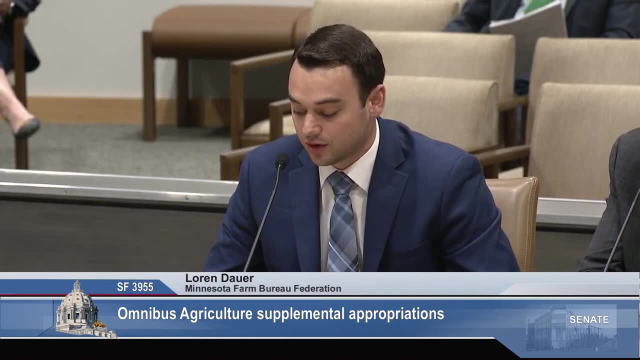 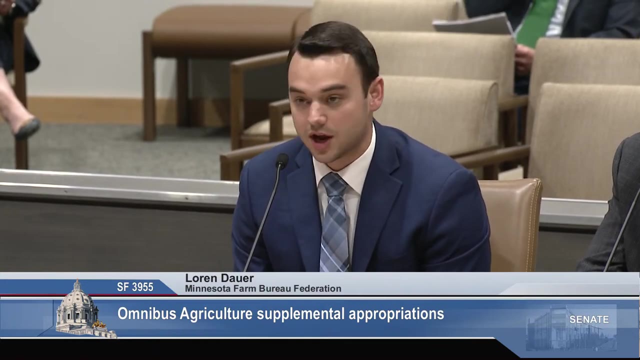 committee members here for your hard work and continued support for our farmers as well as the larger agricultural community. there are several provisions in this bill we support and I would like to briefly highlight a few. first, we appreciate the consistent funding allocated to the Department of Agriculture for the AGRI program. we know this program plays a vital role in 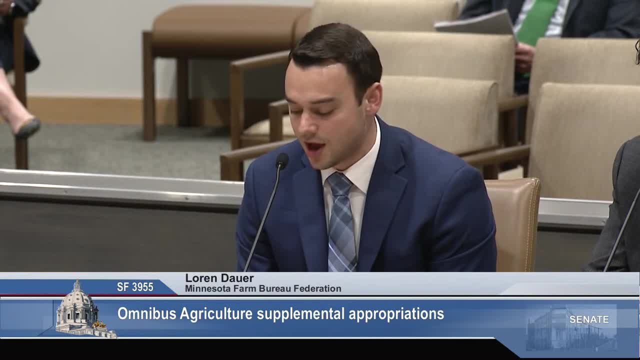 encouraging growth opportunities for the agriculture and renewable fuels industries. thank you for including funds specifically for the animal health protection grants or turkey lasers farm school programs, as well as meat cutting and processing education grants, and for understanding the importance of having our younger generation understand where their food comes from. we definitely. 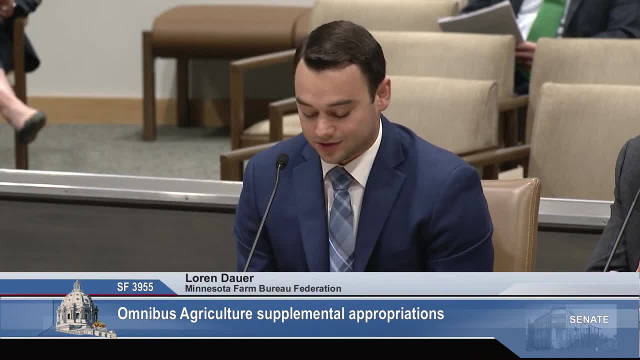 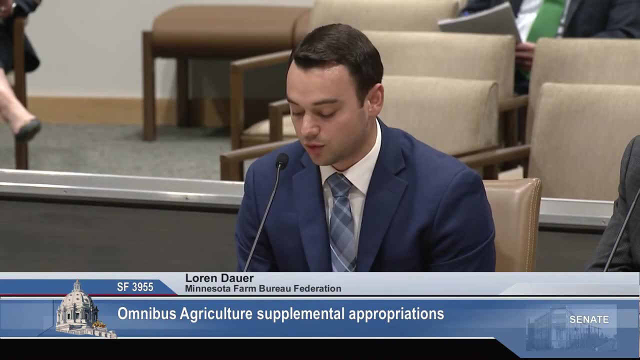 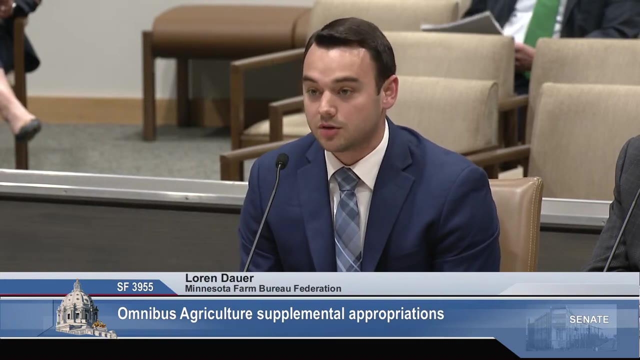 appreciate that we're so. we so support the effect. excuse me. we support the efforts of the dairy profitability and enhancement program and believe the new language in this bill will provide better and flexible access to dairy farmers who are transitioning or adding value to their products. we commend the committee's efforts towards soil health. 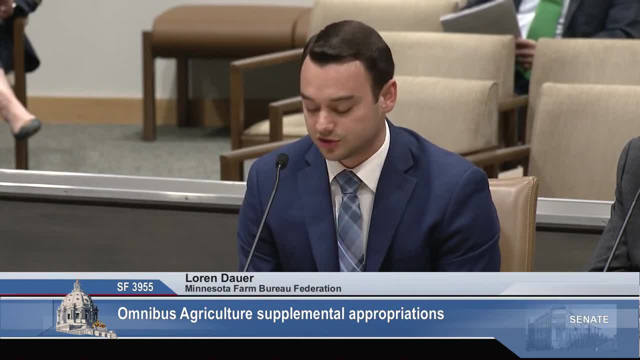 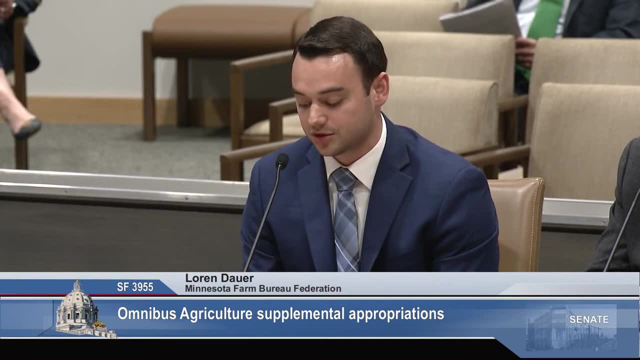 and water quality. as we look towards increasing participation in soil health, we thank you for investing more into the soil health financial assistance grant, which allows farmers access to technology and equipment that helps them use practices that make sense on their farms. we are also grateful for the reauthorization of AFRAC and its 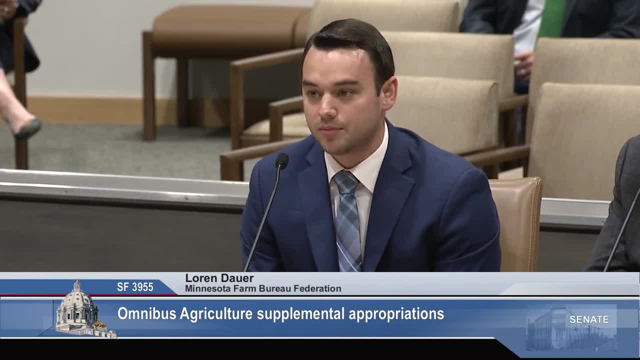 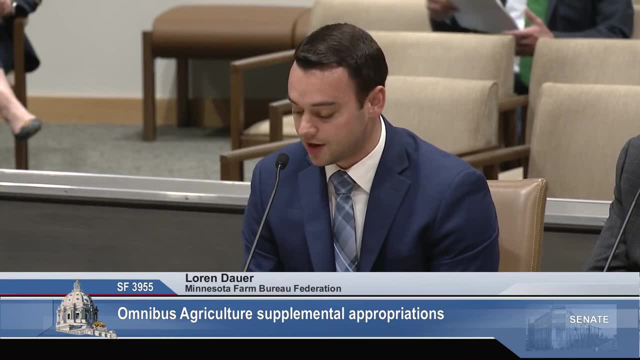 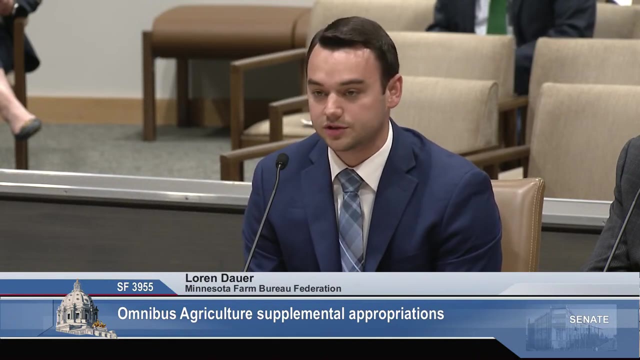 commitment to better understanding how fertilizers utilize and what best management practices assist us in reducing nitrate runoff into our groundwater. the council is a clear sign of strong collaboration in the agriculture community and it's and it is critical to our members who wish to improve their soils, clean water and have economic vitality in their 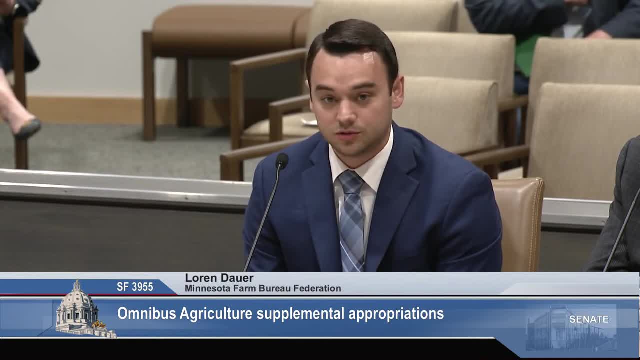 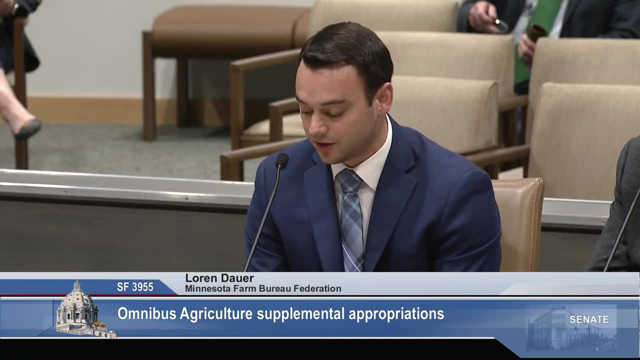 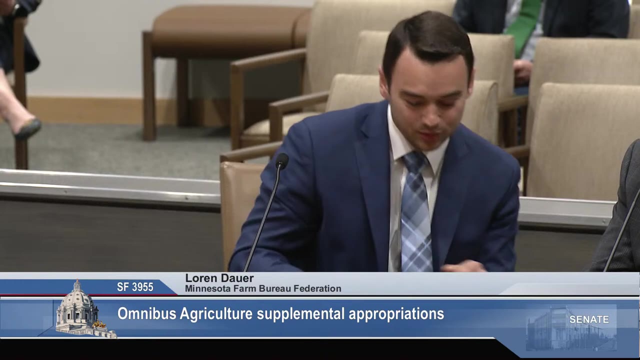 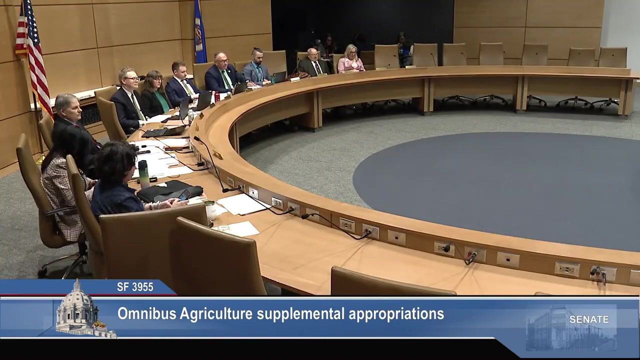 future, and we thank you for your support and we look forward to seeing you next time. thank you, Mr Dower, and with that we have one more testifier to come up, which is Commissioner Tom Peterson, thank you. thank you, Mr Chairman and members. 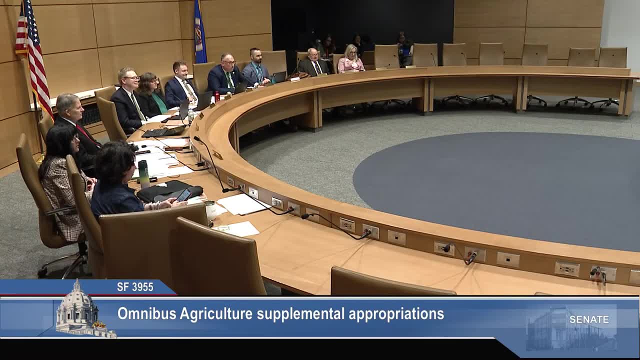 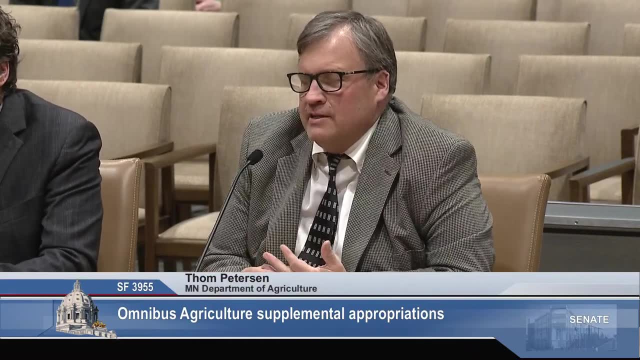 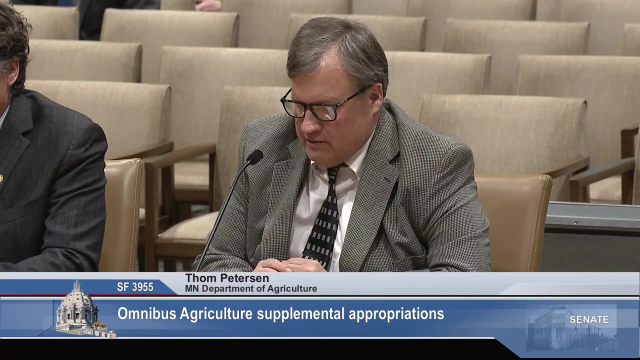 thank you, Mr Chairman and members. I' m Tom Peterson, commissioner for the Minnesota Department of Agriculture, and just appreciate the opportunity to comment on this and again, it's really an interesting and unique to be here with targets and a set amount of dollars to work for, but with the limited dollars in budget the department was really pleased. 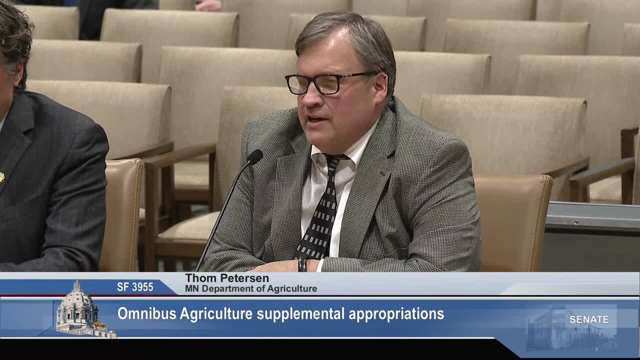 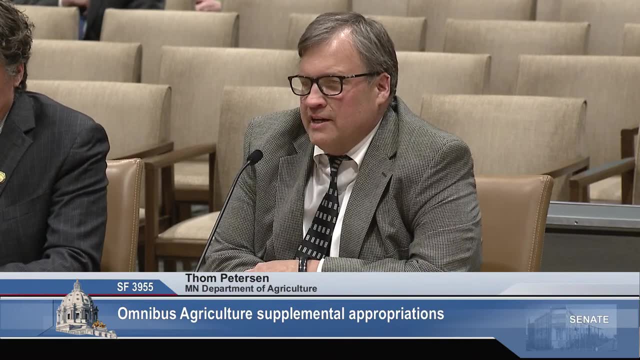 to see dollars put towards the nitrate initiative and then what the Senate did with the bill, or chair putnam, uh, you know, working with us with the ro systems, and again, i think that we can really build on our pilot kind of see what the need is and then when we come back next year, we 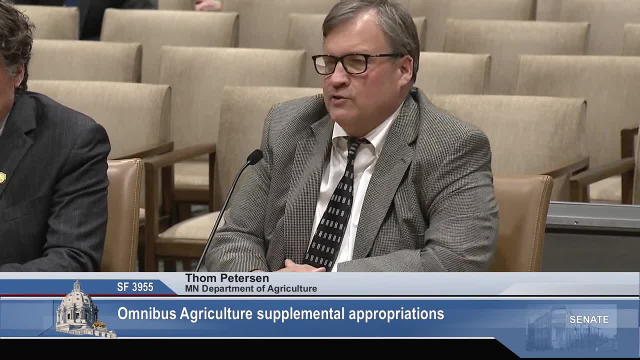 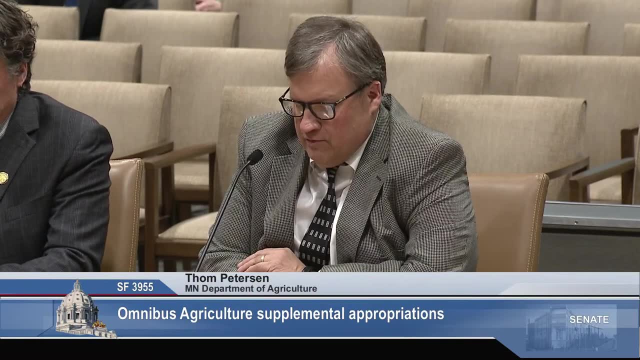 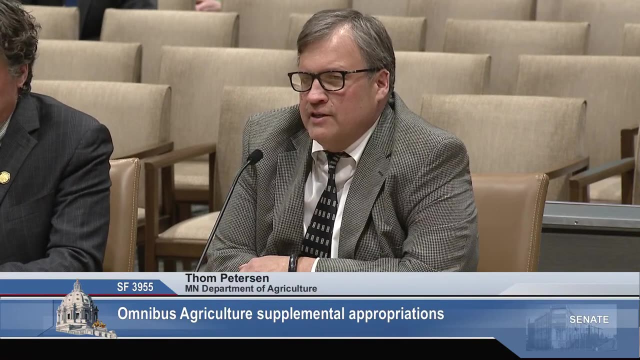 can continue to build upon that and look at that. but it also helps us work, as mr ternell said, getting to our uh addressing our epa work plan, uh in moving that out, but also uh the soil health equipment grants. i think that's been a wildly successful program. but then taking it uh for this, 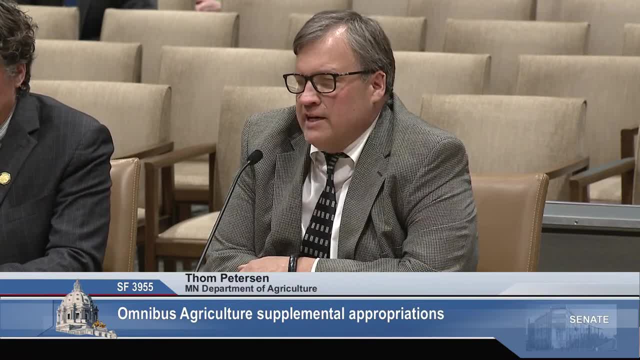 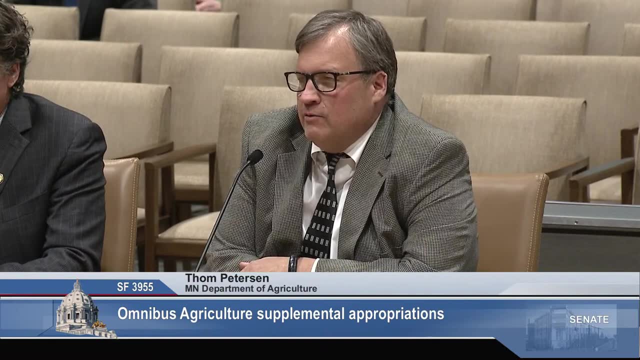 uh amount of dollars and targeting it into those eight counties, i think will be really impactful, but it also will help us statewide. things that we're learning uh, building upon there, what's working, are things that we can take out uh and move uh again across the state. 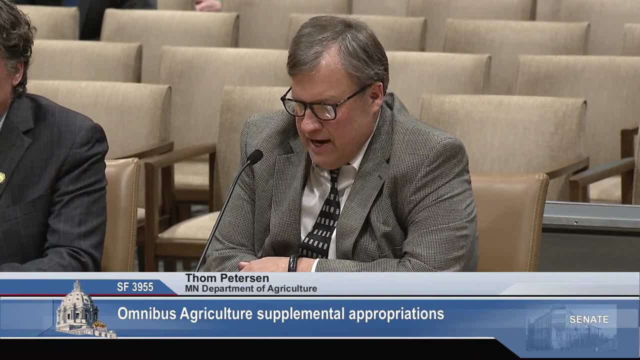 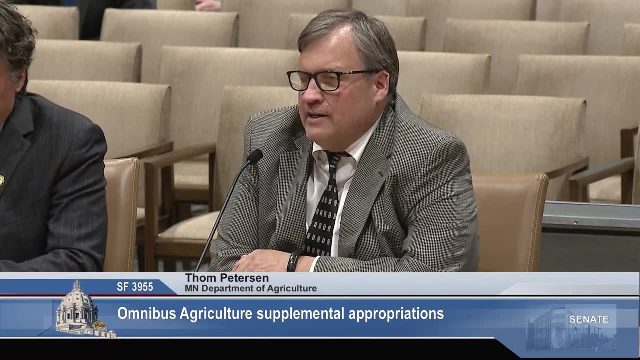 i'd also like to say the uh, the agri is also a really important piece that we've heard about and we worked really hard last year and so, uh, you know and took a um, you know, took a hit in there. you know we've been doing a lot of work on this and we're also doing a lot of work on the. 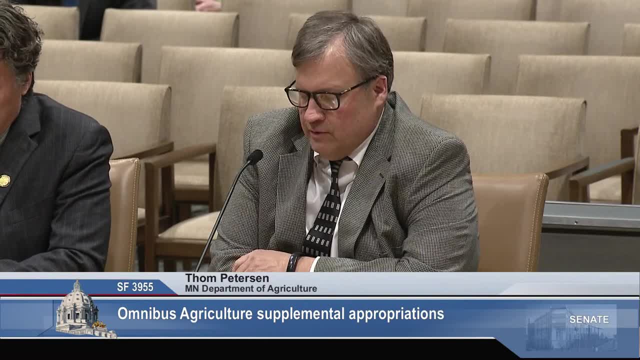 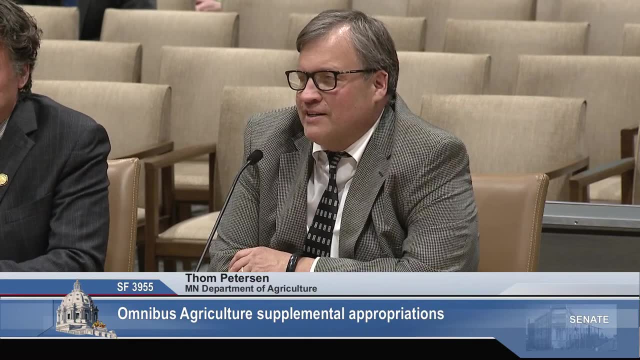 on the agri department as well and we're also working on the agri department as well and um located And so any dollars that we can put back into there and I really like what the Senate did working on. you know we joke a lot about turkey lasers but it is really important work. you know having a foreign animal disease such as HyPath, and now we can see what it's done with dairy cattle and goats. 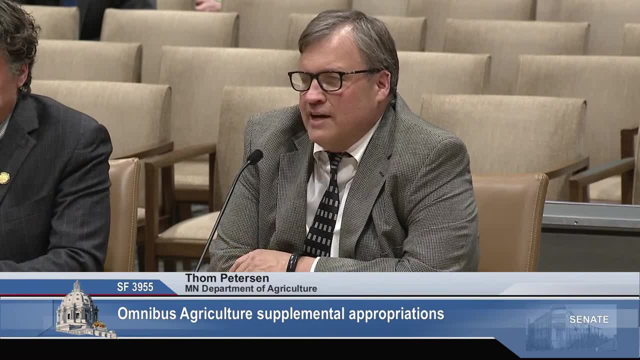 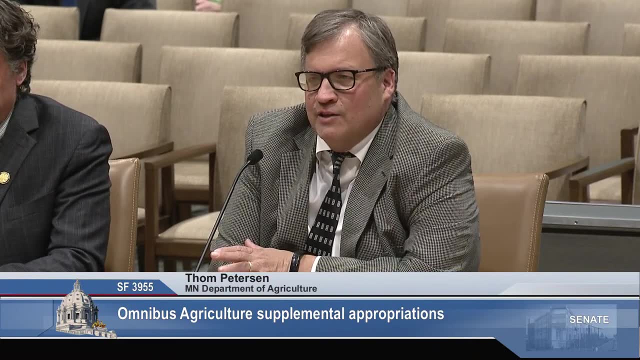 And you know, but the Secretary Vilsack was here last week and you know I was proud to be able to say that we've taken steps to mitigate, you know, and we're one of the only states then that has done something on the front end. 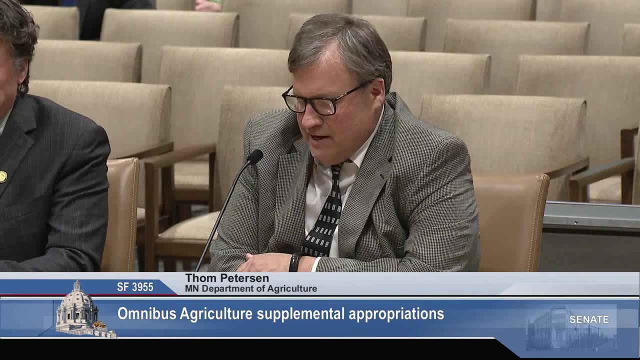 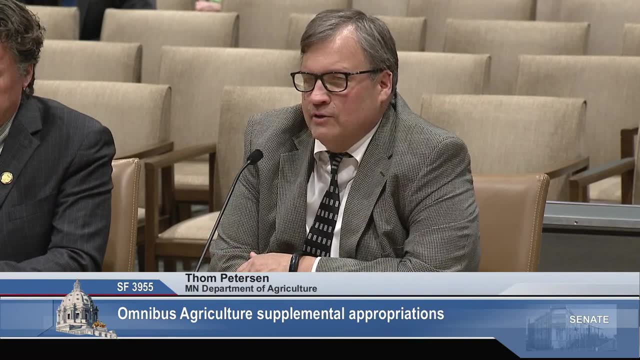 And so this helps us build that out and continues that and also gives us also there's some dollars there for some extra flexibility in agri. I think we would look at dairy and livestock or different things that we would work to use those extra dollars. 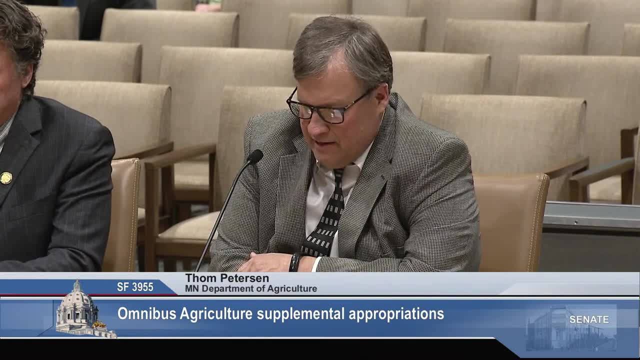 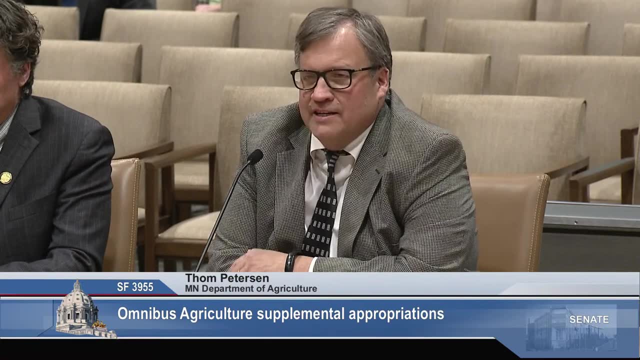 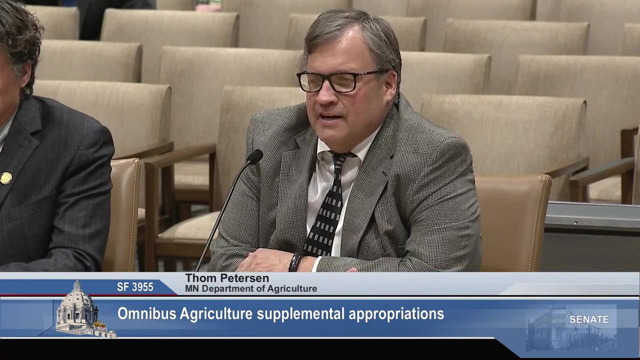 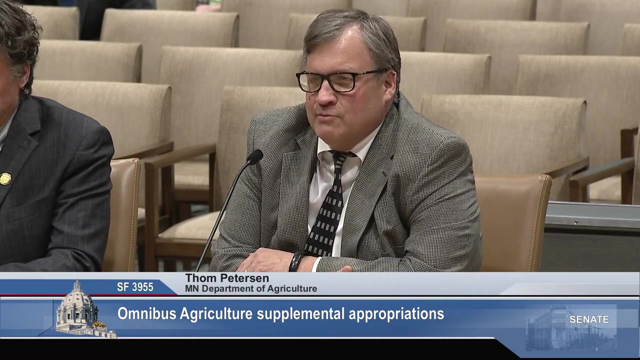 And flexibility in there. Also, the meat cutting piece for secondary schools that Senator Dornick worked on. that's a really impactful piece When you look back at what Mr Werdish was just saying about the secondary schools. I think that during our time here we'll look at what we did for the meat industry in Minnesota on the small end. 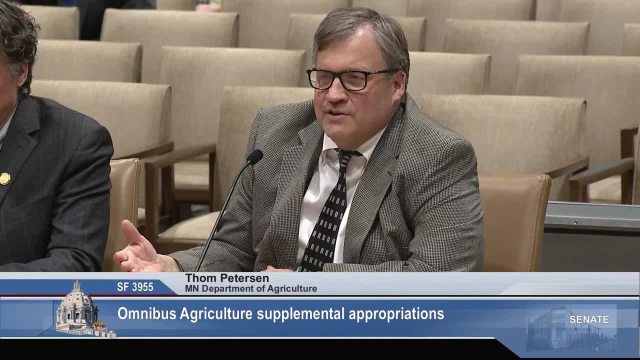 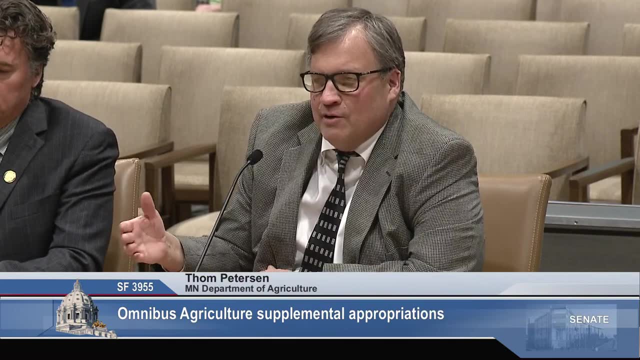 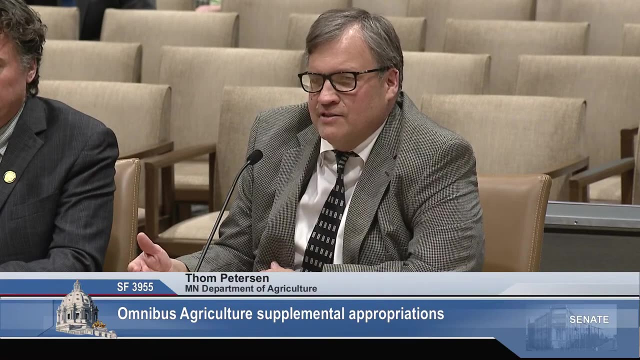 We have a lot of grants and everything, but we looked at we also needed butchers, you know, And so. So Minnesota really stands out across the nation because not only did we build where build out our post-secondary- like they're talking about at Central Lakes and at Ridge Ridgewater, with having classes there. 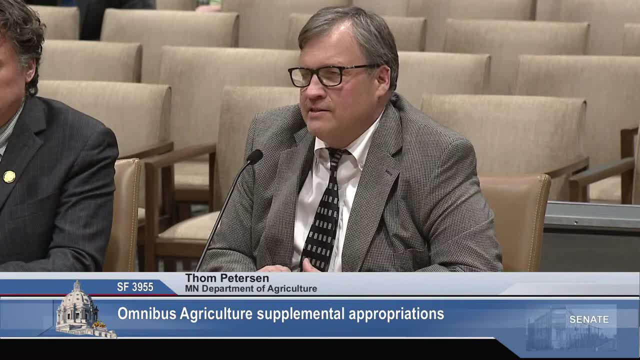 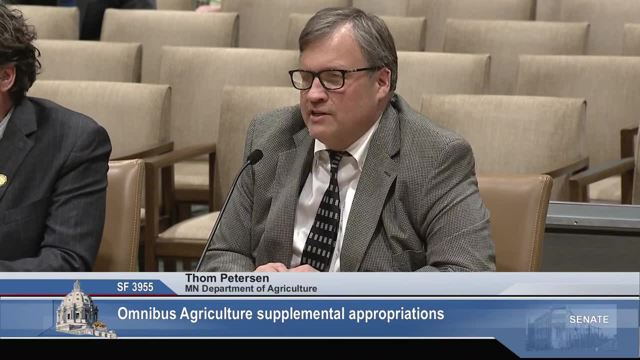 We've also done and started to help support classes in secondary schools and it's really exciting to see- I think it's West Central Area Schools and Senator Westrom's district. I got delivery of their trailer last week. That is really neat if you haven't seen that. 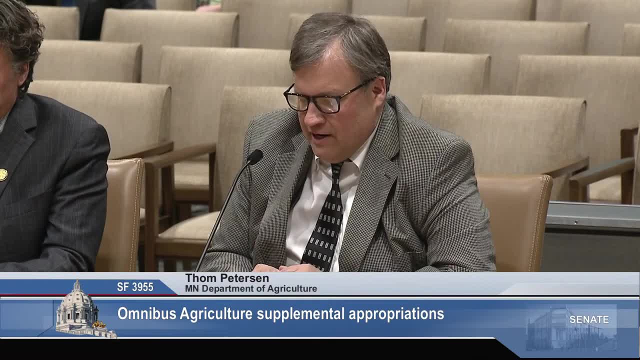 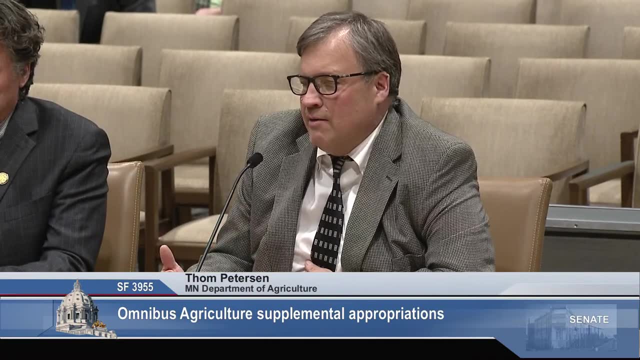 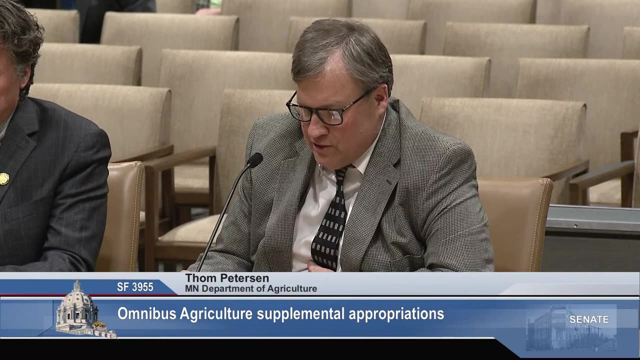 But the other Work that those high schools are doing are very, very good And so that's a real positive piece that again gets to the root of the problem and really helps grow our our industry there that we need to do so much. 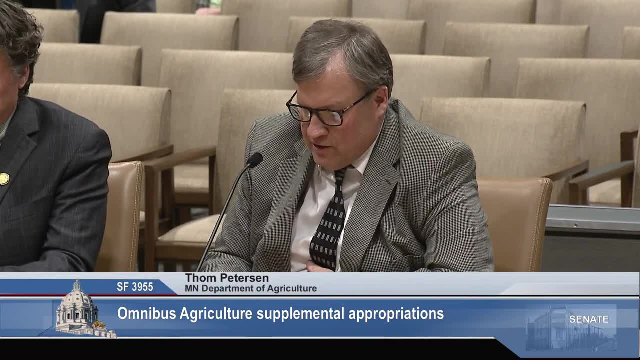 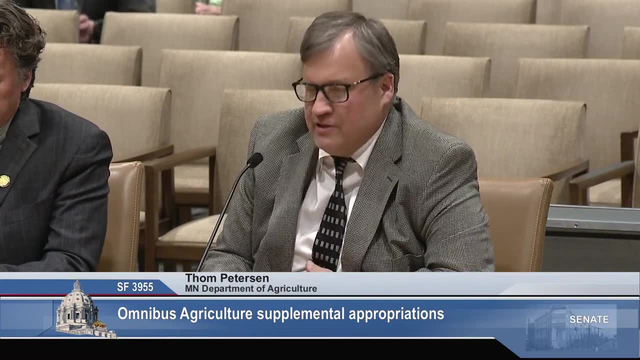 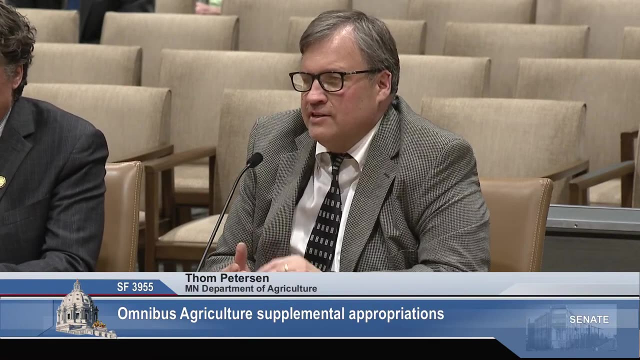 Finally, I'd also just mention AFRAC. a very important piece you know is also is that we've seen- I was here when it passed years and years ago And we talked about it, but to see the work going on in the support it has within the industry, appreciate the continued support for that. 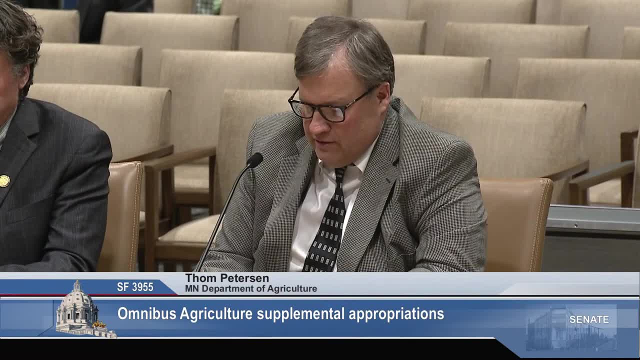 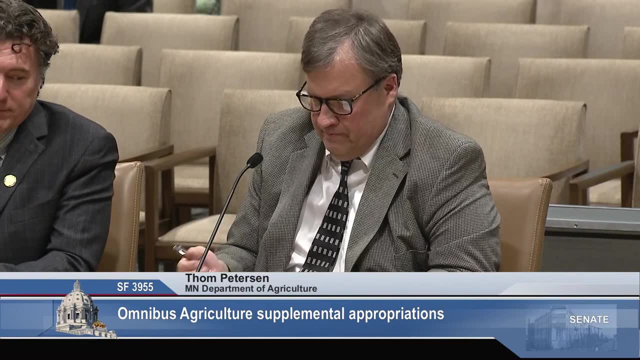 So with that, Mr Chair, I just want to thank the work of Senator Putnam and in in the committee and we look forward to working with you as we go through this process. Thank you And thank you, Commissioner Petersen. 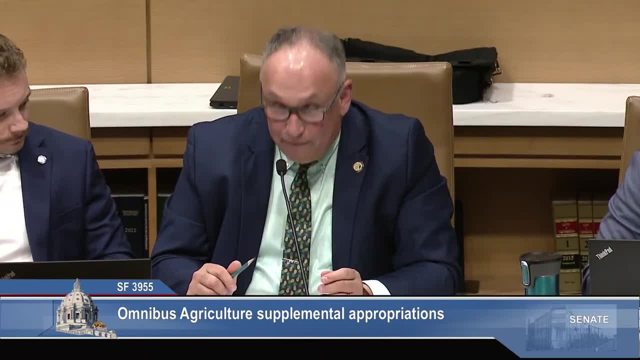 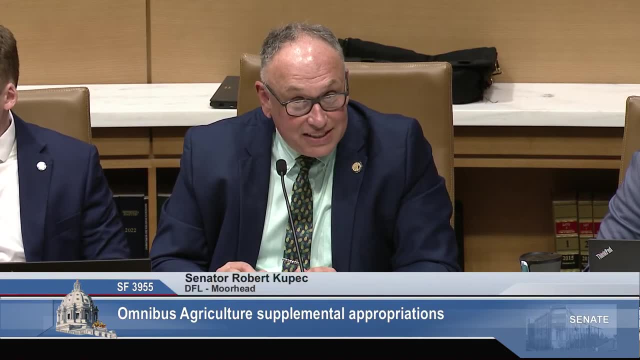 So a reminder: we will do member discussion and amendments for this bill on Wednesday, but if there are any specific questions for one of those, we will be able to answer them, Thank you. Thank you, Mr Chair. If there are any specific questions for one of the testifiers that was here this afternoon, we could do that. 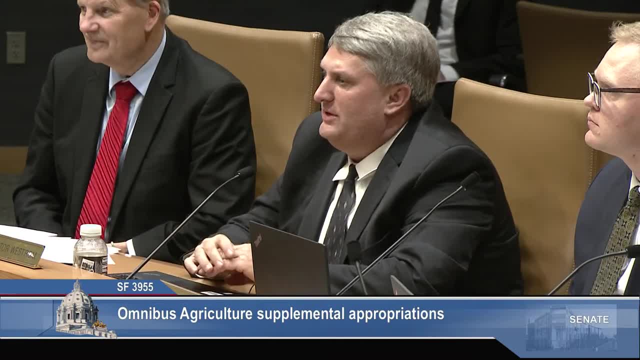 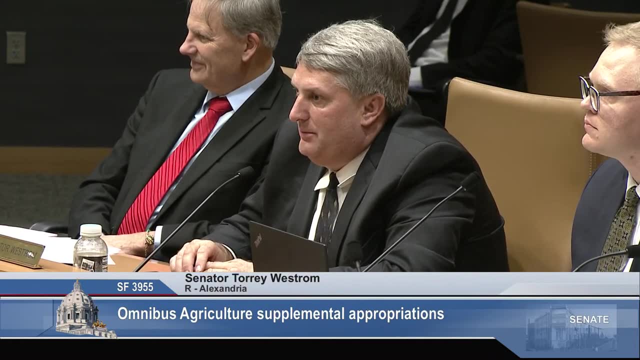 Senator Westrom, Mr Chair, Commissioner Petersen, the dairy with an eye rolling those dollars over. Can you explain that a little bit more? And if you've already explained it before I got back in here, I can talk to you offline. 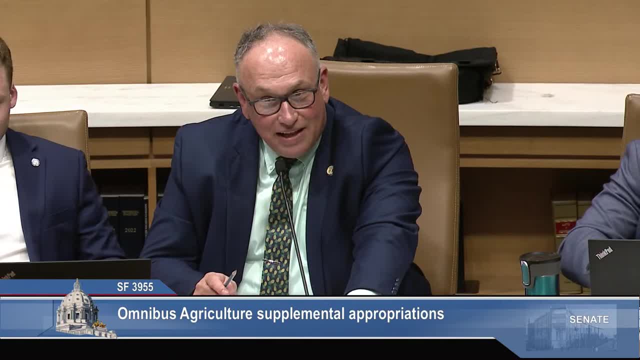 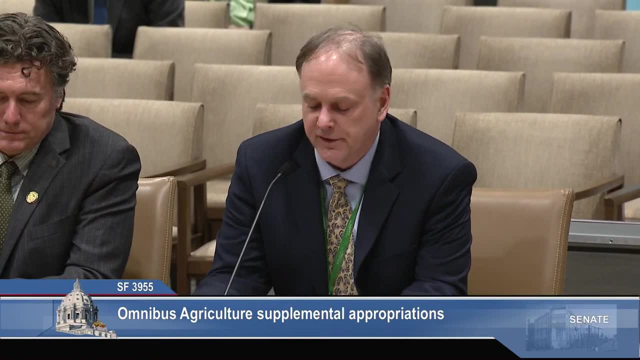 And I believe we are. we are going to have Mr Hugh Going to explain that. Thank you, Mr Chair and members and Senator Westrom. So my name is Paul Hugen and I'm the director of the Ag Marketing Development Division at the Department of Agriculture. 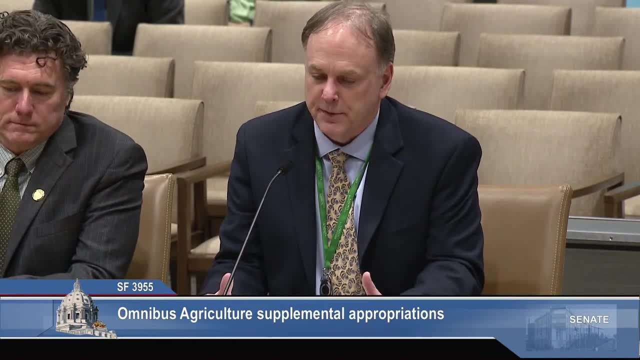 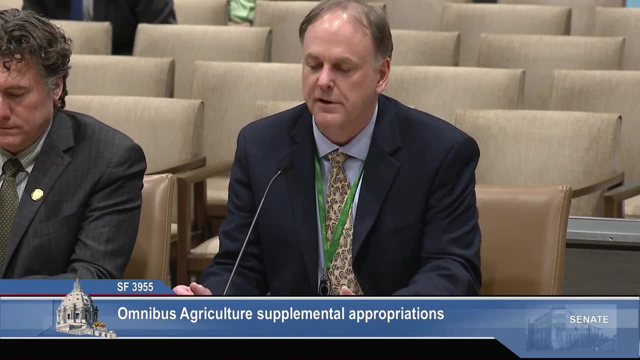 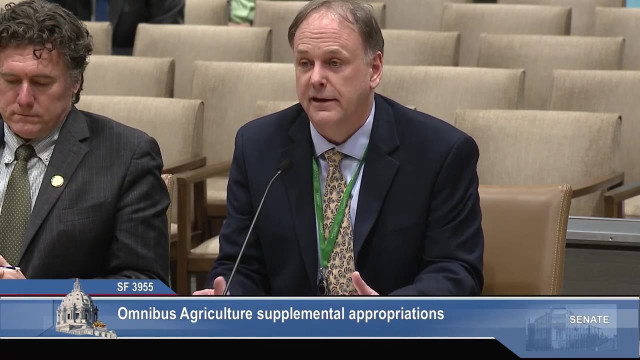 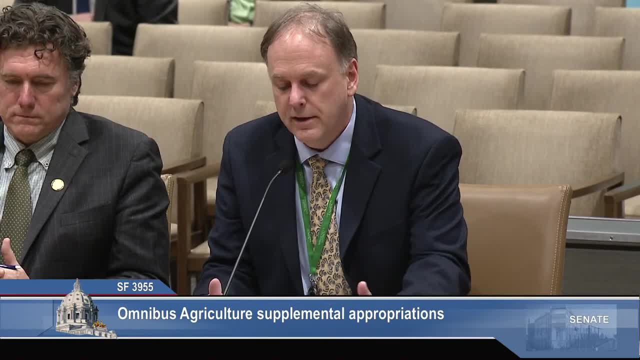 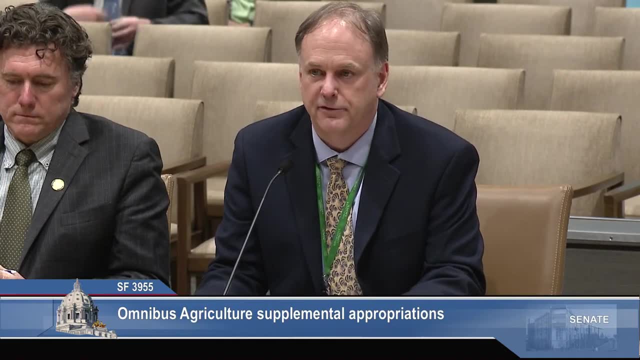 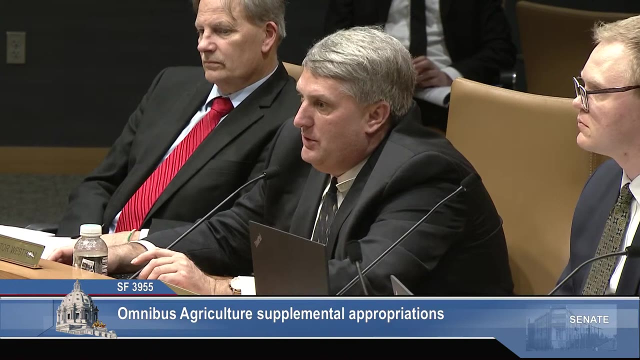 So that we can can incentivize farmers to sign up for more than one year at a time. so that's the reason for for allowing that additional time to have those dollars available. senator Westrom. mr chair, it's the same dollars, it's just there's been. 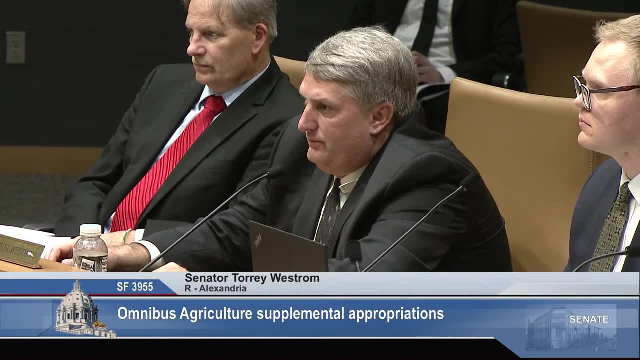 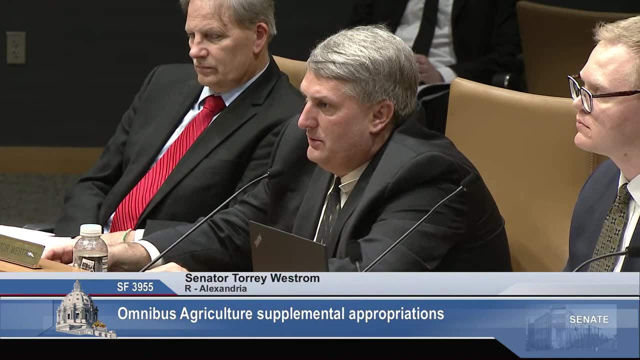 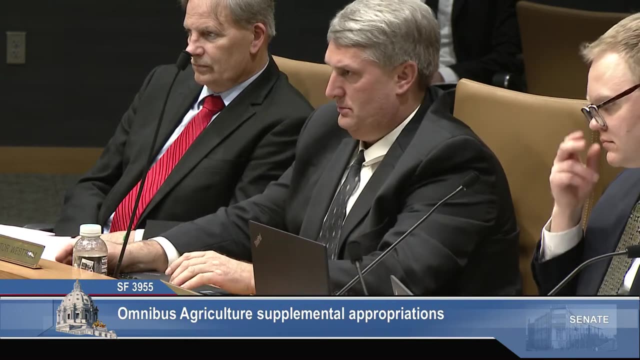 some uncertainty or without a new farm bill, you can't get the five-year plan now. is that the deal, and you're gonna kind of move ahead with the current landscape as much as you can? yeah, mr chair, senator Westrom, so the what, the what's available right now, is simply just a one-year option for dairy farmers. 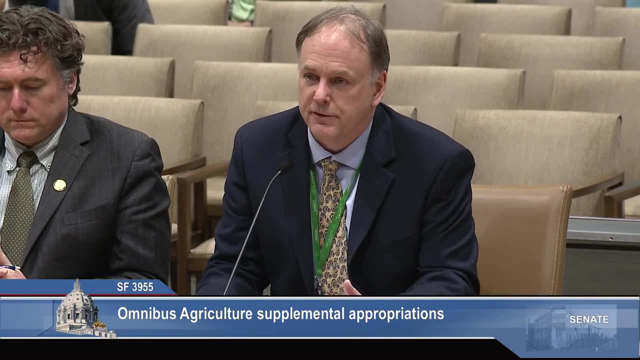 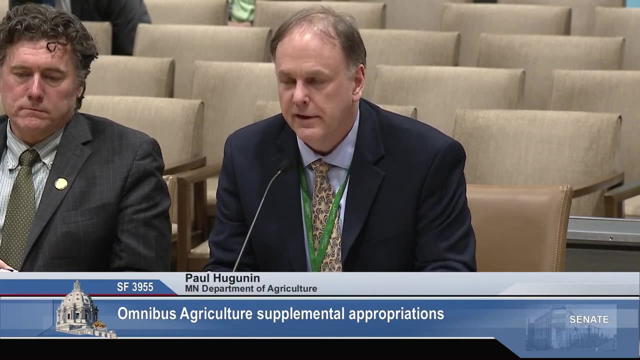 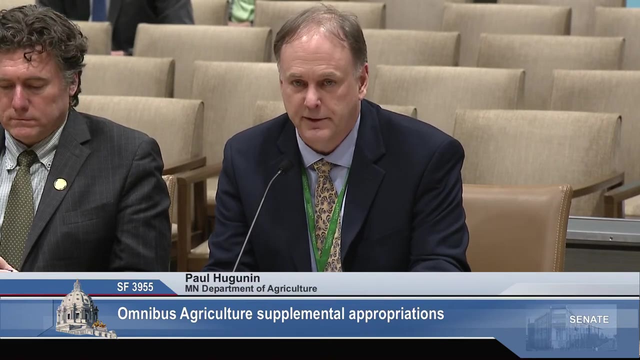 to sign up for dairy margin coverage, and industry folks would prefer that we hold off- be able to use that four million dollars to incentivize longer-term signups. and you're correct, it's the exact same dollar amount. it's just allowing us a longer window to invest that with dairy. 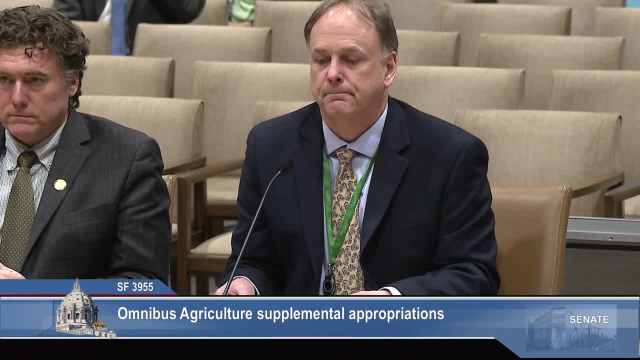 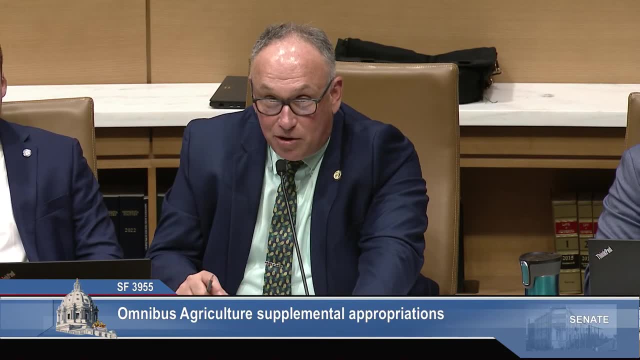 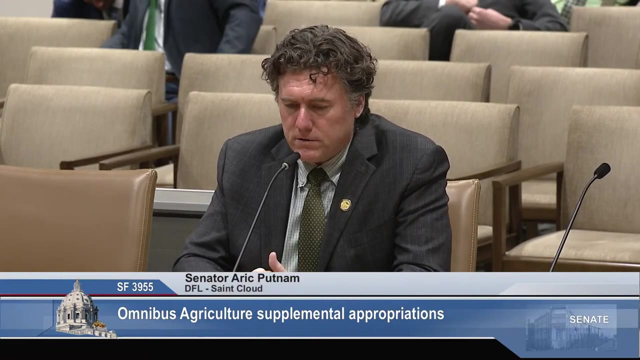 farmers as they sign up. okay, anybody else if not senator Putnam, do you like to make some closing remarks and tell us where we're headed on Wednesday? mr chair, sir Thainley, thanks for the indulgence today. I do want to take an opportunity now, so I don't forget to do it later, to thank everybody who has been. 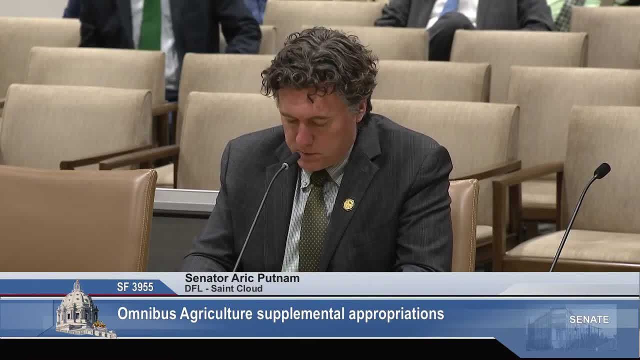 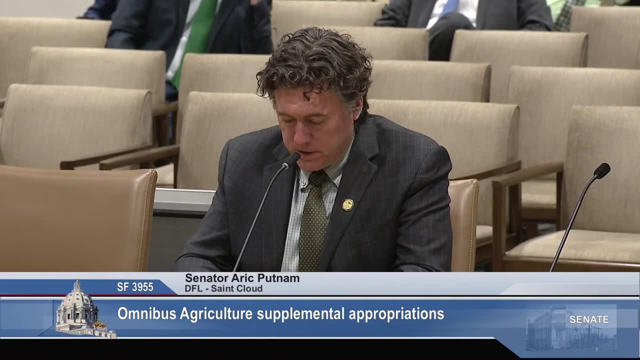 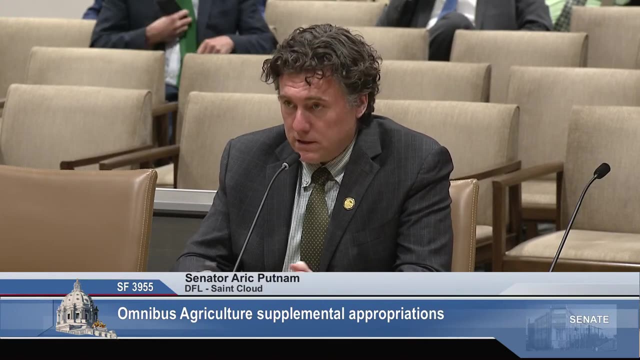 involved in this process, this session. you know I'm gonna thank mr Painter and mr Olafson for always being incredibly skilled but also very kind, and Miss Peterson, mr Larson for your work researching for this committee- thank you for your hard work too- and, of course, hunter and Nick and the 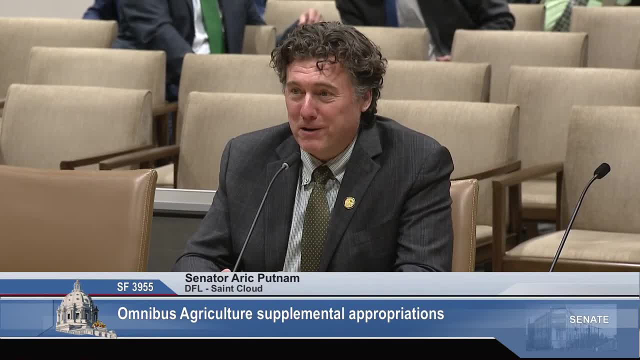 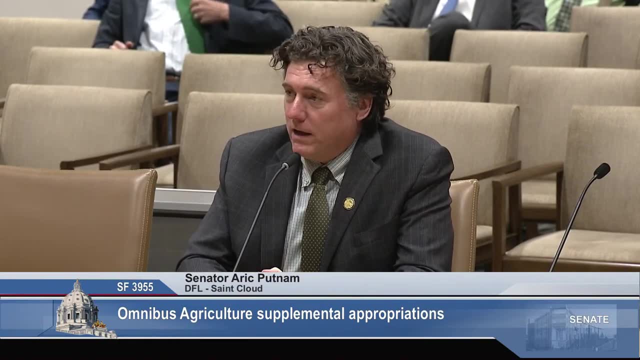